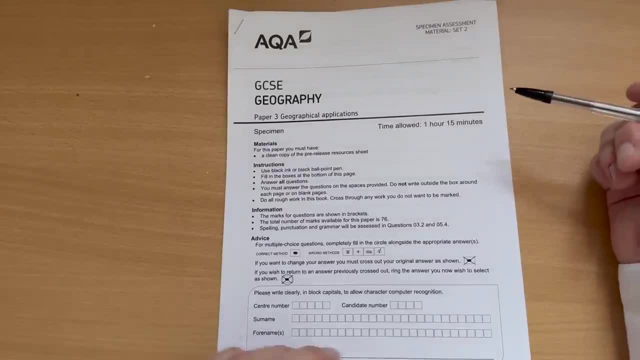 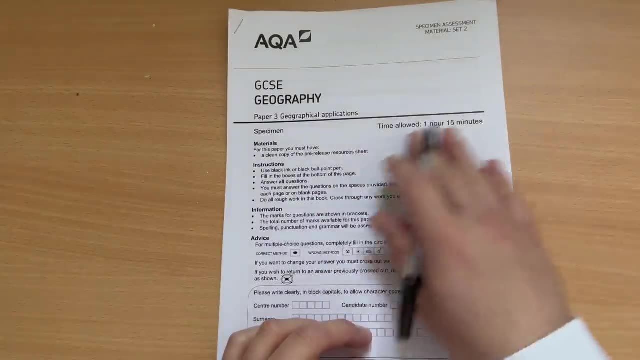 hopefully you'll see some similarities between each paper as we go through. So I'll fill the front end as usual. You know you might want to. I don't think you need to put as much on the front as you would with your other exams, but again, I reckon it's definitely. 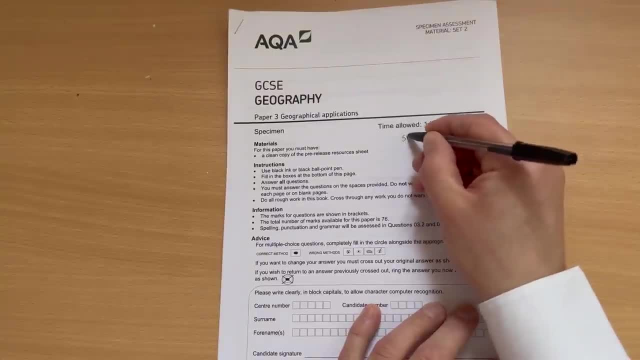 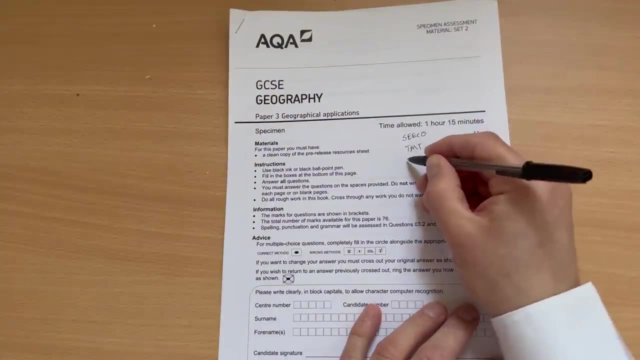 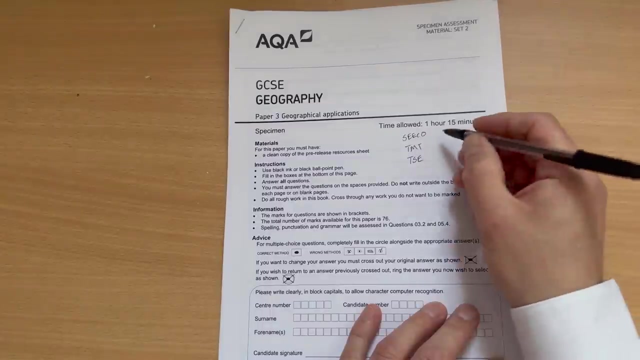 worth putting a compass on the front. SECO Social Economic Challenge Opportunity. If it's going to ask you to explain, this means that If it's going to ask you to make a decision, so evaluate, assess, agree to some extent. There might be a graph question. 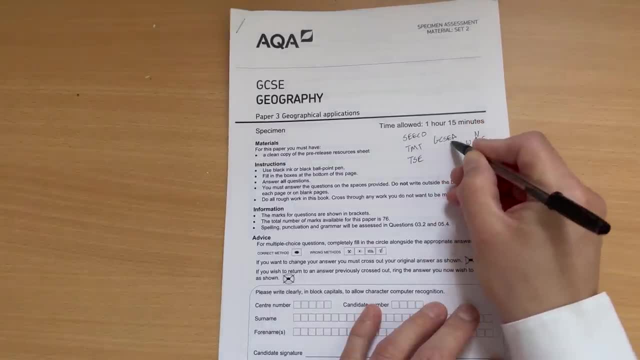 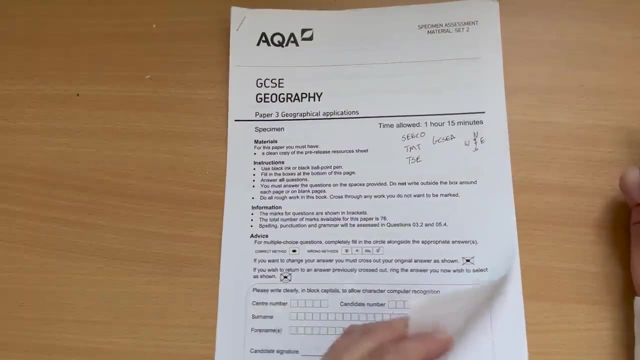 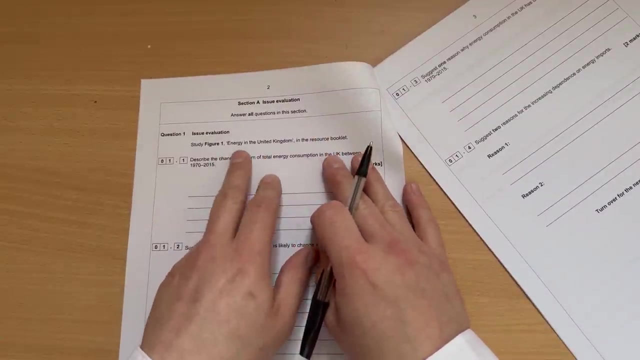 GCSEA General Comments. Specific Example: Anomaly: But yeah, but this is often called the skills paper because there's a lot of skills in it. Now, the first question is going to be about a pre-release. Now, we've not looked at this pre-release. It was about energy. 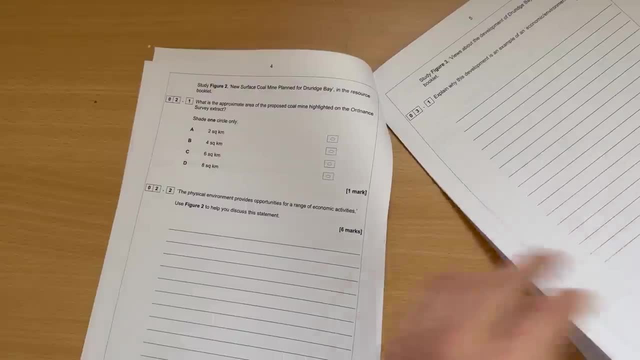 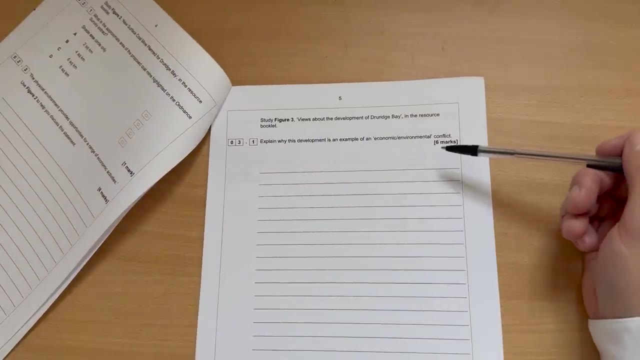 in the United Kingdom. okay, And the first two questions are always going to be about the pre-release. Question three gets a bit bigger. That's going to be a sequence of questions. Question three is going to be the six marker And then finally the second half of question. 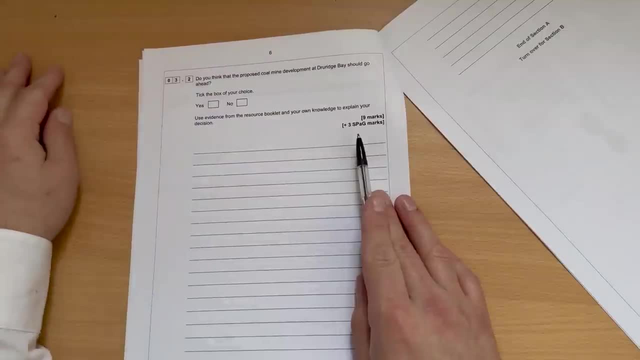 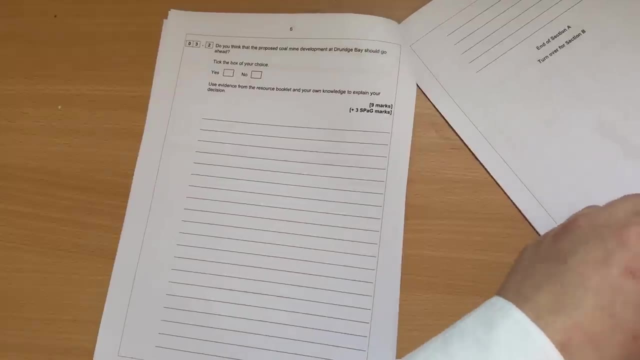 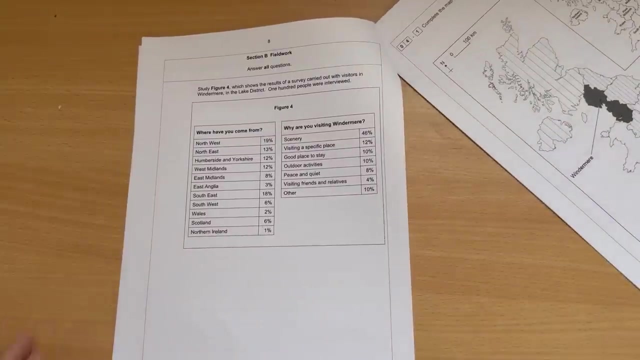 three is going to be the 12 marker, And if you watch our other video for 2023,, you'll probably see a great example of that answer. Please excuse the people shouting in the corridor. They're just having a laugh, aren't they Right? So, section B- fieldwork- This is what 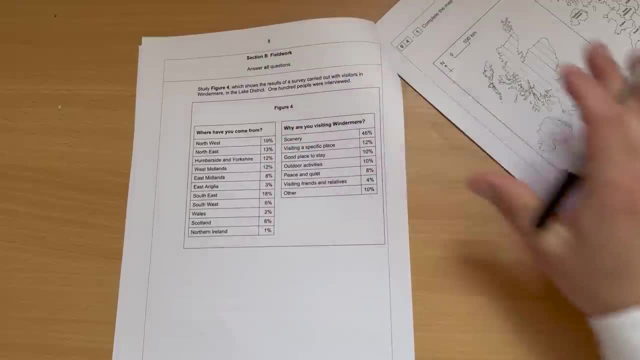 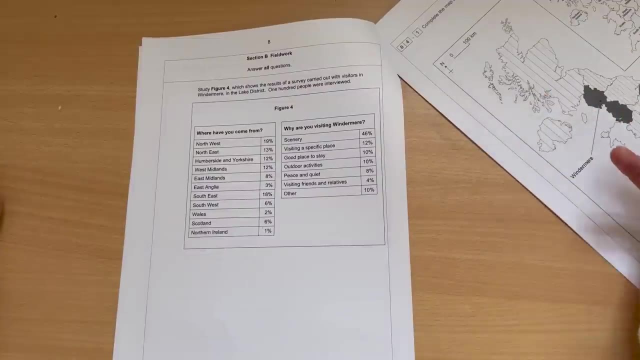 we're going to look at in this video. all right Now. the first one is unfamiliar fieldwork, So this is not fieldwork you've done. It's fieldwork you've done, You could have done, but it's data that other students have done. So let's have a look. 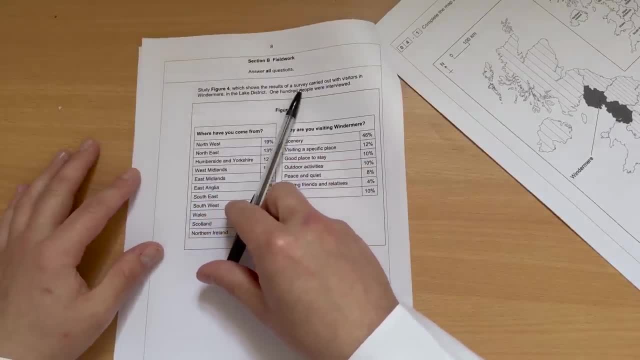 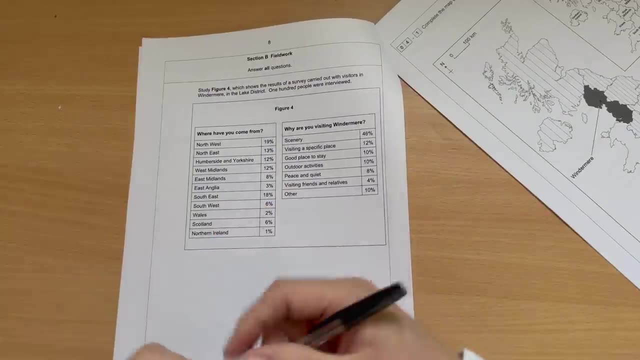 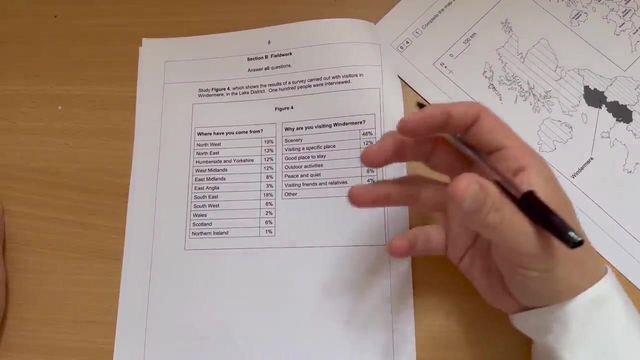 It says study figure four, which shows the results of a survey carried out with visitors in Windermere in the Lake District. 100 people were interviewed Straight away. you've got to think right. if we're interviewing people, all right, these results are going to be based. 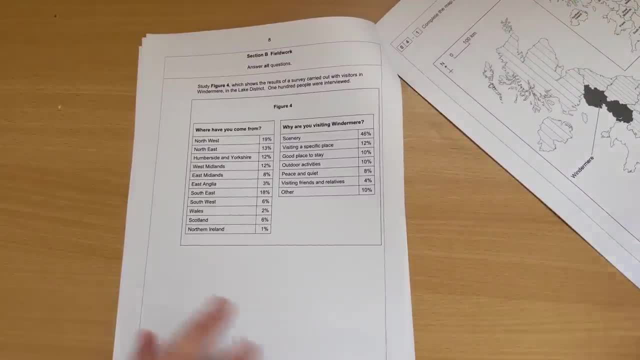 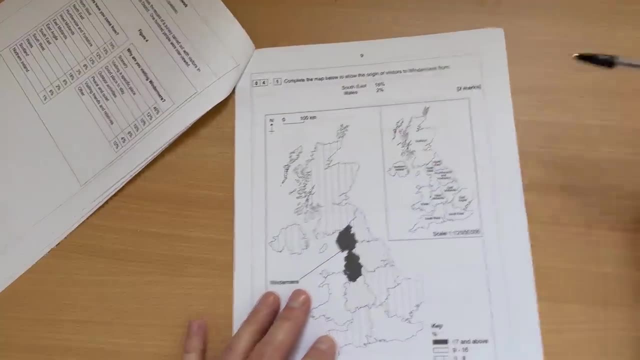 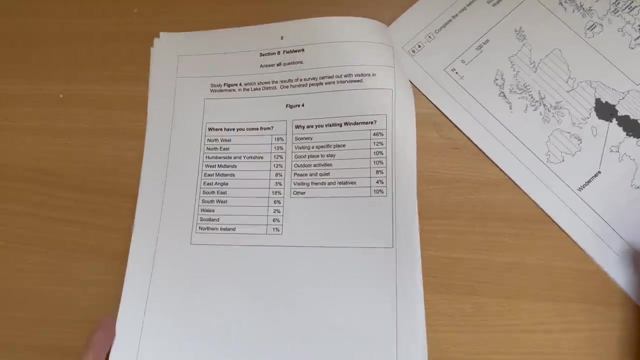 a lot on their opinions. okay, But anyway, what's the first question we want us to do? Complete the map below. We want to show the origin of visitors to Windermere from South East. So the South East is down here. It tells you on the map there. And the South East: we've got 18%. So you 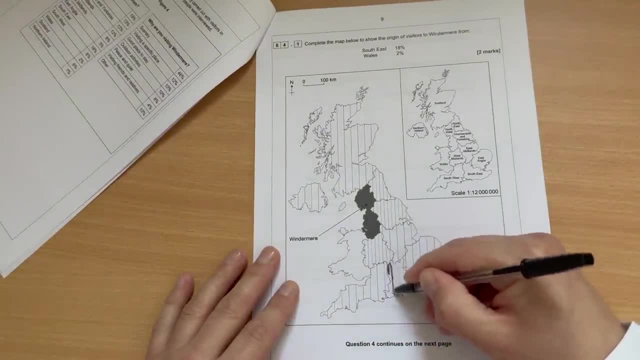 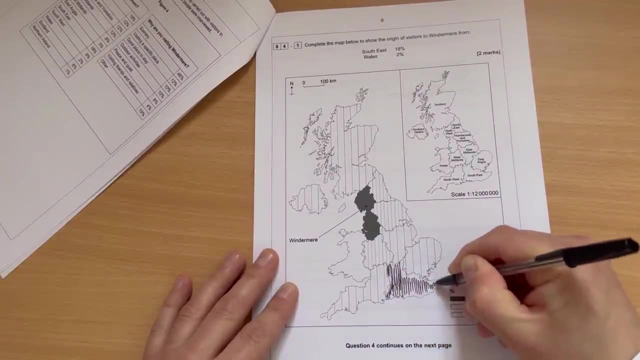 should colour that in, Like that now. As long as you colour it in fairly dark and it's obvious it's not the other two, You will get the marks You could. if you wanted to be double safe, you could put an. 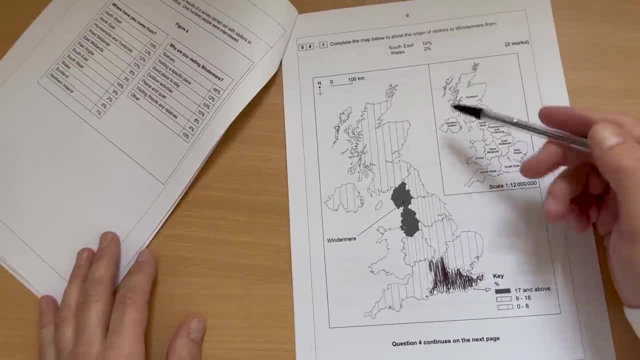 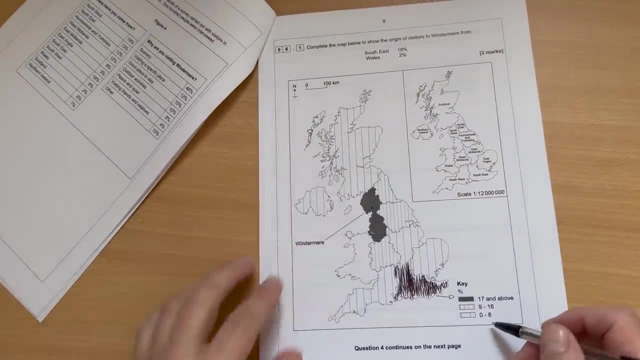 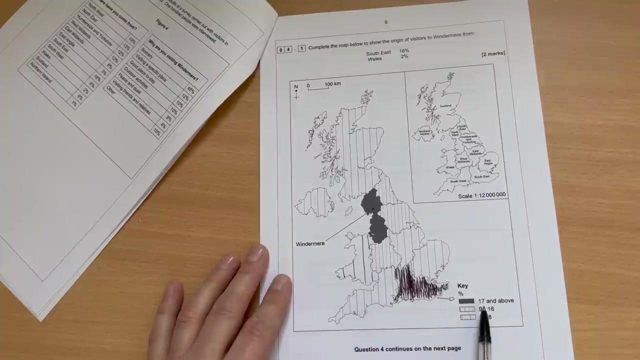 arrow there, but I don't think you need to. And the second one, Wales, is 2%. Just double checking It tells you up here. actually, Just make sure you put your lines far apart, Because if you put them close together, you're going to be representing 9% to 16%. Okay, 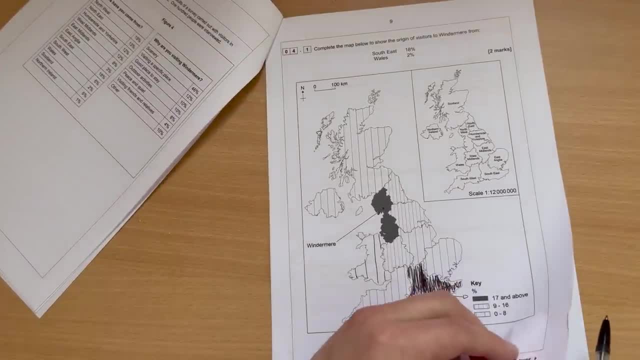 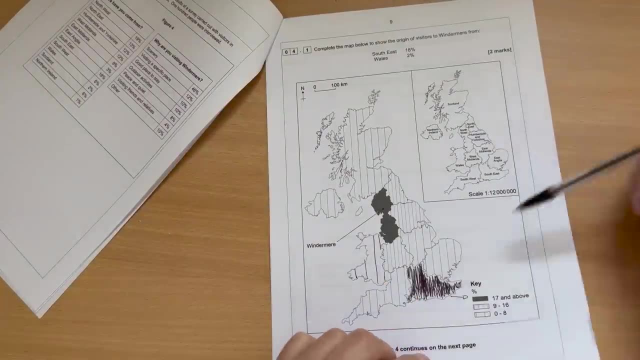 So that's nice, Too easy, Mark. Now the next question is: what will you do if you lose two marks when you're colouring in a map? If you see that map, alright, and you just flip onto the next page, you've lost two marks. 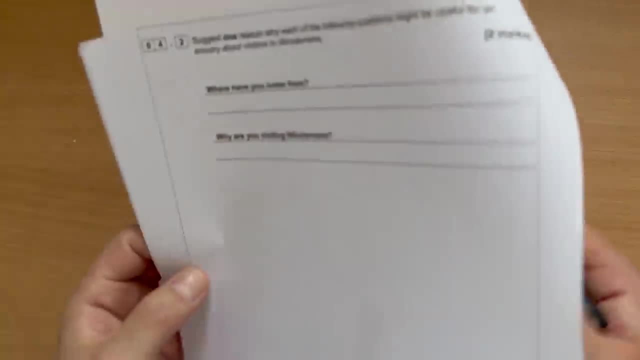 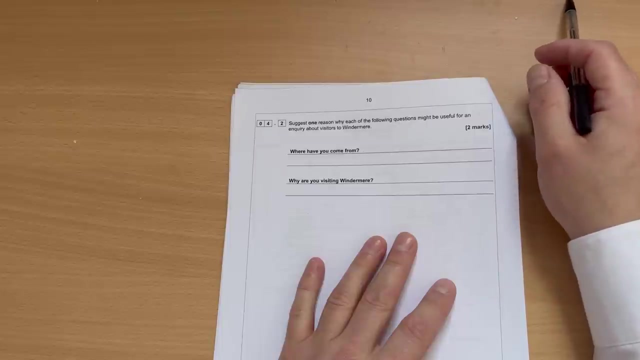 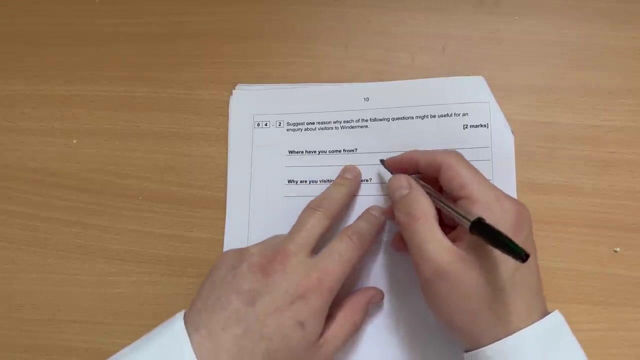 They're not going to put things in there just to fill the paper, but everything's got a reason. Okay, Suggest one reason why each of the following questions might be useful for an inquiry about visitors to Windermere. Now, where have you come from? Now, if this was international, you could maybe consider. 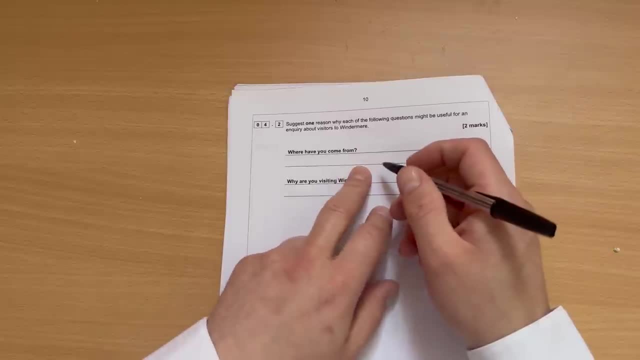 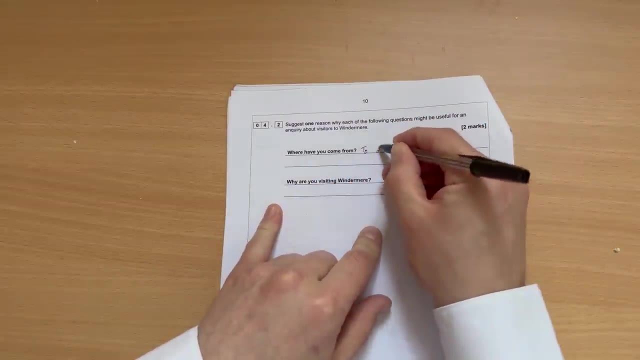 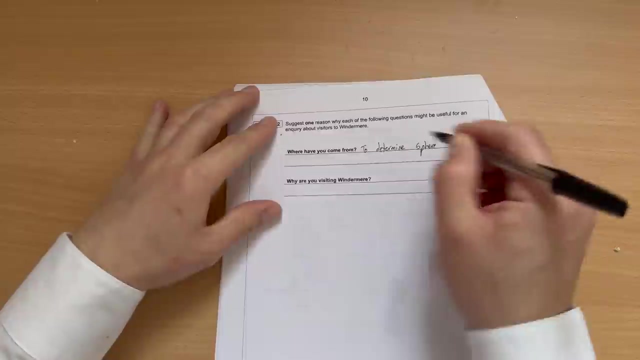 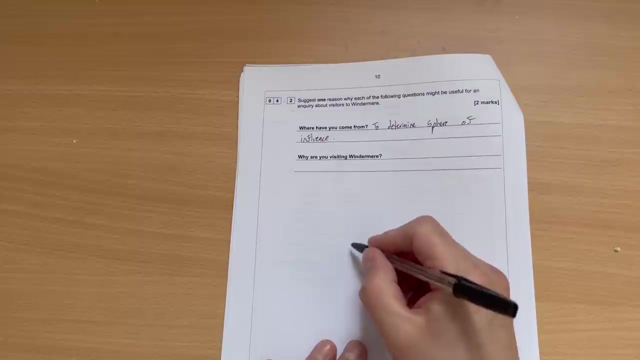 talking about Leicestershire. Yeah, like language boards saying welcome and directing people to places, but the one i would use is i'd write to determine sphere of influence, and that's a posh way of saying how big of an area does windermere attract people. so 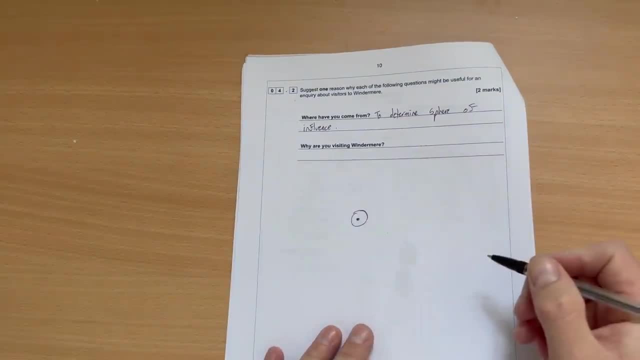 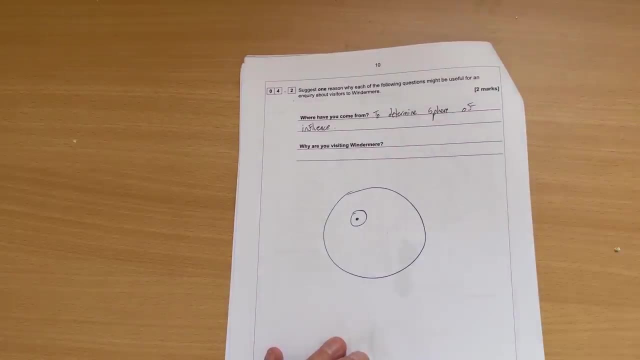 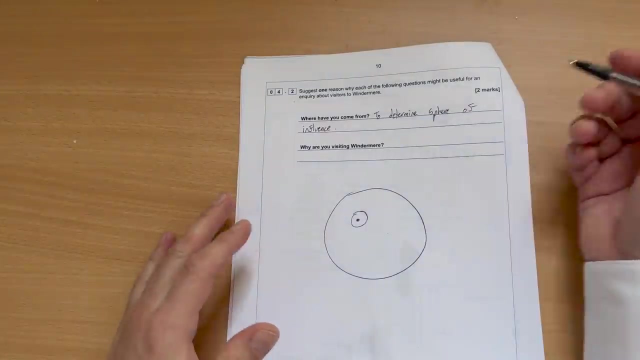 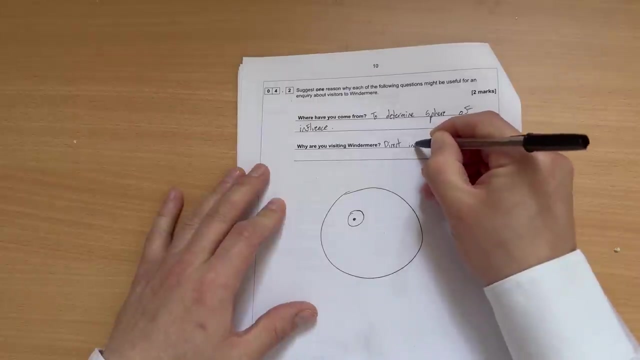 if i draw there, that would be a small sphere of influence, whereas that would be a big sphere of influence. why are you visiting windermere? um, for why are you visiting windermere? it could be, i don't know, maybe people are visiting to go boating. it will direct investment. 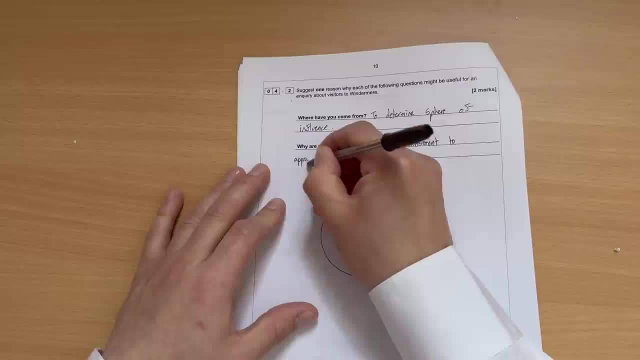 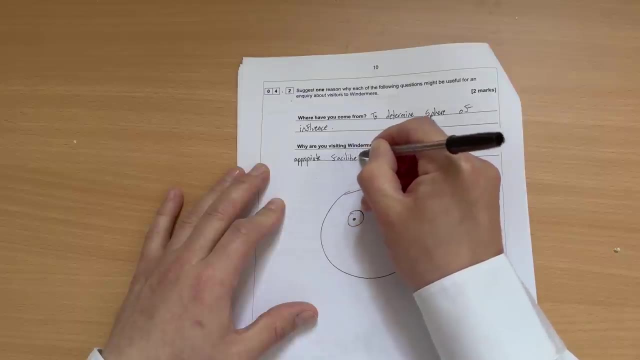 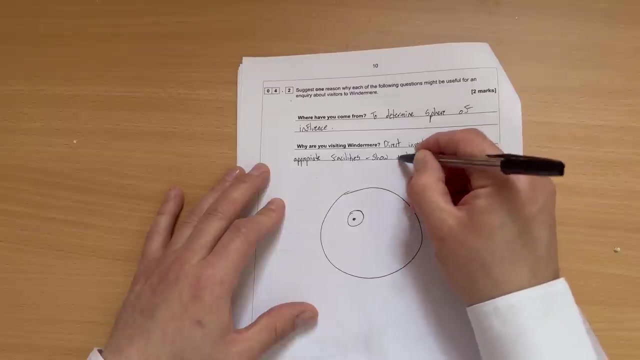 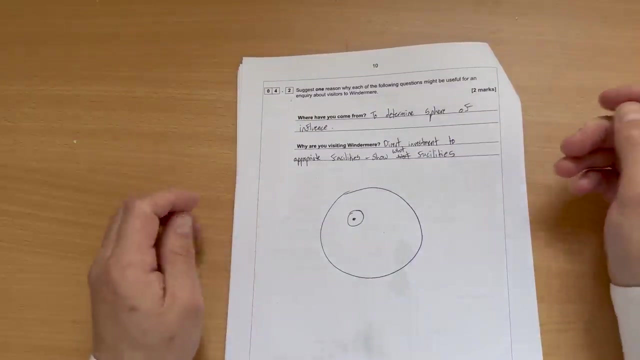 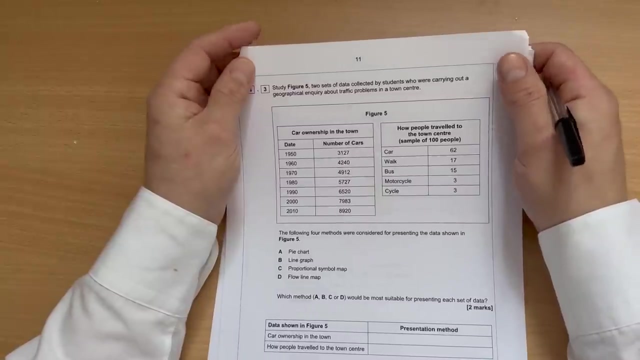 to appropriate facilities. okay, or it will show what facilities, what. how do you spell what? what facilities are required? so, as i said, if everyone says i've come to go on the boat, well, they might need more boats. two more marks right next. study figure five: two sets of data collected. 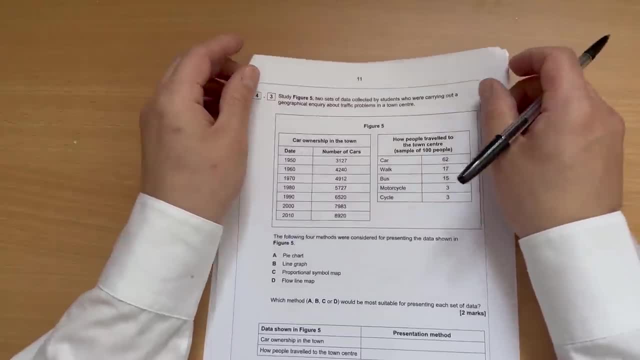 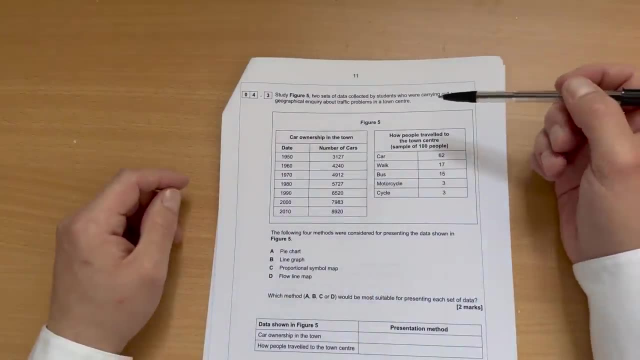 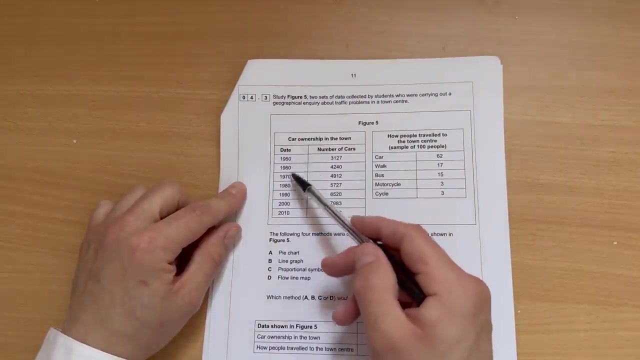 by students who were carrying out a geographical inquiry about problems in a town center. now it says car ownership in the town. so as time's going on, that's quite like straightforward, isn't it? as we go through the decades, the 10 years, more people on cars, hey. 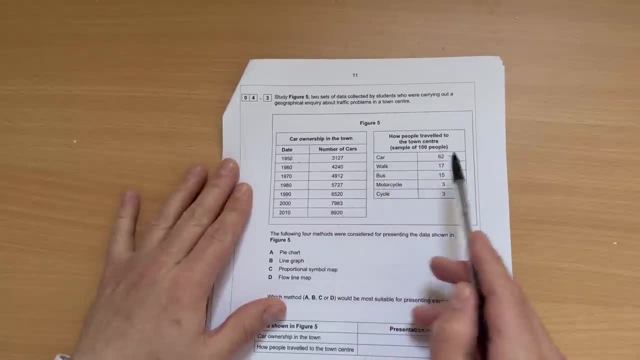 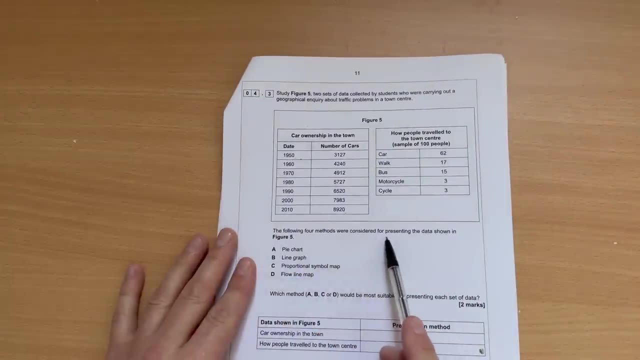 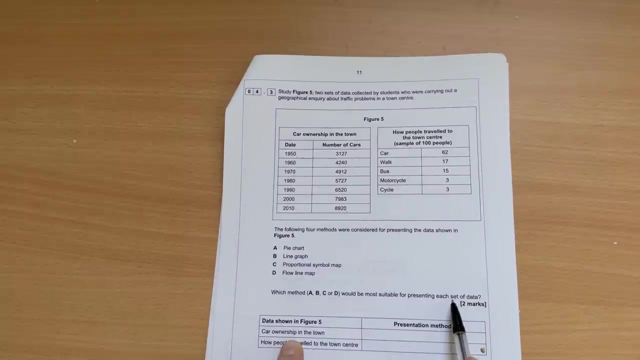 people travel to the town center out of 100 people. well, straight away i'm thinking pie chart. maybe we'll see. just to click on that topic at the beginning of this video, if you go to car ownership and see the first não, you'll see that here's a new method called the a, b, c, d. 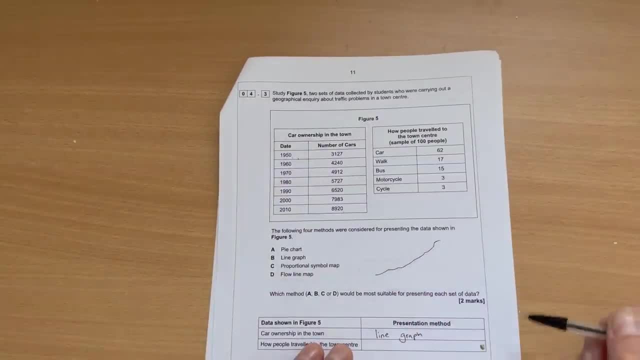 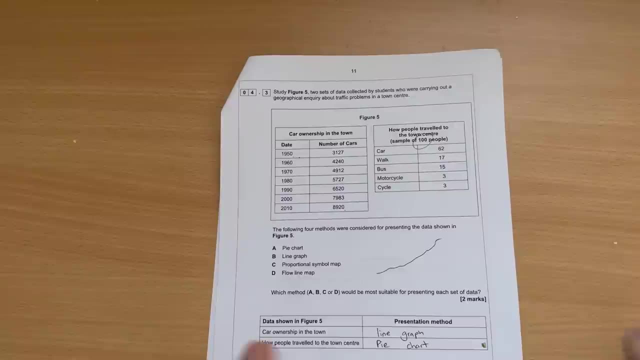 which is the same sort of thing that's used to look at cars. so a lot of people who are driving now. that makes sense right now in this situation. karen's on a lot of cars, so we'd like to know who's driving today. people, it makes sense to use a pie chart because pie charts are out of 100 percent, so that very 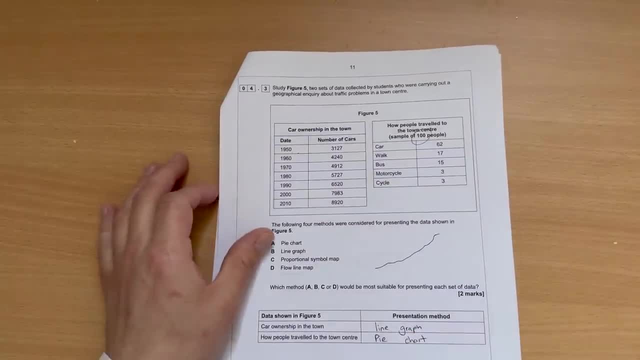 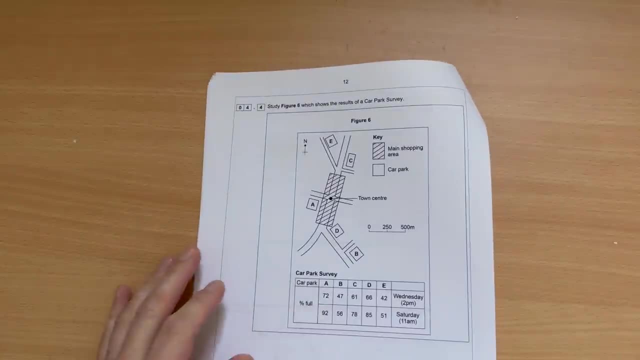 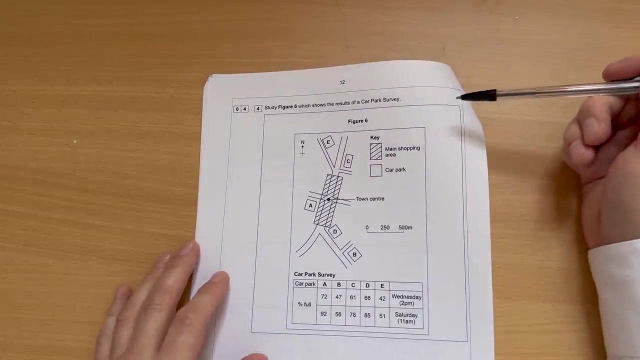 quickly showed the data, so we're looking at the most appropriate presentation methods. yes, yes, let's have a look at this one. so, question 4.4, study figure 6, which shows the results of a car park survey. okay, so we've got the town centre and we've got the main shopping area. 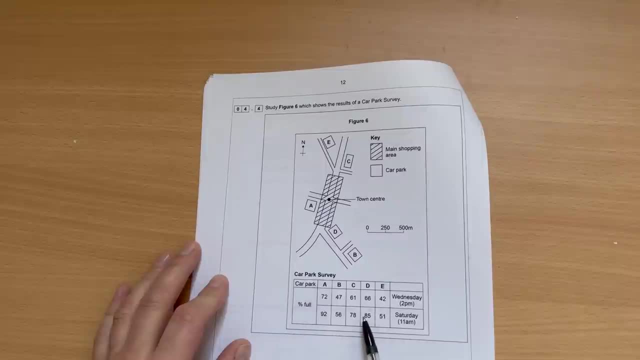 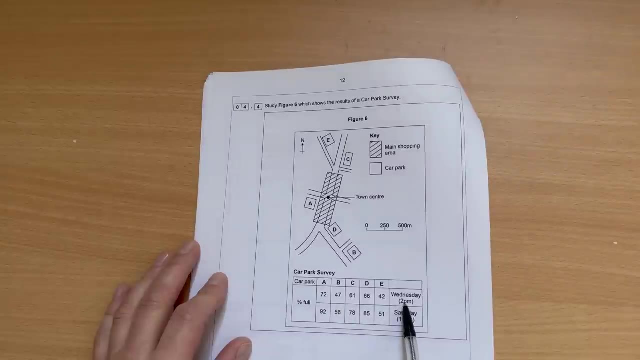 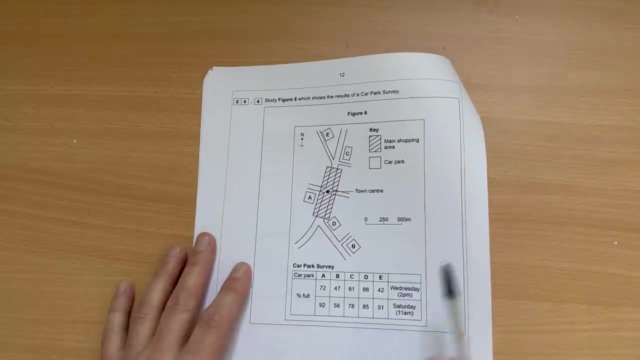 and these are the car parks, okay, and what it's showing you is how full they are at different times of the week. so wednesday afternoon 2 pm versus saturday at 11 am. now i just straight away. i'm thinking: well, the wednesday afternoon you might have people who are actually working. 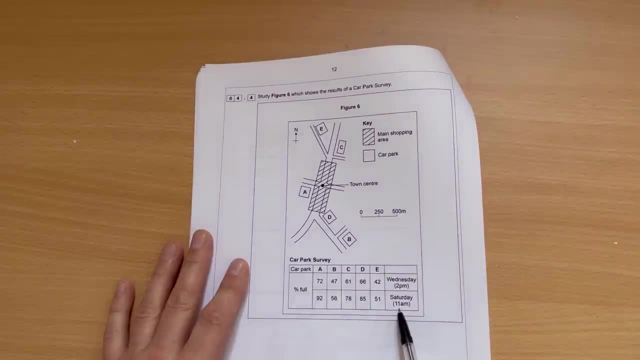 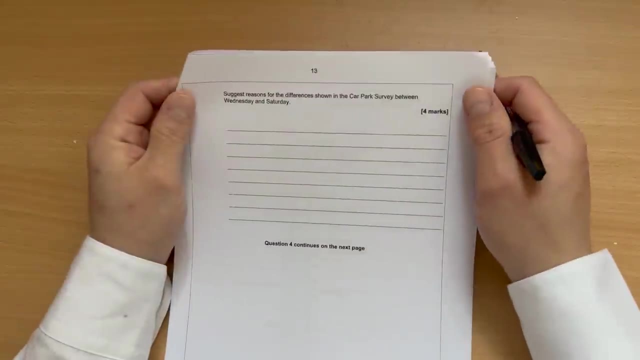 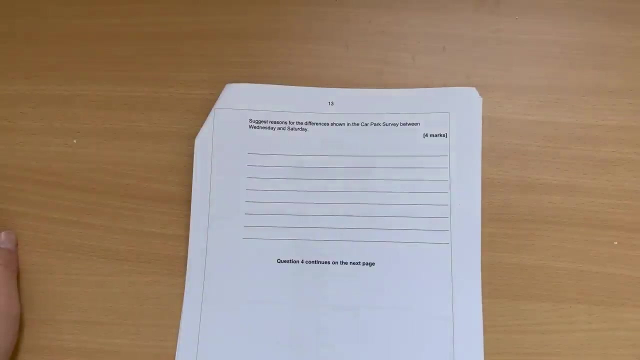 there or parked up for the day. but at the weekend, saturday 11 am, you're going to have prime time shoppers, aren't you? because that's when most people are off work to do their shopping. so it says, suggest reasons for differences shown in the car park survey between wednesday and saturday. 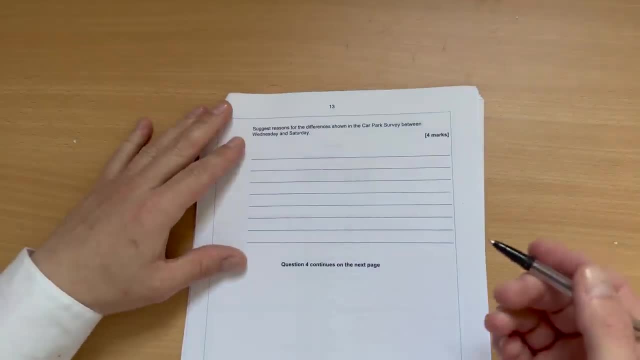 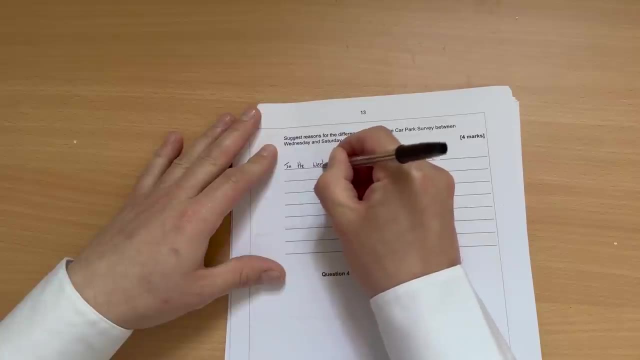 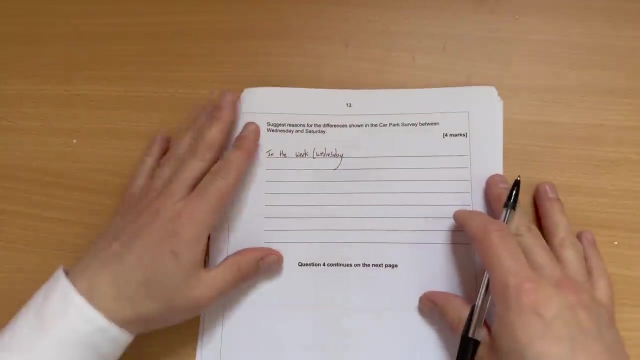 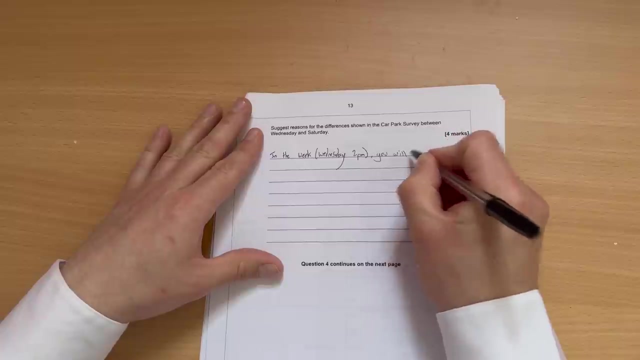 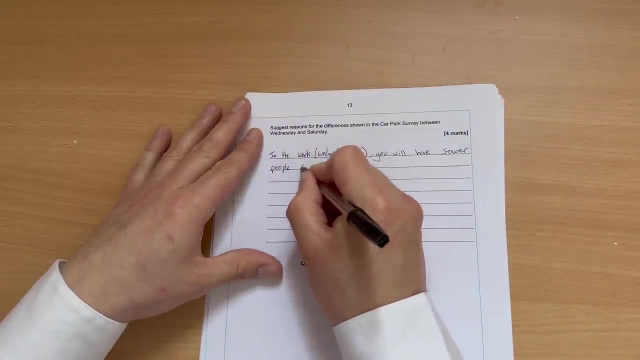 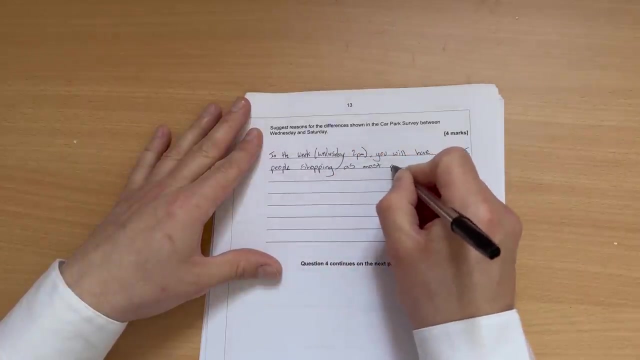 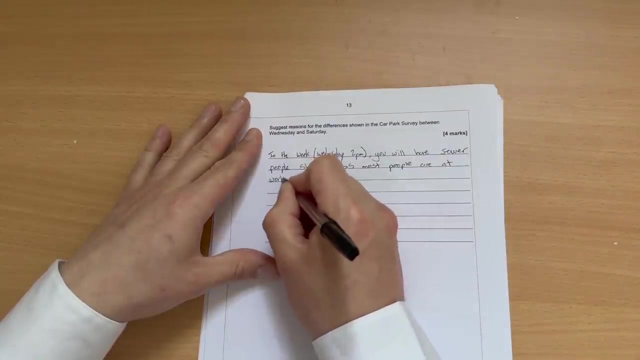 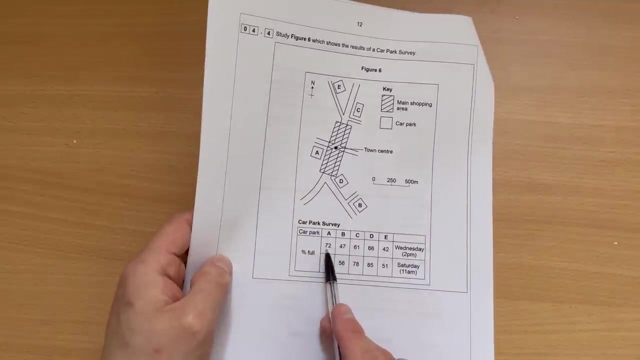 okay, so i'm going to think the first one. so in the week- wednesday, 2 pm, 2 pm comma- you will have fewer people shopping as most people are at work. then we need to use some data. for example, we'll use car park a versus b. now it's 20 percent different. 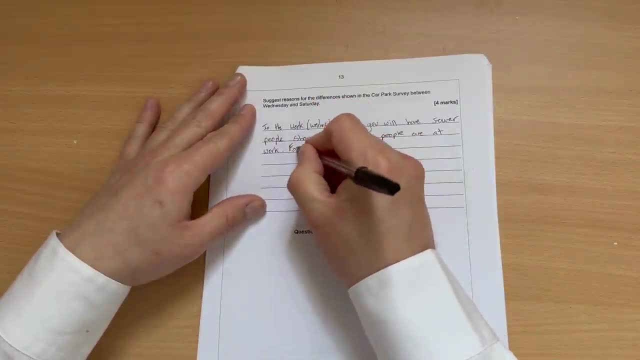 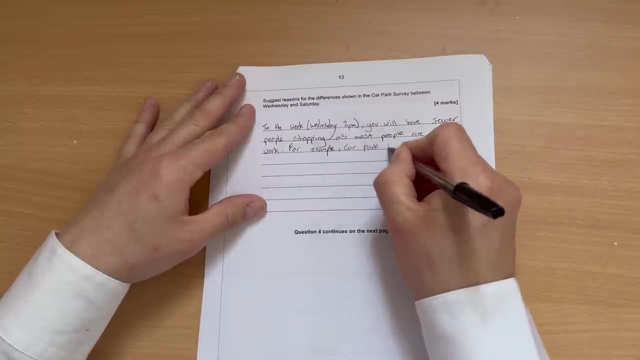 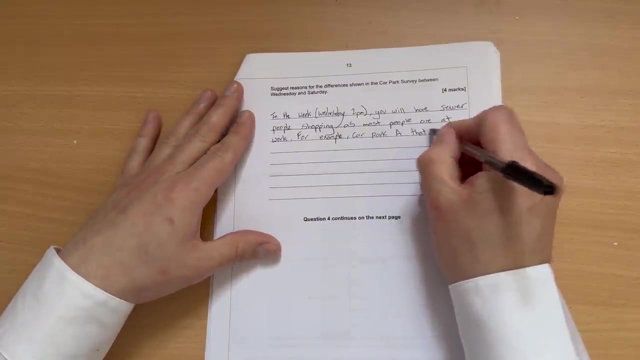 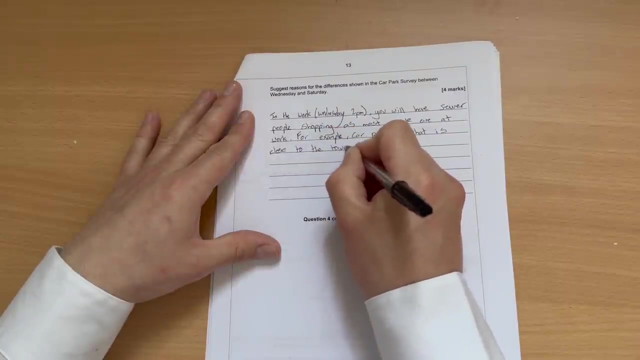 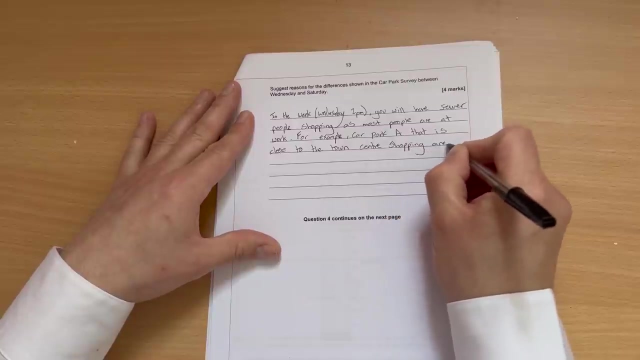 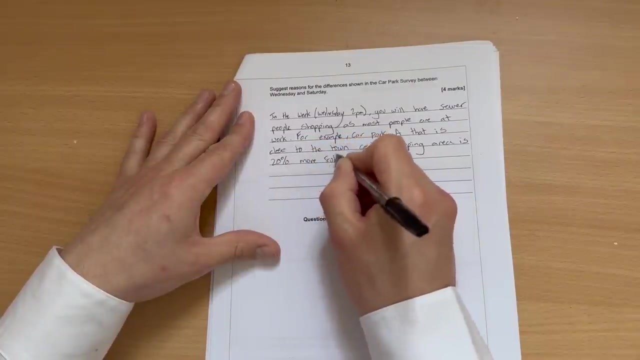 for example, comma car park a- how close is it? which is right next to the town centre. so that's there for you, so that's close to the town center. shopping area is 20 percent more full. that's not the best sentence. we'll be all right, more full. 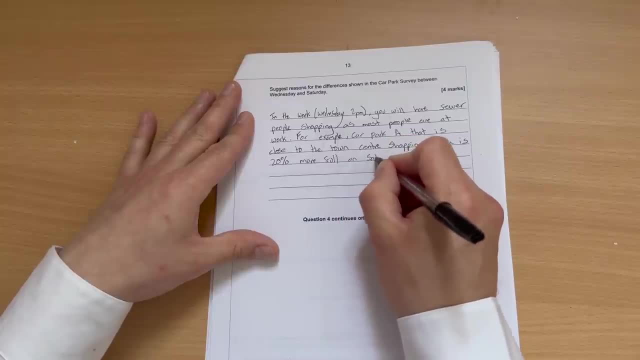 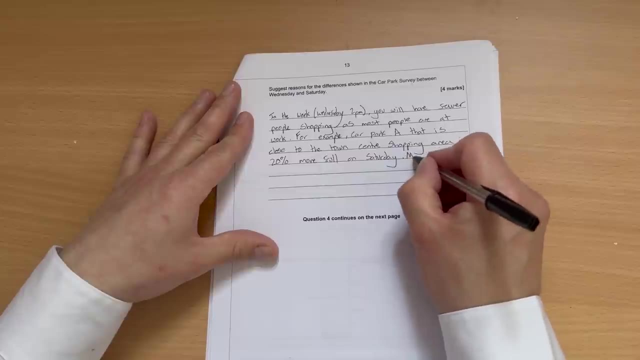 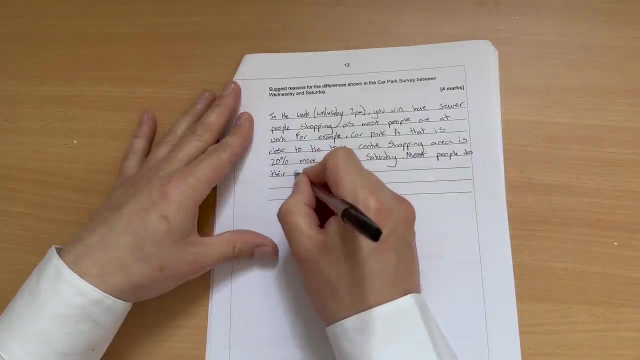 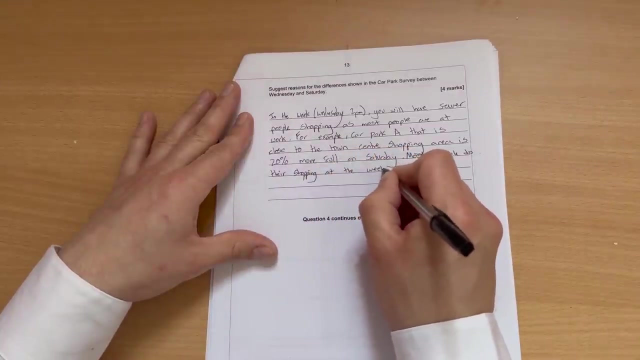 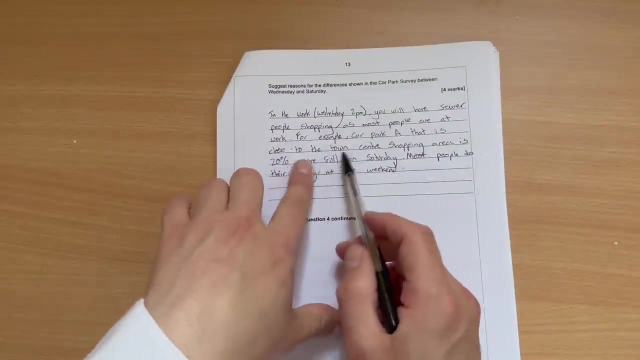 on saturday. that's exactly what you're doing. it's really busy free on saturday. okay, most people do their shopping at the weekend, so we've suggested- you know most people at work in the week. we've said that this car park is close to the 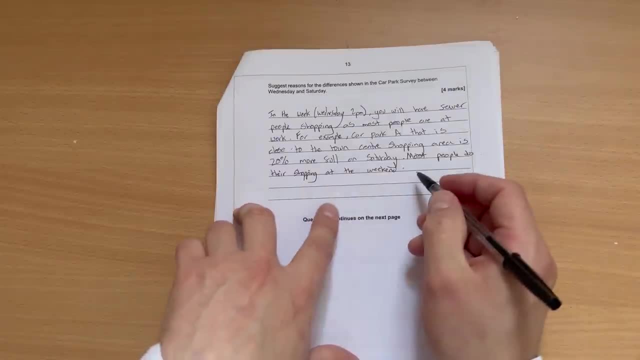 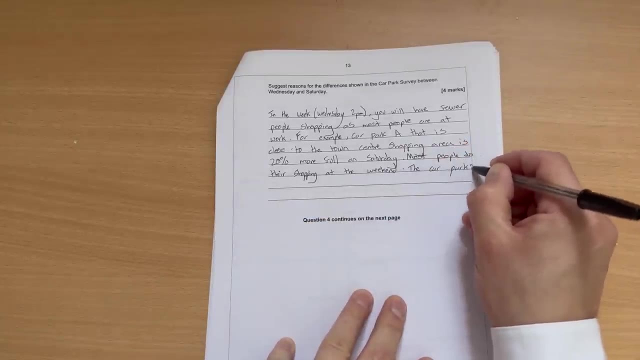 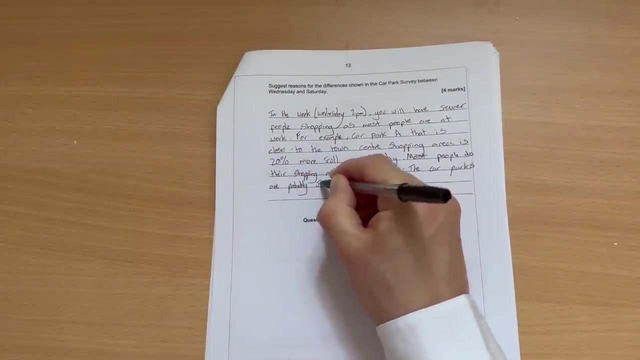 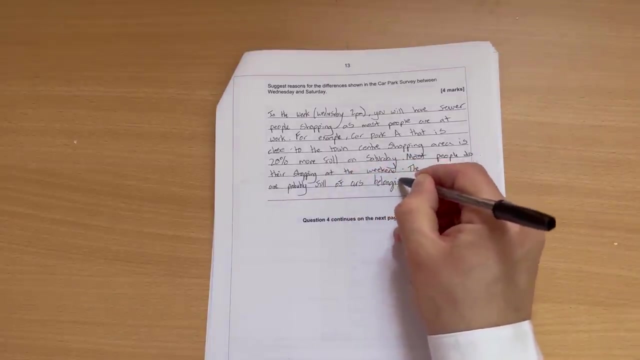 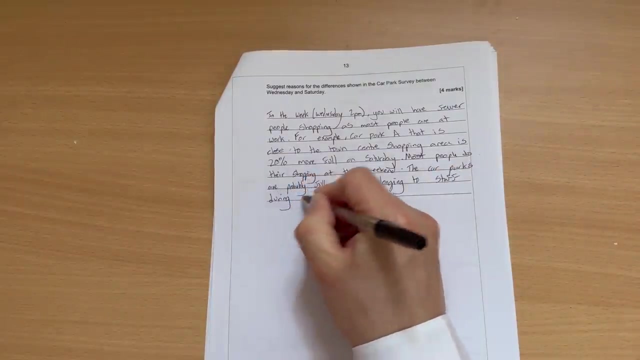 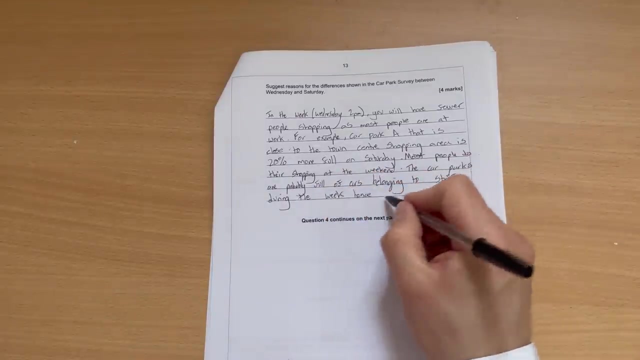 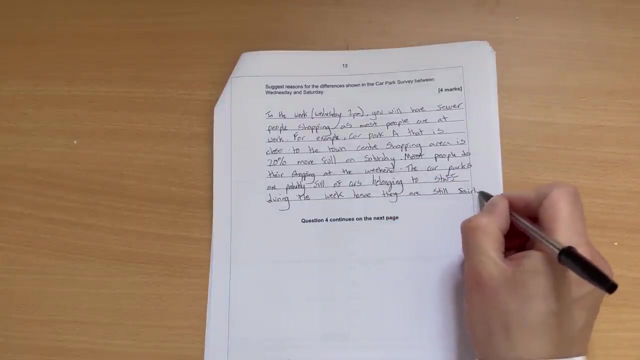 town, it's 20% more for some suggesting reasons. most people do shopping at the weekend. the car parks are probably full of cars belonging to staff during the week, hence, or this means that something along that line- hence, they are still fairly full. final model: what happens at the weekend? maybe there's a football match, or maybe 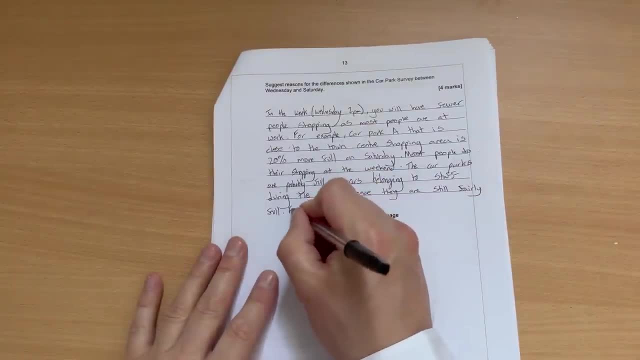 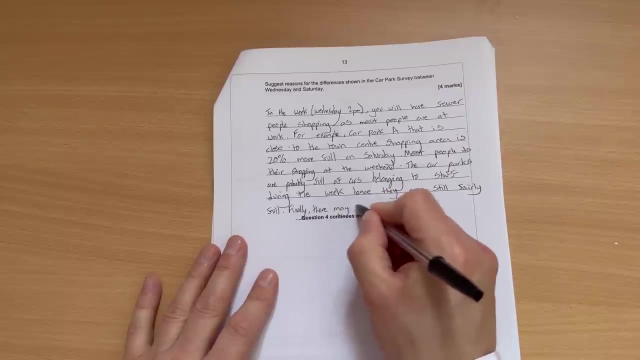 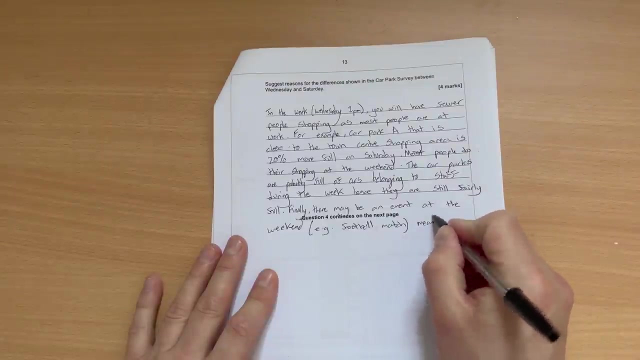 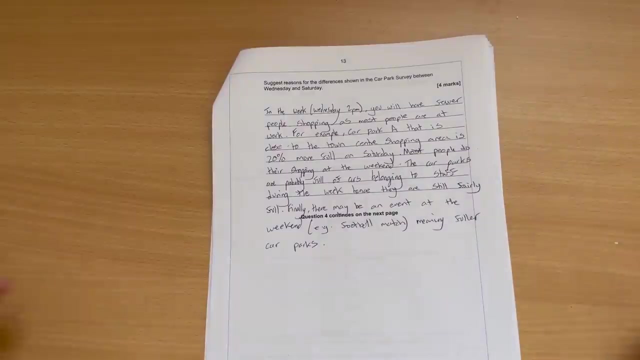 there's a- i don't know- some kind of carnival in the city. finally, there may be an event at the weekend in brackets, eg football match, meaning fuller car parks, okay again. so. so so we've said that this car park is close to the town and we've suggested- you know, 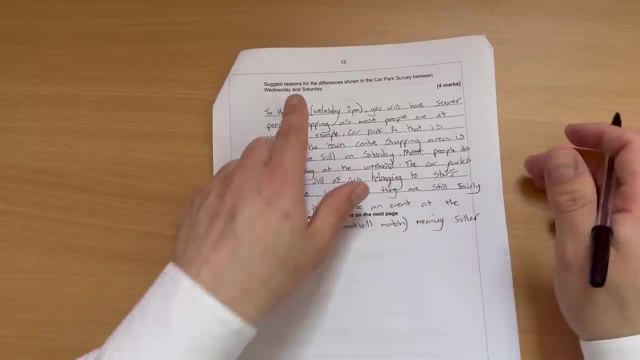 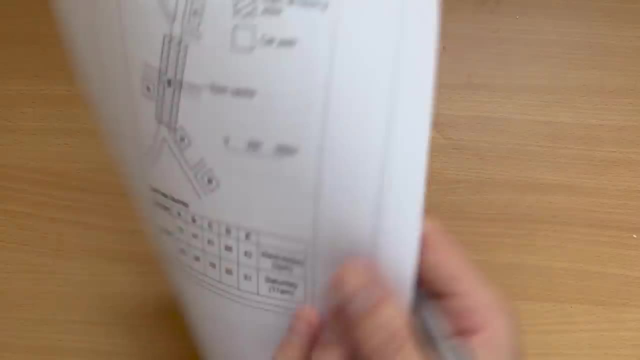 you're gonna get three or four marks. that's, i'd say, four marks. remember you're suggesting reasons. just imagine what. what are town centers like? all right, put yourself in the position if you're really struggling, draw a picture yourself. here's my look. hmm, what's going on there? okay? 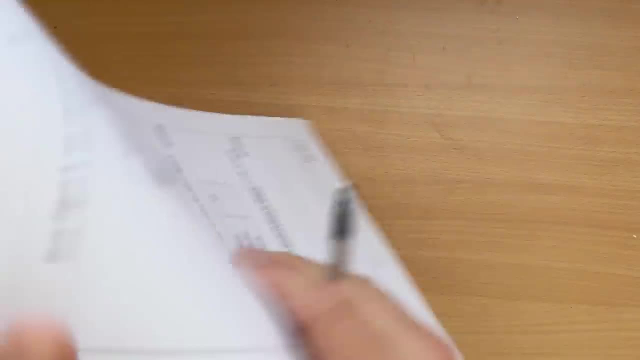 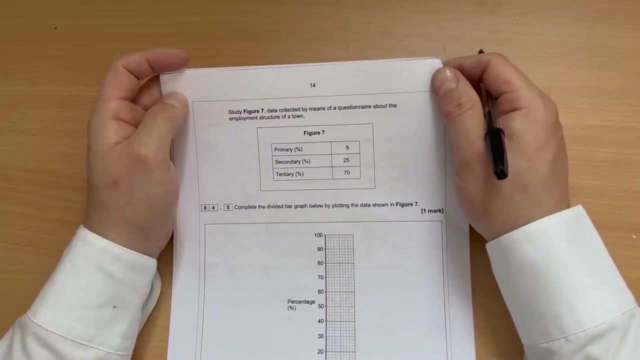 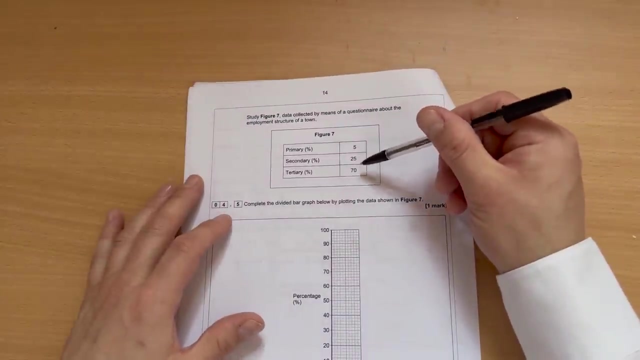 okay, study 7 data collected by means of questionnaire about the employment structure. so i'm going to get into the study seven data collected by means of questionnaire about the employment structure of the town. employment structure of the of a town. so we've got few in primary, 25 secondary, 70 tertiary, complete. 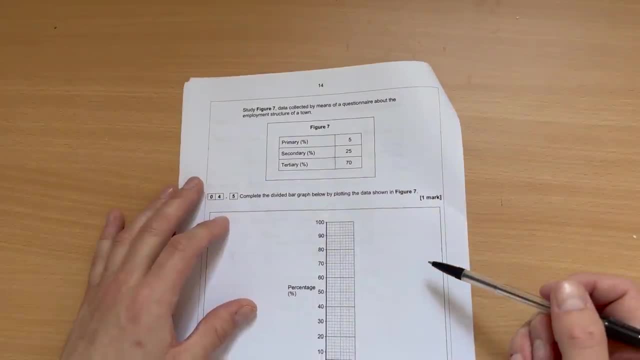 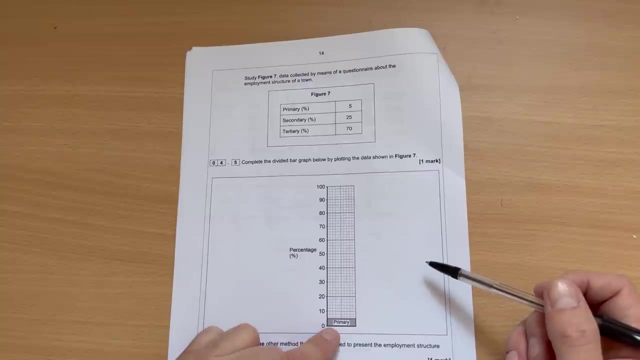 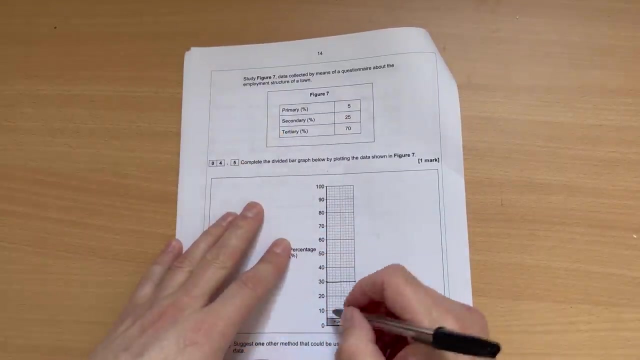 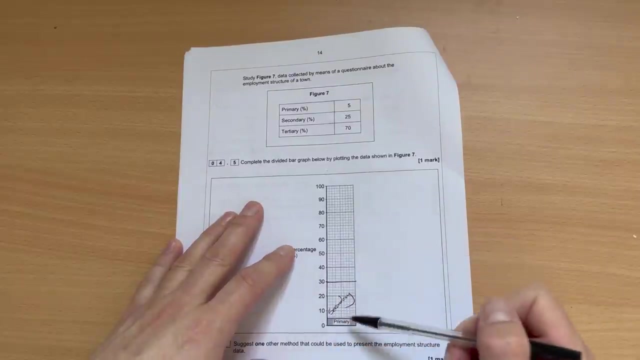 the divided bar graph by plotting the data. a lot of kids lose a market because they don't do both bars. so we've got primary already done. secondary: go up to 30, because 25 plus 5 is 30. secondary: some kids might go to 25 as well, but you already got five. five plus 25 is 30 and then all that's. 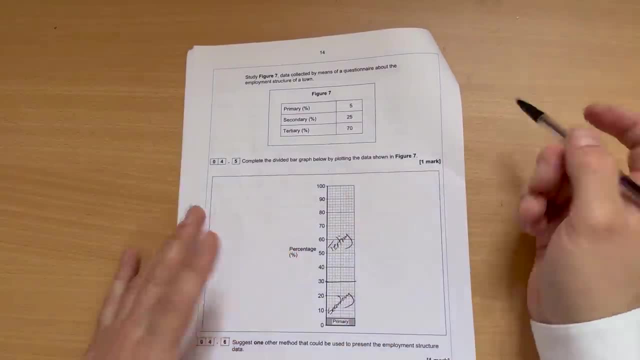 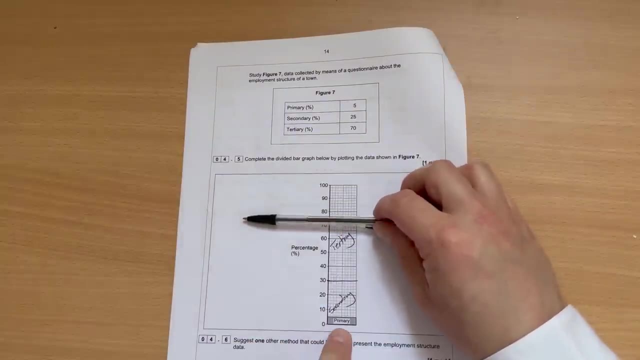 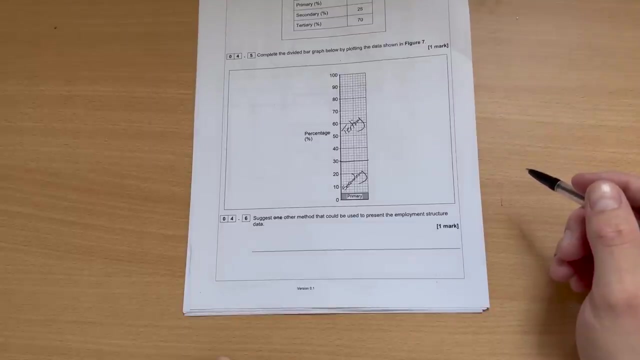 left is tertiary and that's the trick of doing that. all right, some people might do tertiary first and go up to 70. well, 70 minus the five primaries, any 65. uh suggest one other method that could be used to present the employment structure data well. 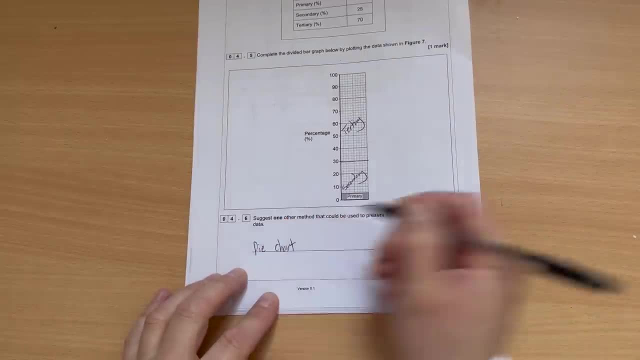 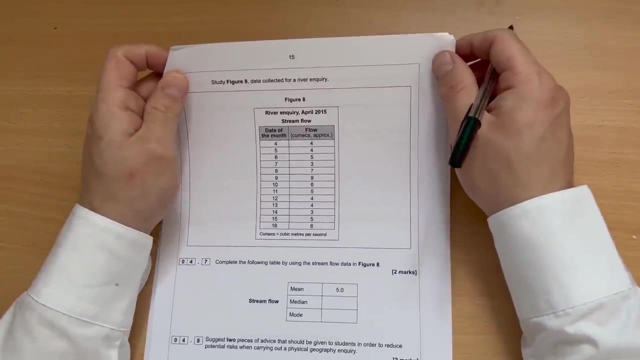 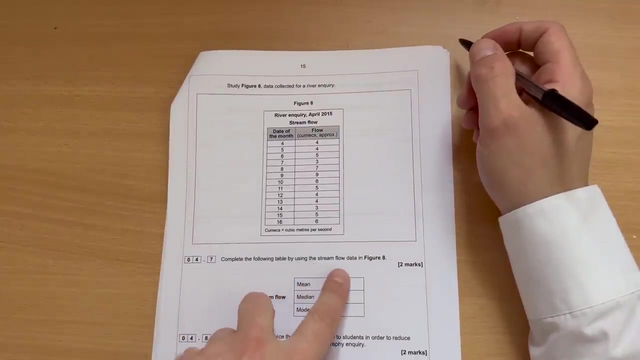 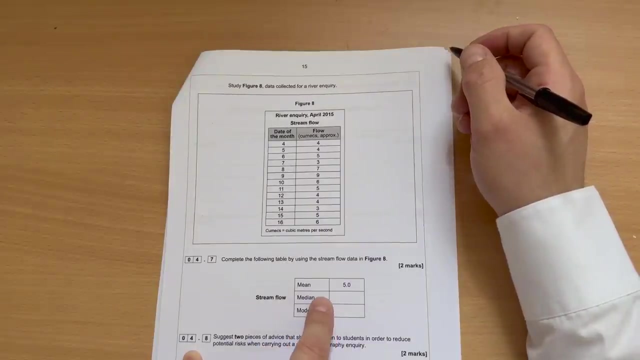 if you've got a percentage, i would go pie chart for your mark, okay. data questions, study- figure eight: data collected for a river inquiry. complete the following table using the stream flow data in figure eight. so median right to get the median you've got to put them all in order, so i would go about doing it like that. what's the? 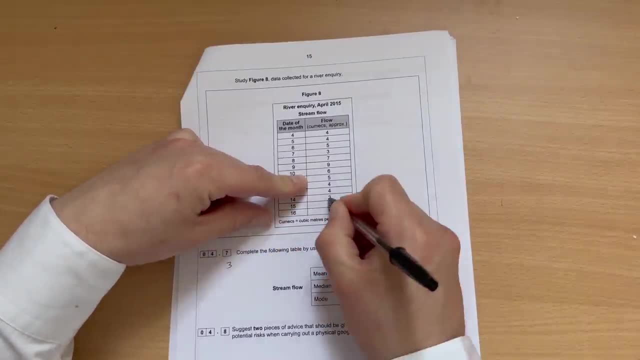 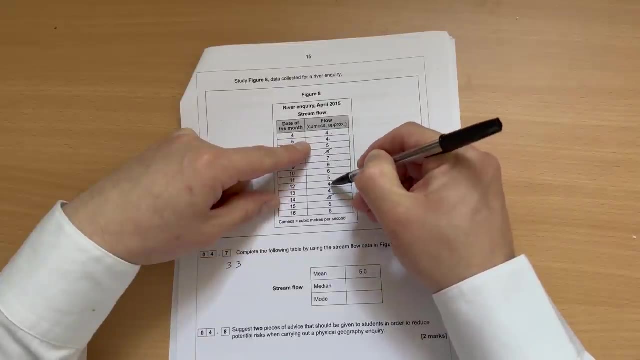 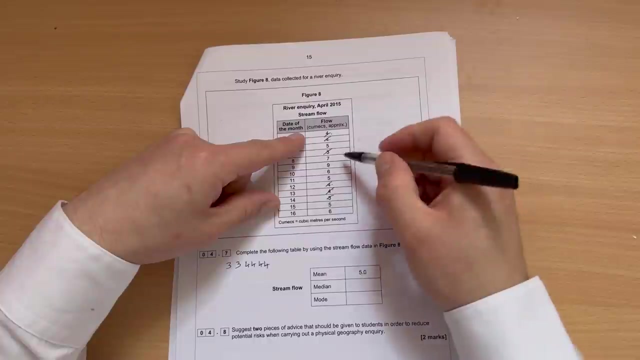 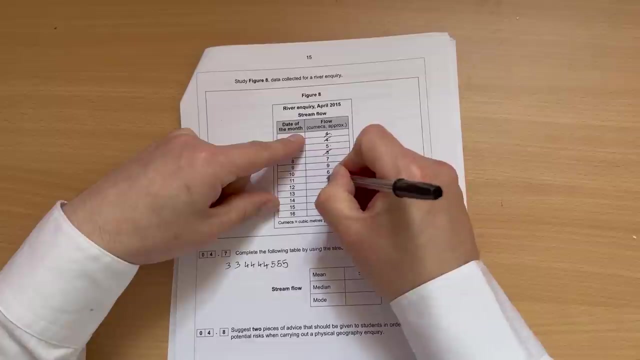 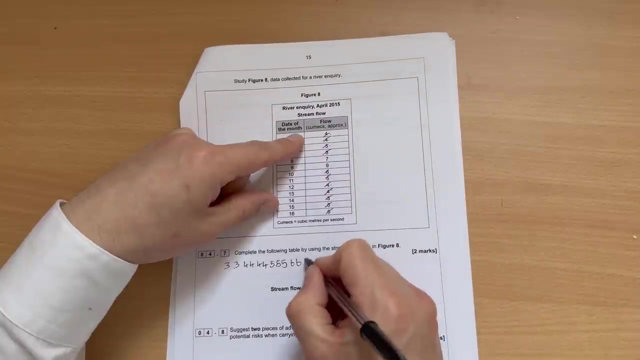 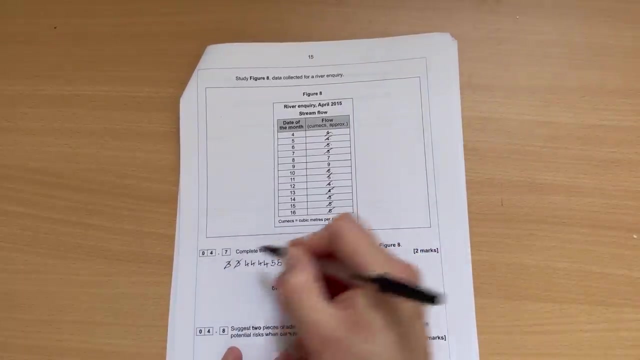 lowest number three, how many threes. so three cross, three cross. then next, how many falls? one, two, three, four, four, four, four, four. one, two, three, four, five. one, two, three, six, two, sixes. we've got one, seven and one nine. okay, now, median, we go get rid of one from each side. get rid of one from each side, get. 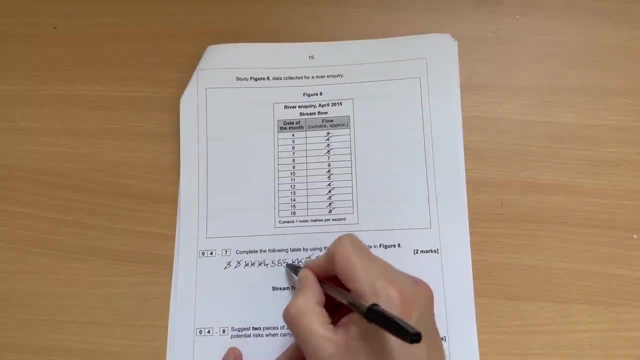 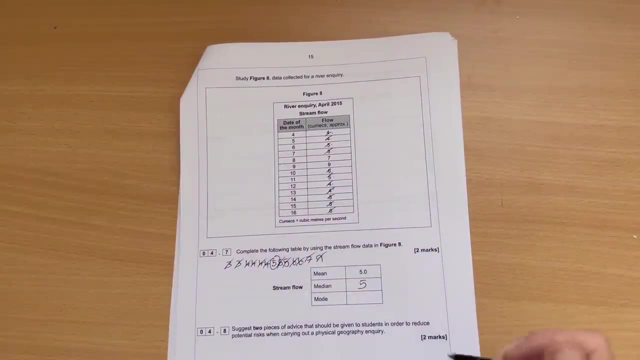 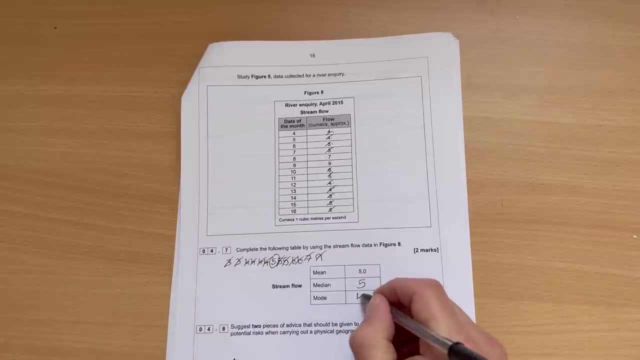 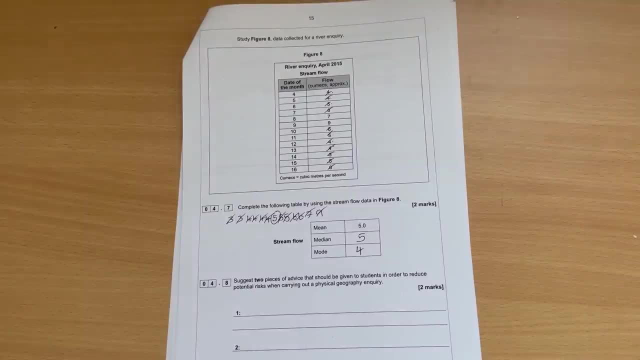 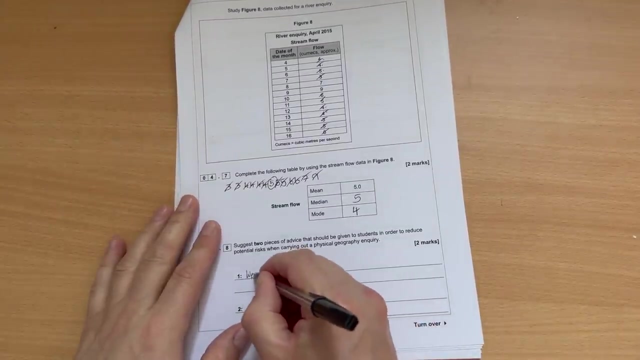 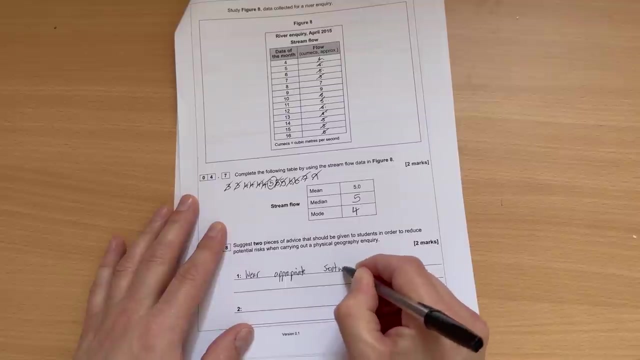 the next question suggest two pieces of advice that should be given to students in order to reduce the potential risk when carrying a physical geography. okay, easy peasy, all right, um, where appropriate, footwear to reduce slips and injuries. if you're walking up a river valley and you've got high heels on, you may as well call. 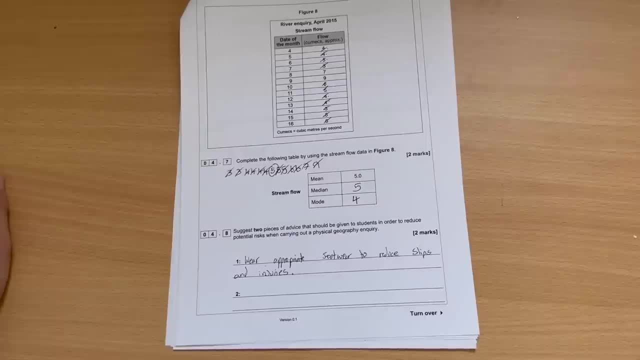 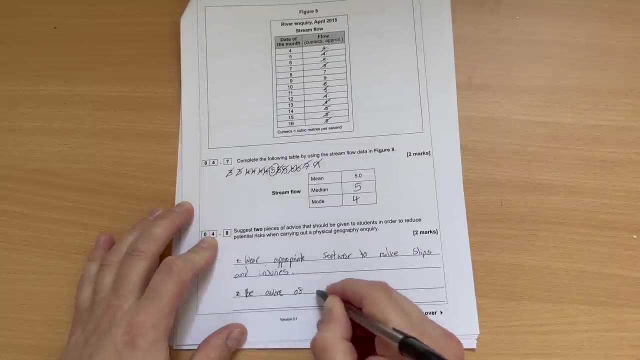 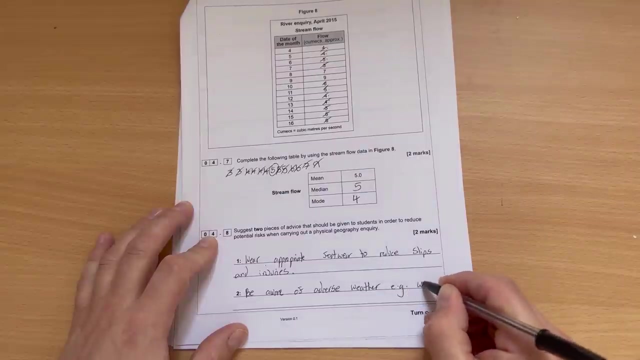 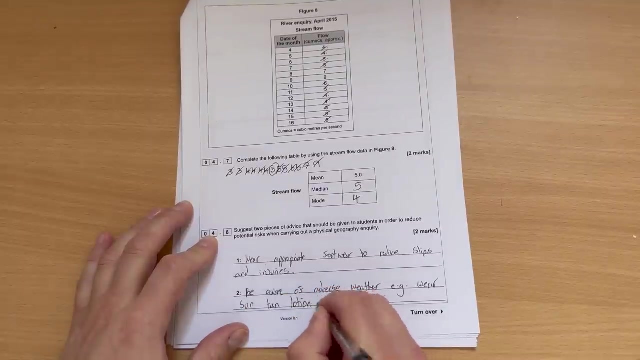 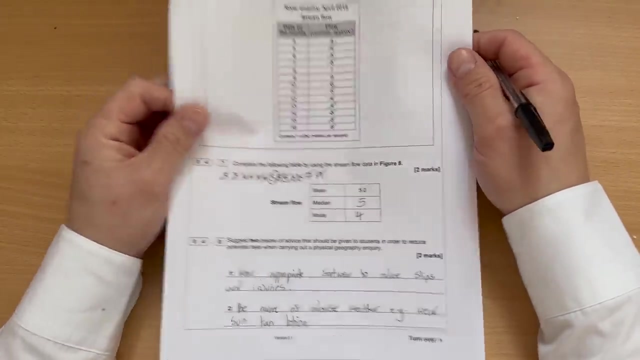 999 before you get out the coach. um weather, uh, be aware of adverse weather. eg wear sun tan lotion or wear a waterproof coat, other things, I don't know, other first aid kit available just in case you get hurt. it's just common sense now, when we get to, 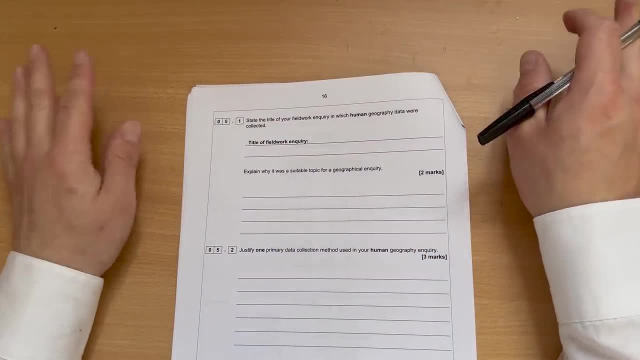 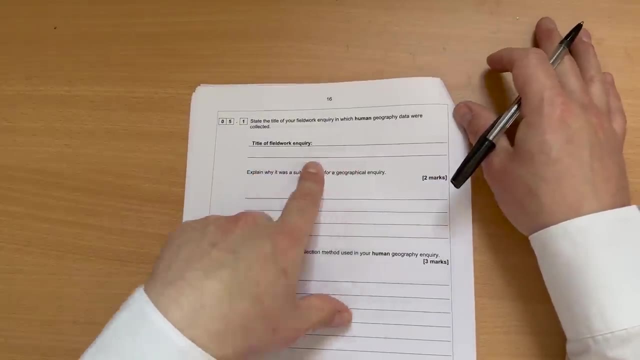 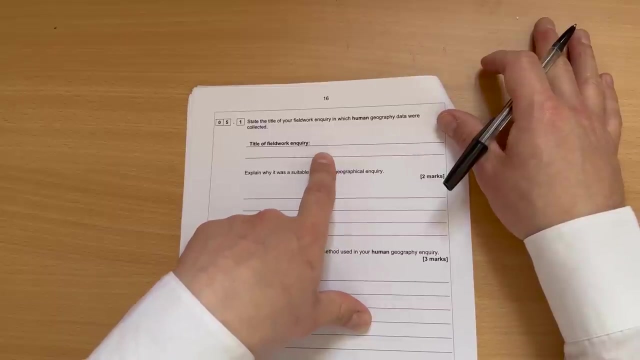 question five: this is not unfamiliar. this is your fieldwork now. these titles here. you don't need to spend forever writing them, you don't get a mark of that. but as someone who's marked the exam papers- or I haven't actually marked them, I'm a man, mr Batalas, he said, and we spoke to the example this gives them. 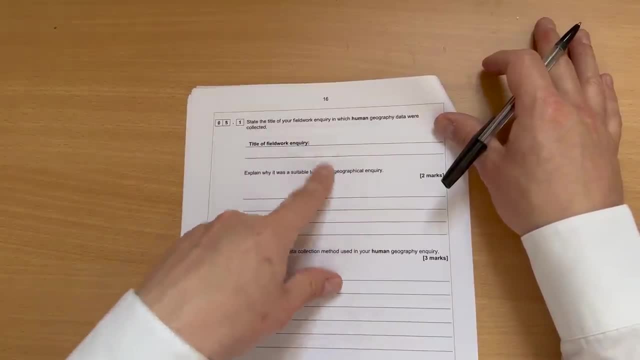 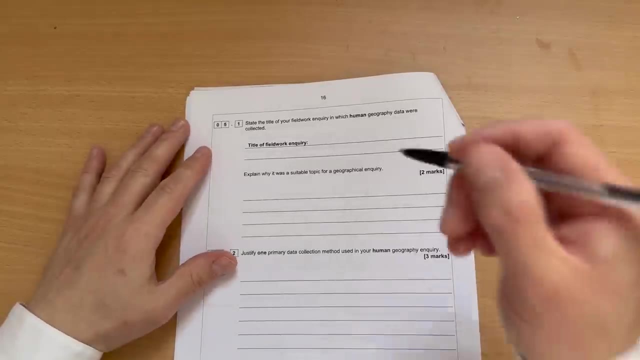 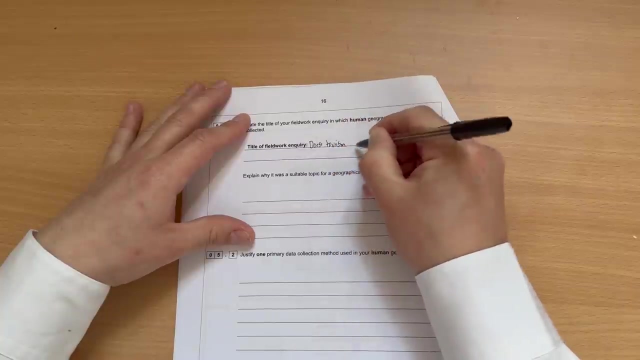 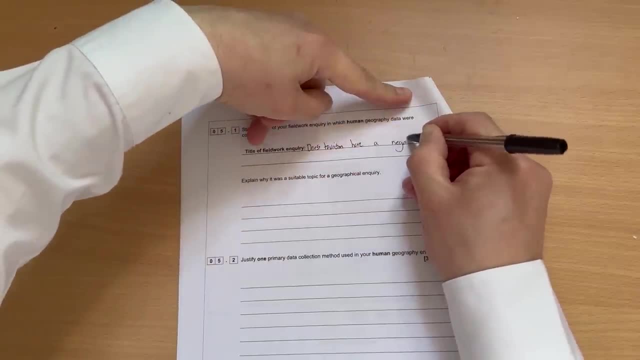 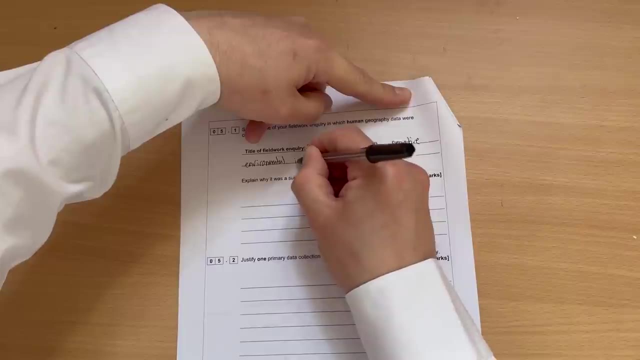 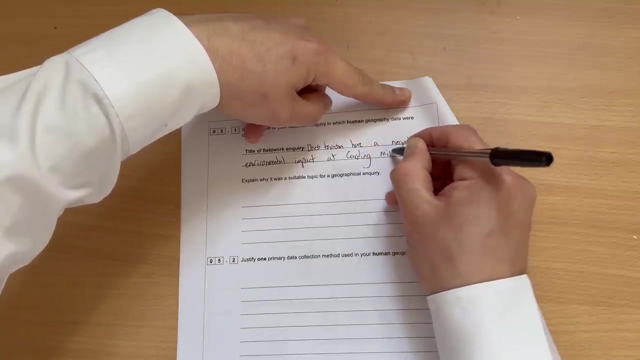 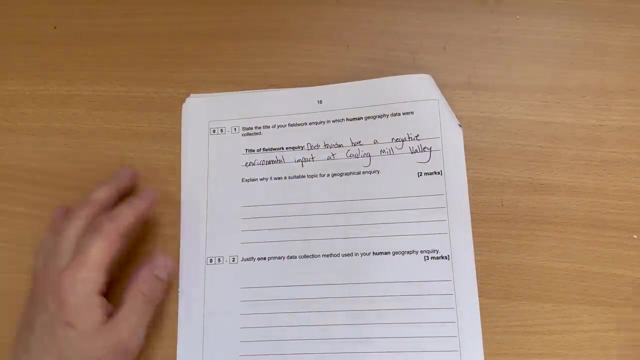 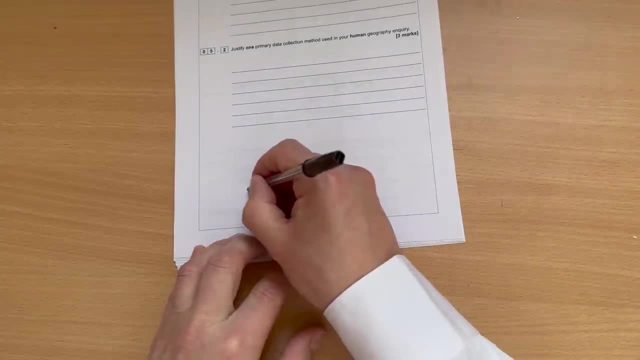 bottom here and I've got all the waterfalls and river valleys, but it's here and I've got all the waterfalls and river valleys, but it's here and I've got all the waterfalls and river valleys, but it's got a visitor center, all right. 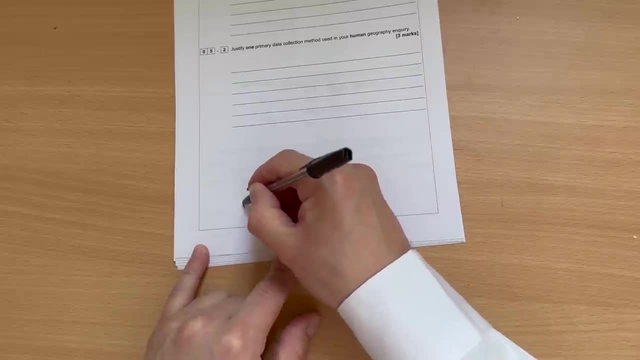 got a visitor center all right. got a visitor center, all right, where loads of people hang around to go for a where loads of people hang around to go for a where loads of people hang around to go for a way to have a sandwich, to buy an way to have a sandwich, to buy an. 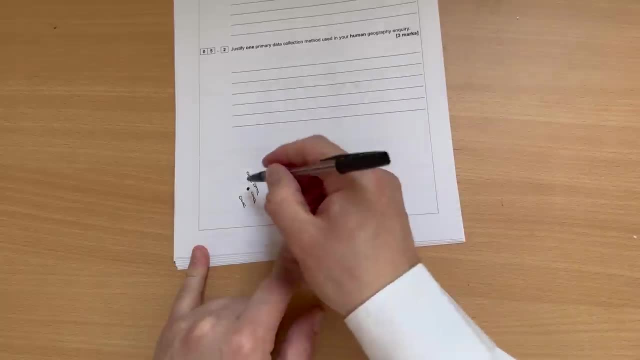 way to have a sandwich, to buy an ice cream- whatever it's a meeting spot. we ice cream, whatever it's a meeting spot. we ice cream, whatever it's a meeting spot. we were saying that the area here is gonna. were saying that the area here is gonna. 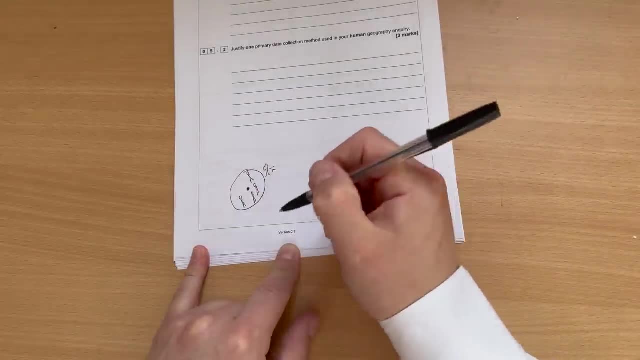 were saying that the area here is gonna have more environmental impact because have more environmental impact. because have more environmental impact because people are making noise dropping litter. people are making noise dropping litter. people are making noise dropping litter, etc. than the areas further away. this, etc. than the areas further away this. 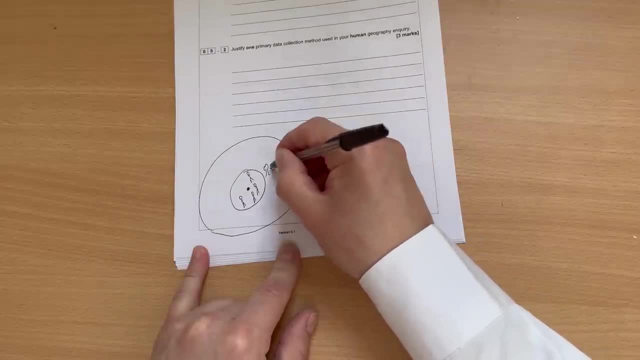 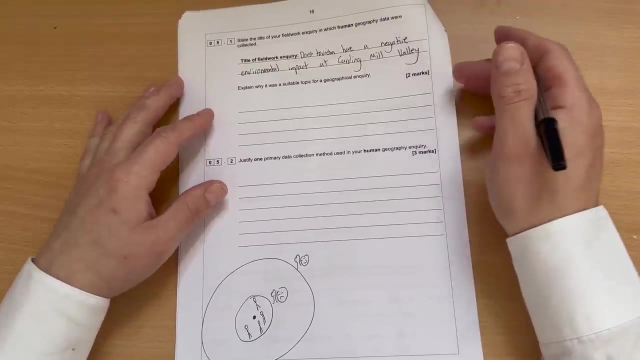 etc. than the areas further away. this would have less environmental impact, or would have less environmental impact, or would have less environmental impact, or at least that's the theory. so why this? at least that's the theory. so why this? at least that's the theory. so why this was suitable for a geographical inquiry. 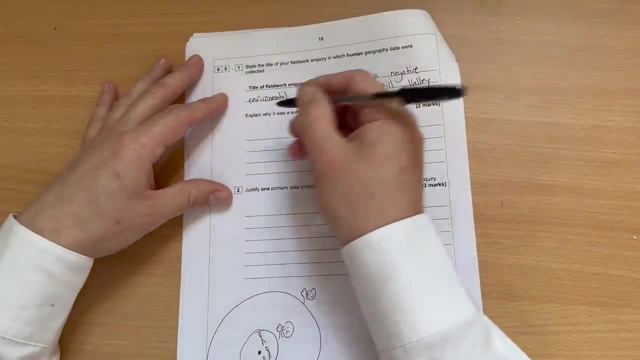 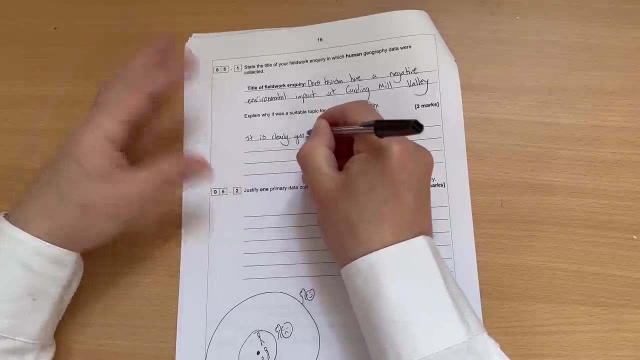 was suitable for a geographical inquiry, was suitable for a geographical inquiry. well that the total. it is clearly well that the total. it is clearly well that the total. it is clearly geographical, it's a geography question. geographical, it's a geography question, geographical, it's a geography question. and 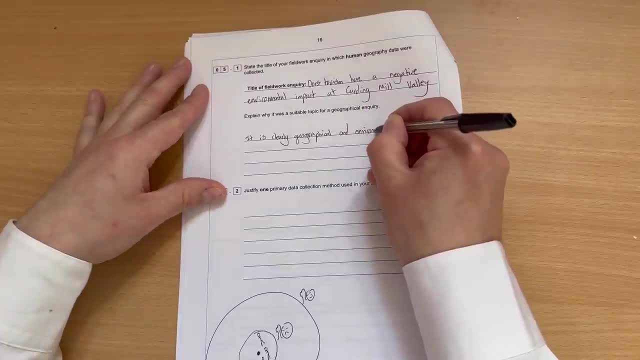 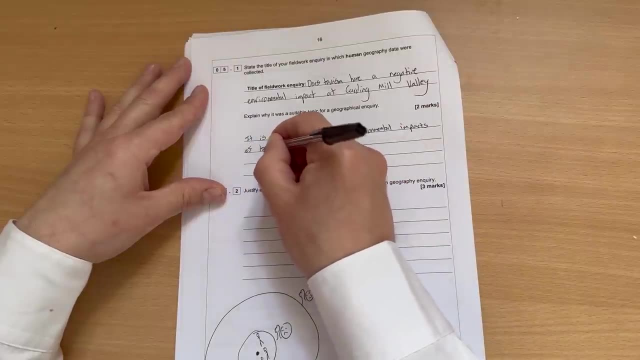 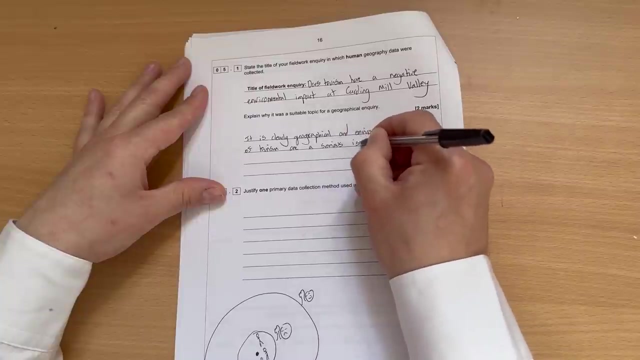 and and and environmental impact, impact, impact of tourism- are a serious issue. are a serious issue. are a serious issue. if you don't believe me, look at the. if you don't believe me, look at the. if you don't believe me, look at the pre-release 2023. it's talking about. 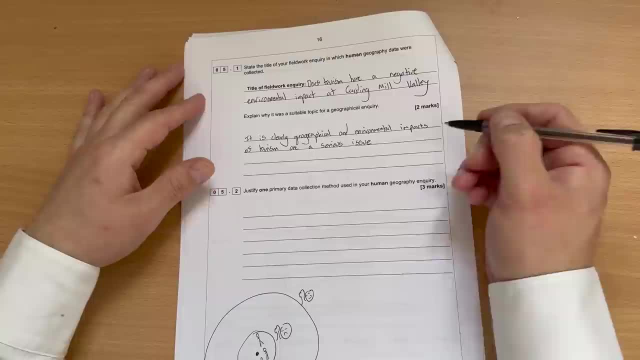 pre-release 2023. it's talking about pre-release 2023. it's talking about building a port: building a port. building a port for more tourists, but the mountain about for more tourists, but the mountain about for more tourists, but the mountain about the environmental issues, such as turtles. 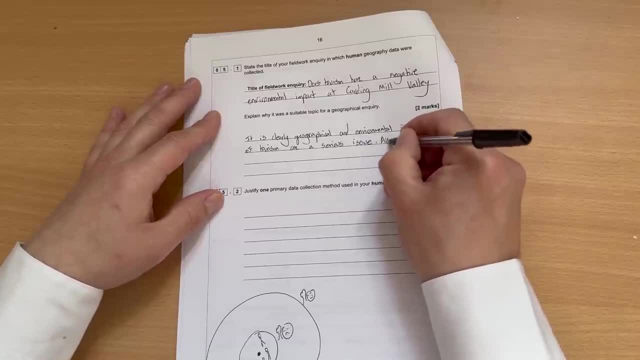 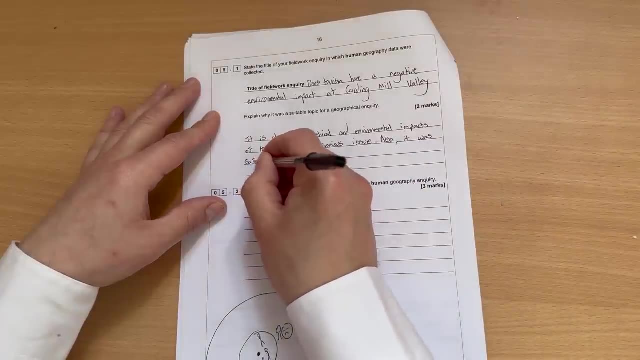 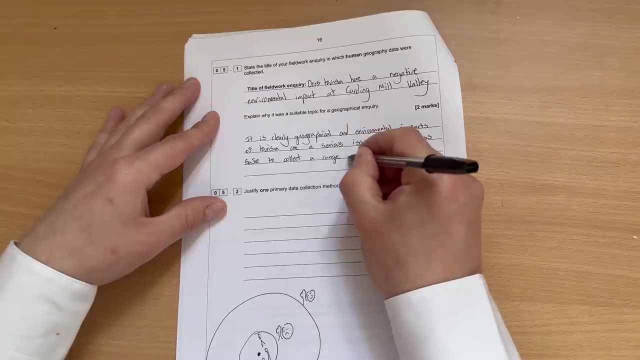 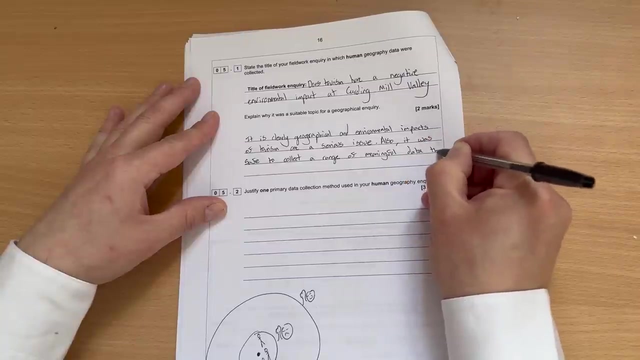 the environmental issues such as turtles, the environmental issues such as turtles becoming an extinct, becoming an extinct, becoming an extinct also also also have have uh, it was, uh, it was, uh, it was safe. safe. safe to collect, to collect, to collect a range, a range, a range of meaningful data. 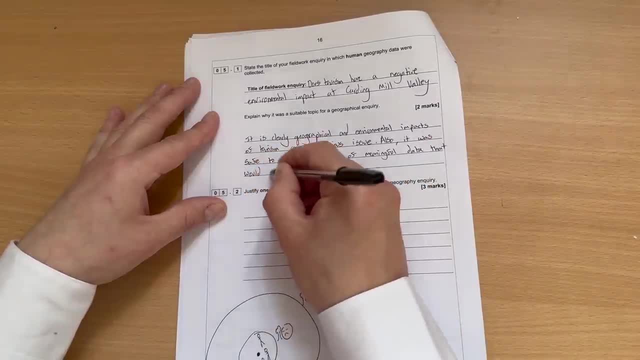 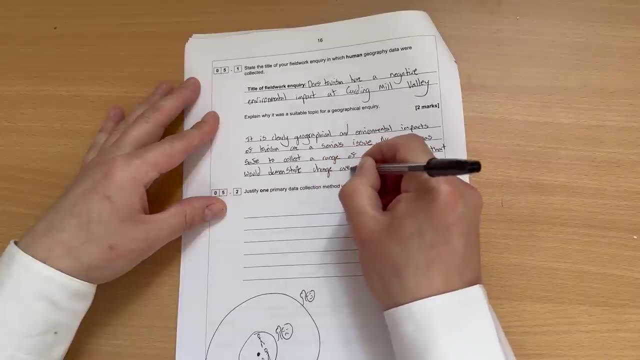 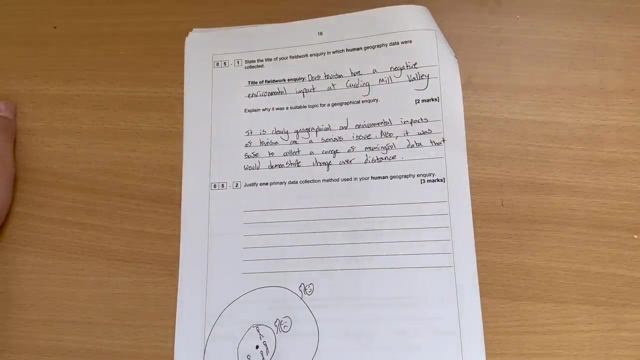 that would. that would. that would demonstrate change, change, change over distance. you could have talked about the fact that, well, the CardioMobility is maintained by the National Trust. It was easily accessible by coach. The footpaths are maintained, But yeah. 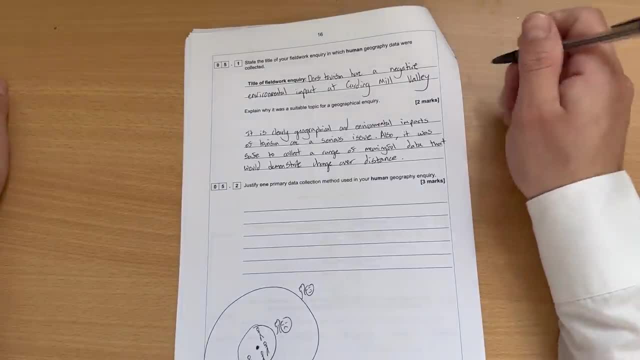 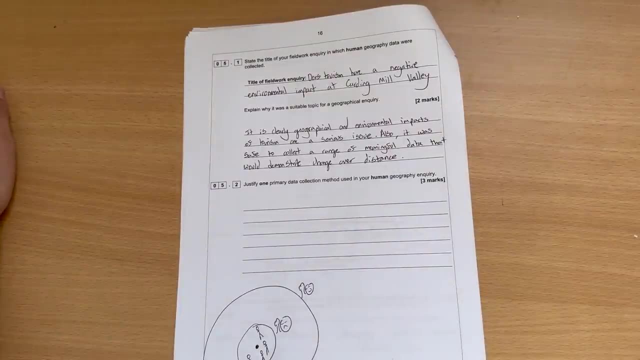 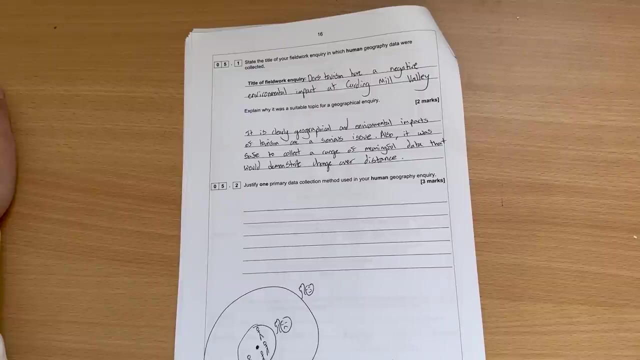 Okay, next question: Justify one primary data collection method used in your human geography inquiry. Now I'm going to have a quick look at the mark scheme here, because it's three marks. It says one method with detailed justification equals three marks. 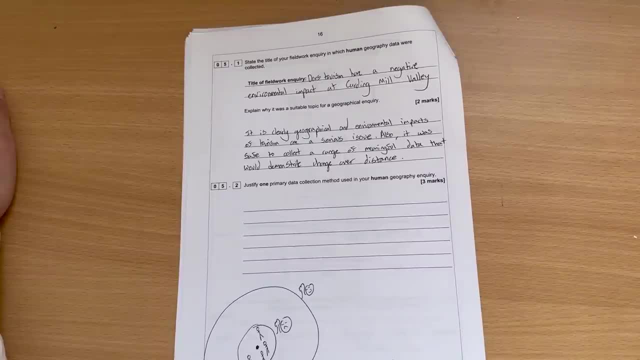 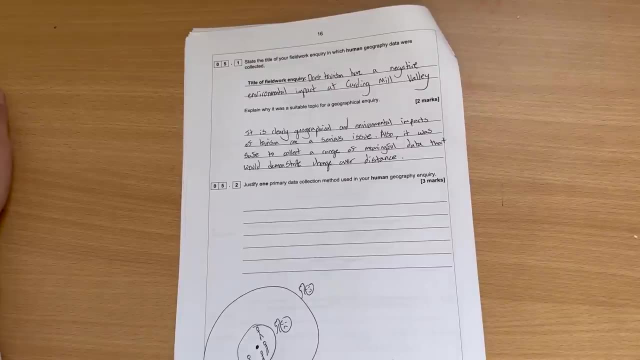 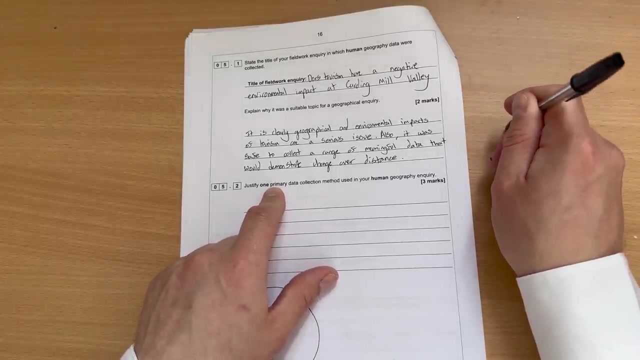 Some justification in relation to aims of investigation: two marks Statements with an element of employed. element of justification equals one mark. So primary is data you collected yourself, So we used environmental surveys. If it was secondary, we'd be looking at photographs, historic maps, other people's studies. 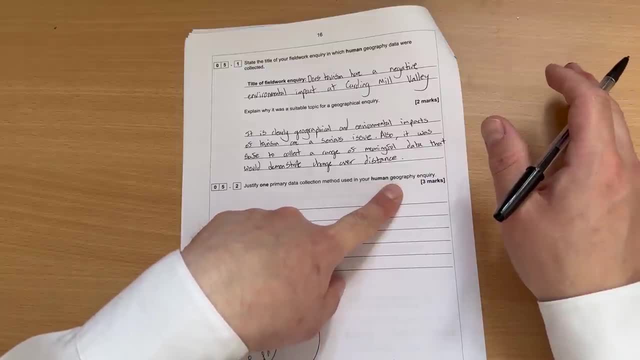 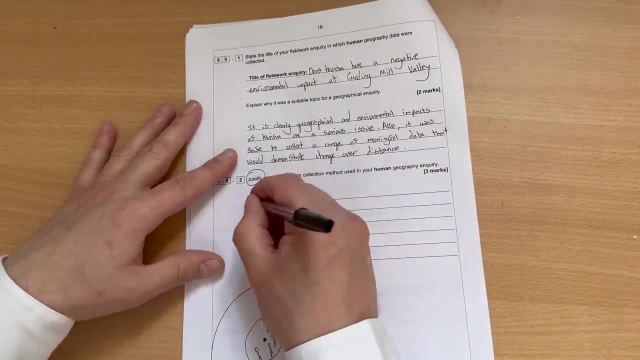 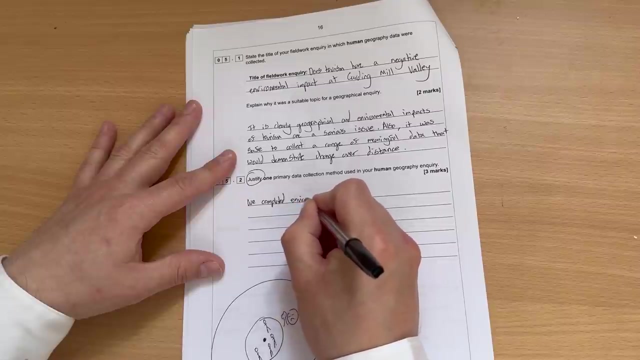 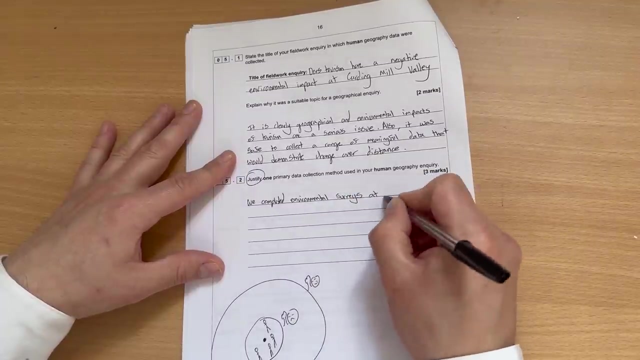 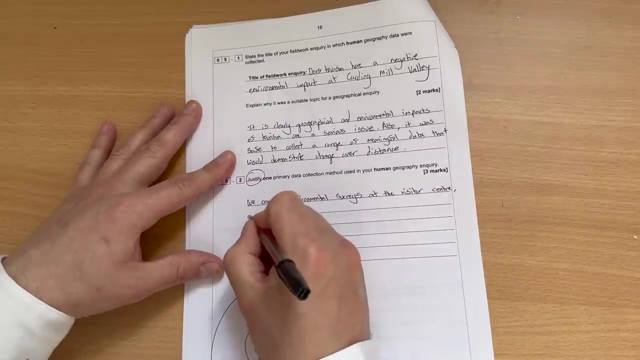 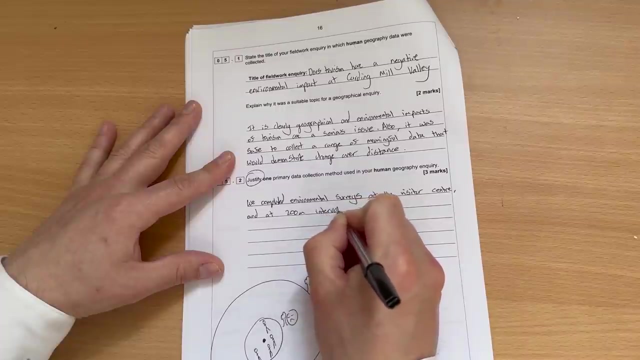 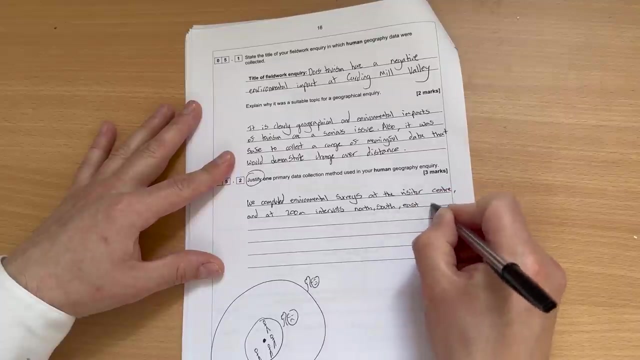 Data collection method used for your human geography inquiry. This is the command word here, So not just what you did, why you did it. So I would say we completed environmental surveys at the visitor centre And at 200 metre intervals- north, south, east and west. 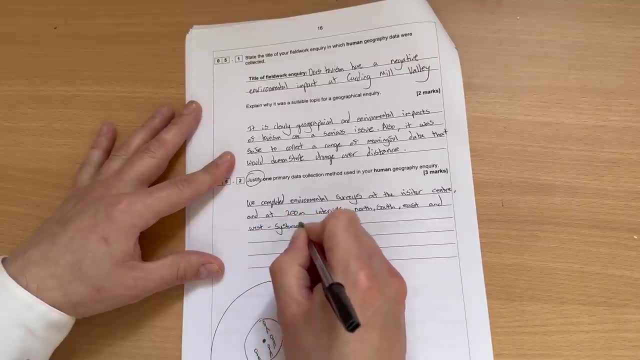 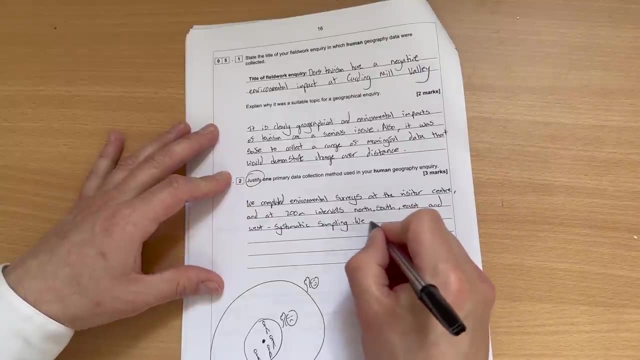 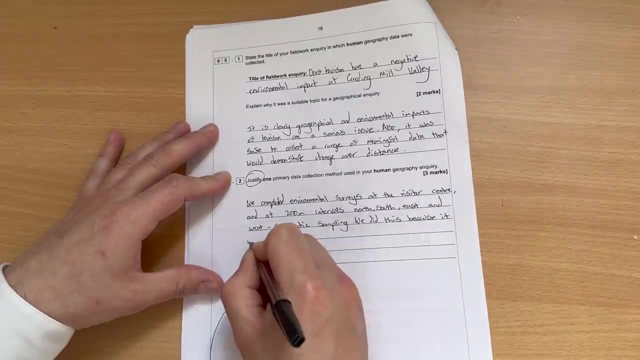 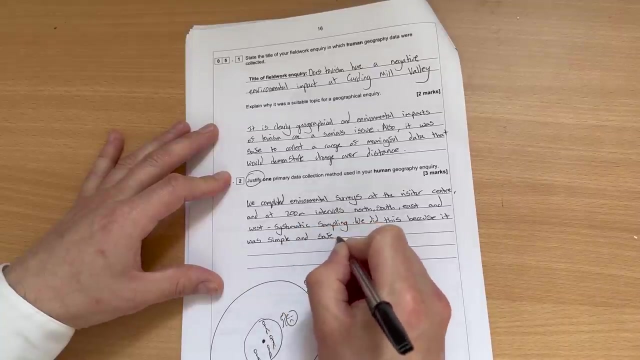 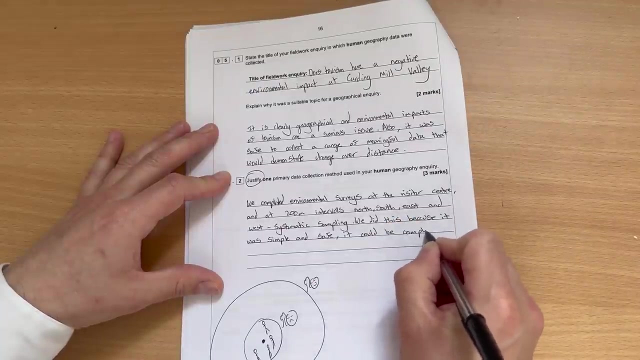 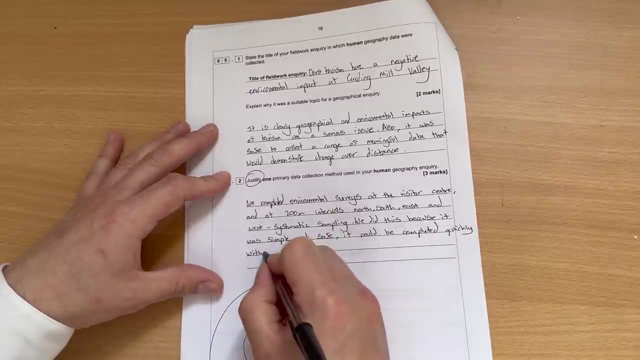 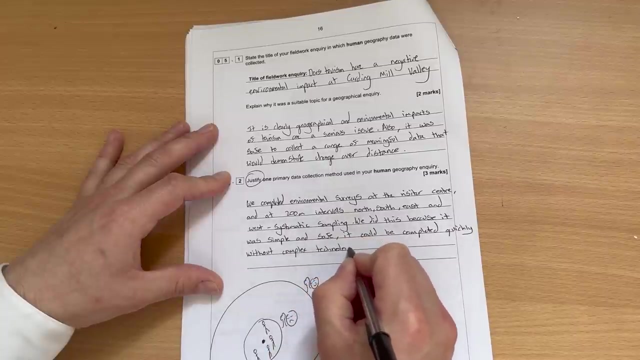 Okay, this is systematic sampling, But remember why have we done it? Justify We did this Because it was simple and safe comma. It could be completed quickly without complex Technology, And I think this is my new favourite phrase. 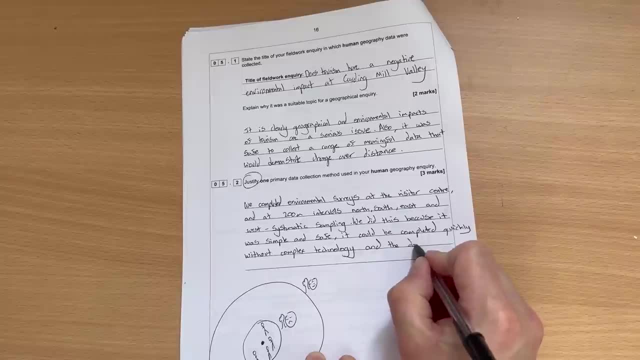 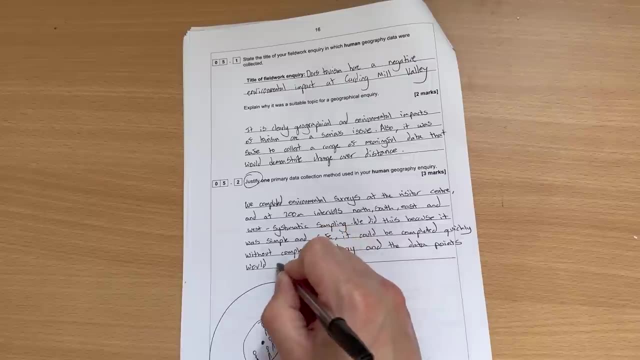 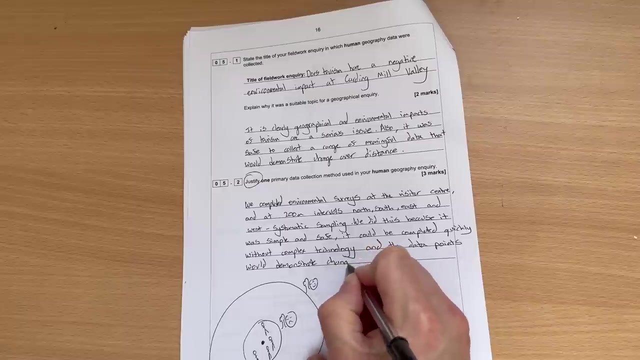 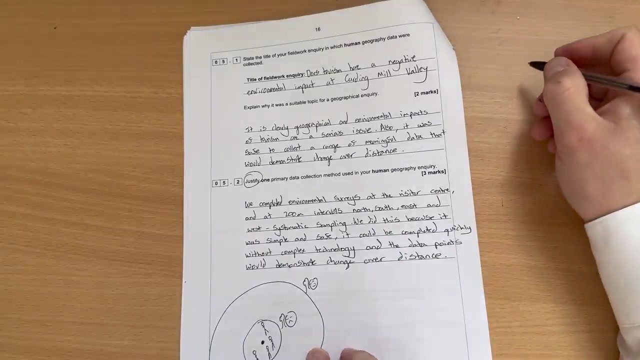 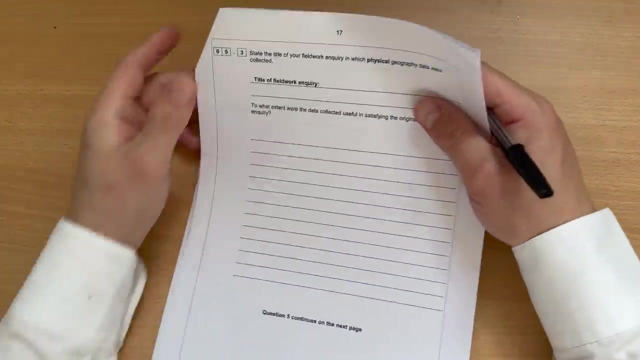 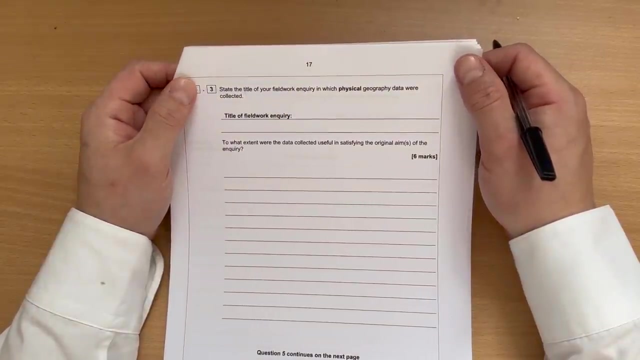 And the data points would show or would demonstrate change over distance. Okay, But if you just say what your data collection method is, you're probably going to get one mark Okie doke State the title of your fieldwork inquiry in which physical geography data were collected. 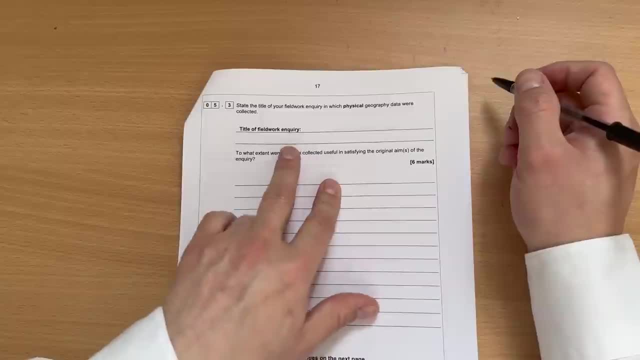 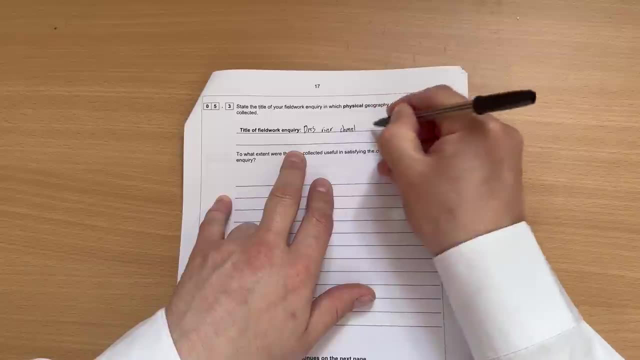 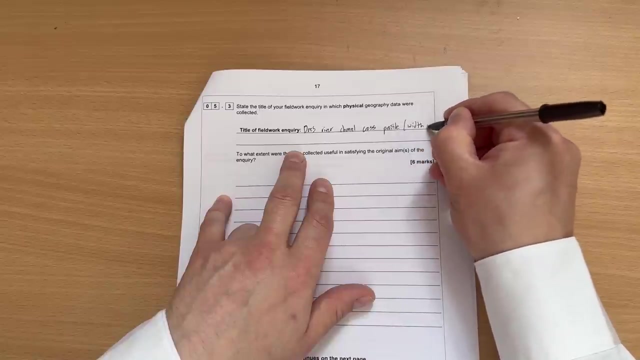 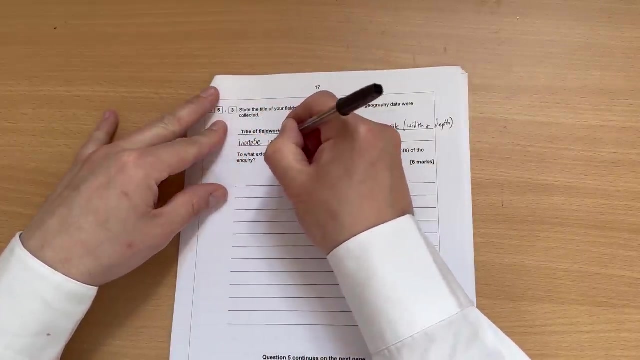 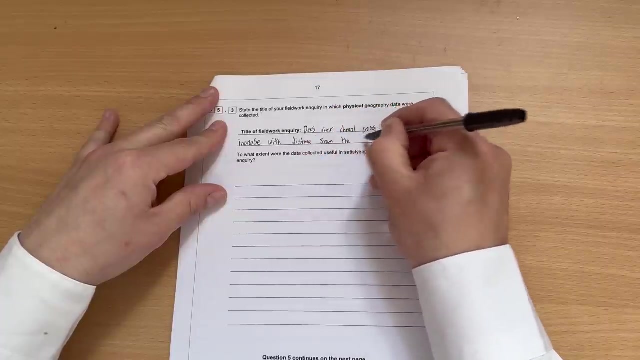 Title of inquiry. So we're doing the physical geography. Does river channel cross? Okay Profile? if you don't know what that means, width and depth Increase With Distance From the source, So let me just show you here quickly what we're saying is. 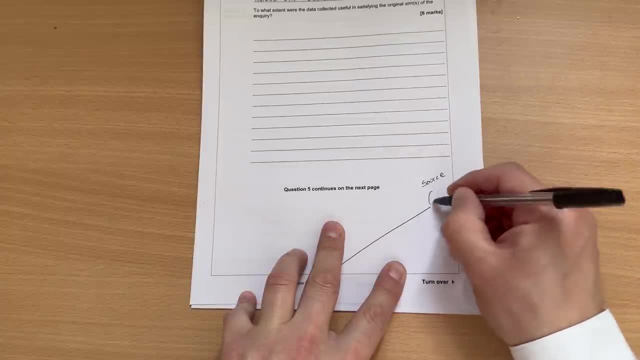 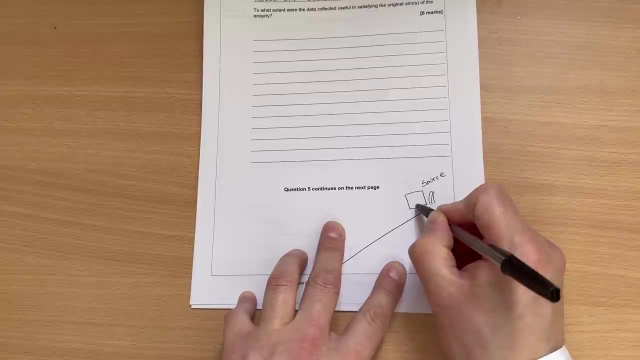 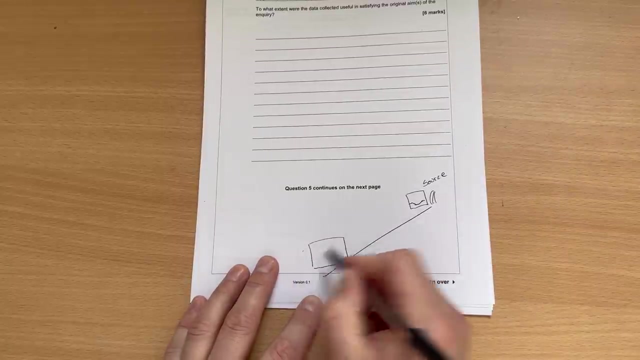 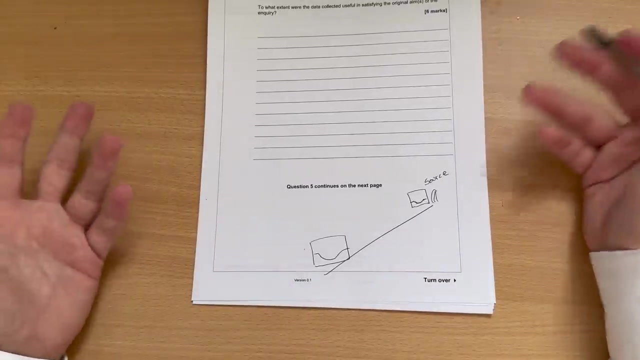 At the source or start the river further up. There was a waterfall. there The river is going to be Shallow And narrow, Whereas down here It's going to be deeper and wider. now, in reality, We only would, we only went down about two, three kilometers, so you're not going to see much difference. 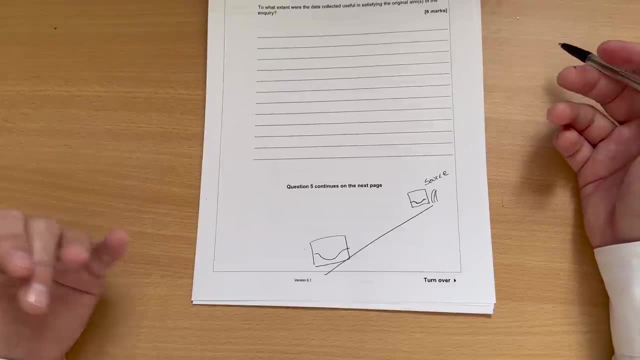 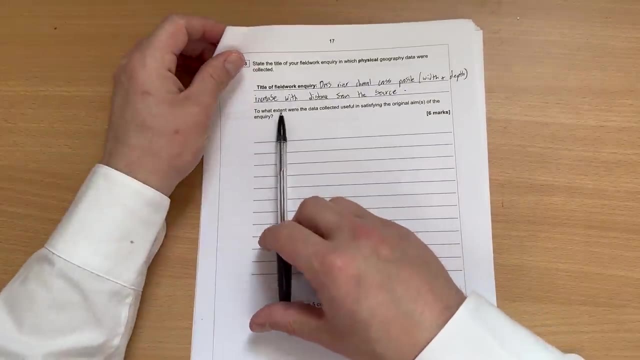 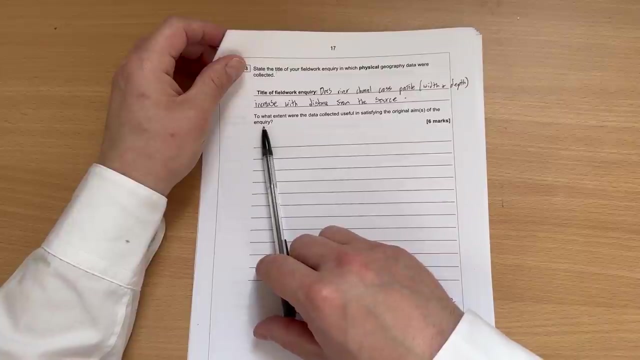 But that's the theory we're testing. Okay, that's the aim of it and That is what the Bradshaw model suggests. wider, deeper anyway, To what extent where the data collected useful in Satisfying the original aims of the inquiry, all right, so I 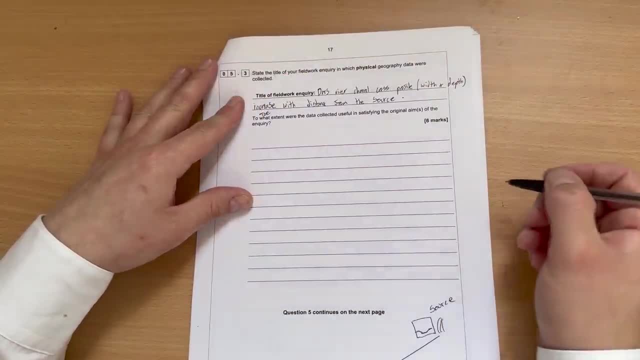 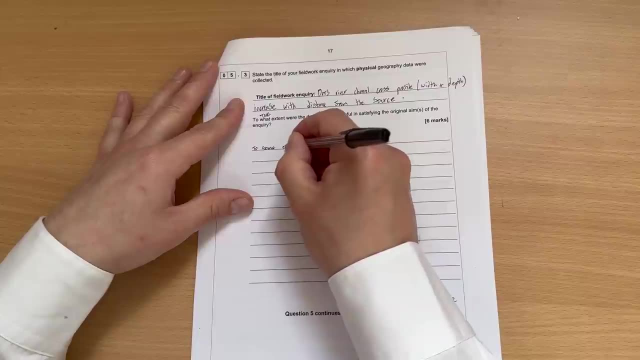 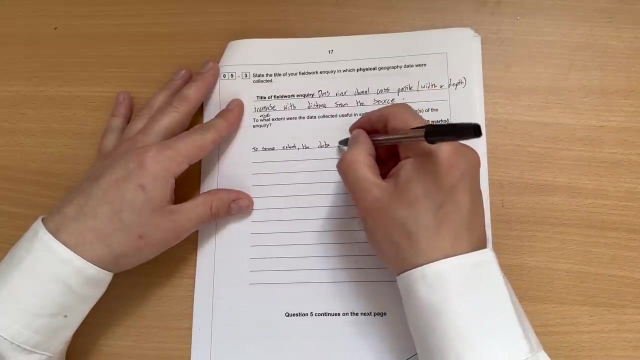 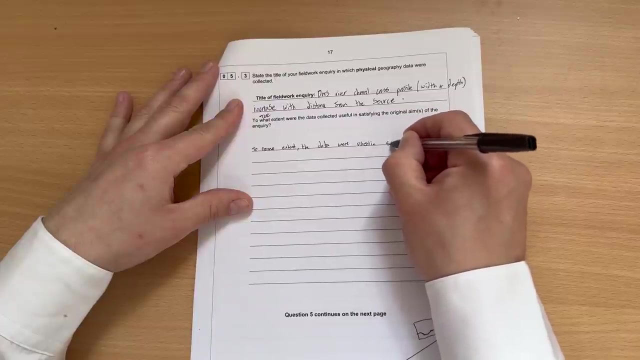 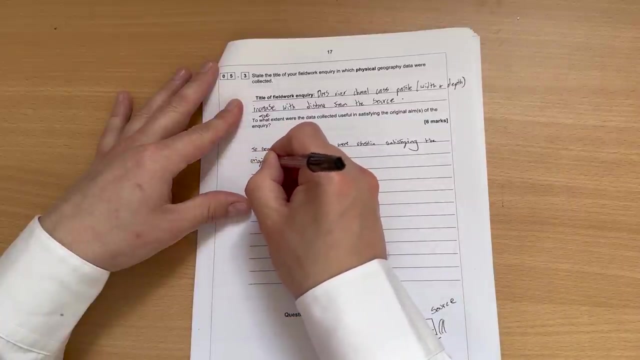 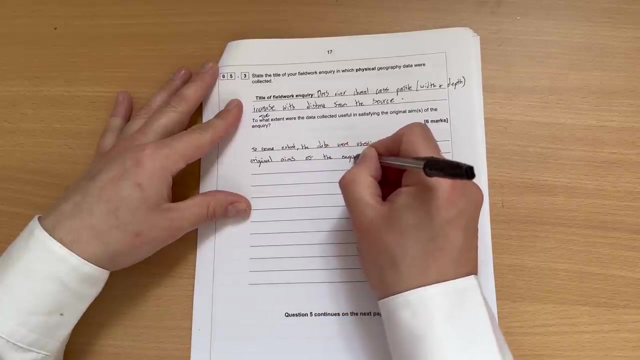 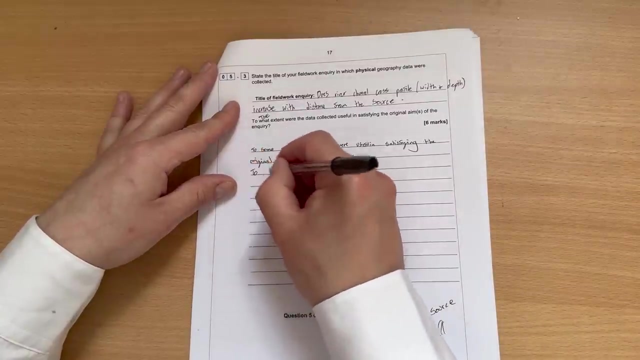 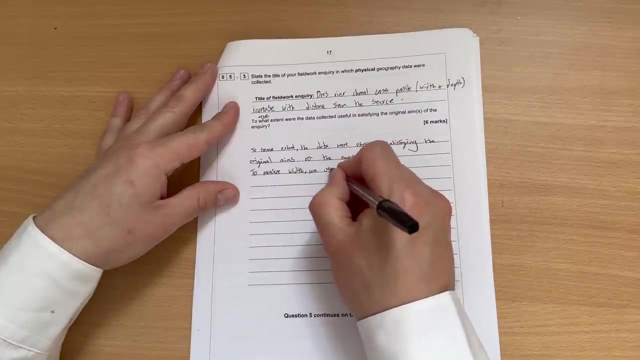 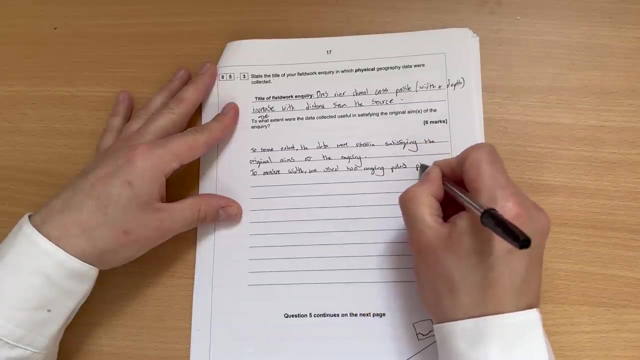 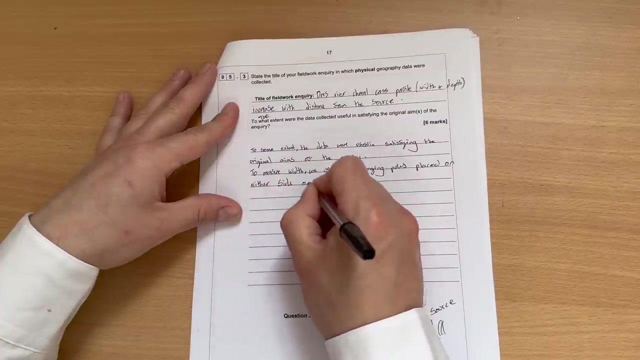 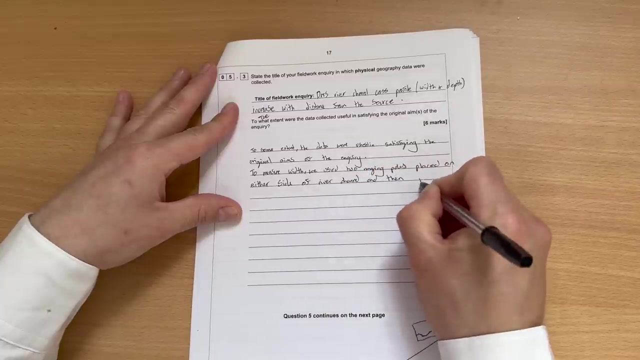 Would start off TSA To some extent. Comma. the data Were useful In satisfying The original Ames of the inquiry. Okay, that's the aims of the inquiry. so to measure width comma, we used two ranging poles placed on either side of river channel and then pulled. 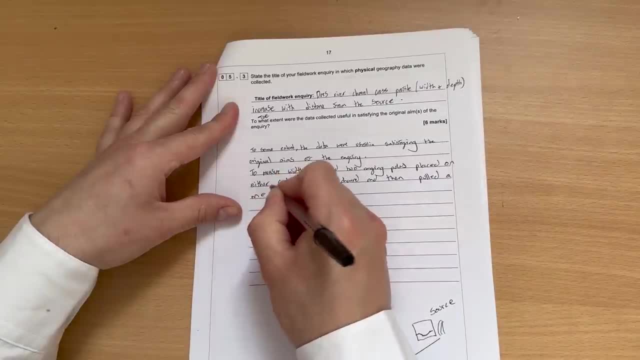 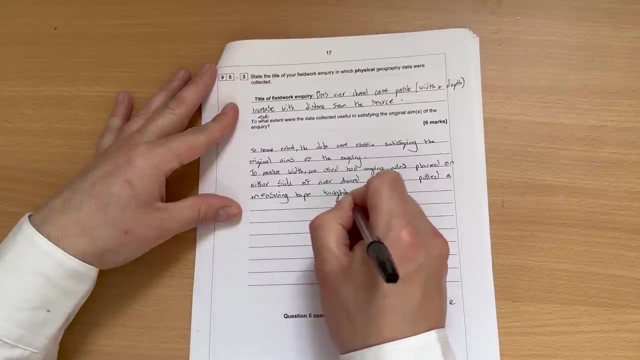 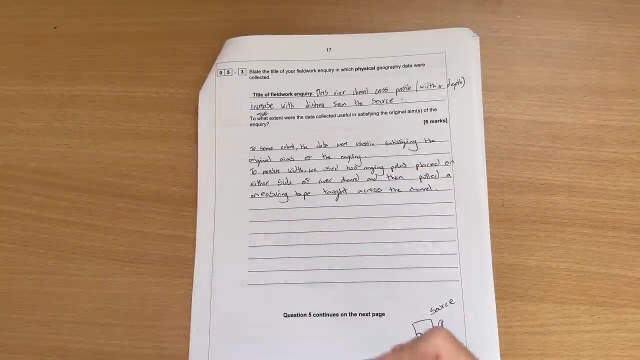 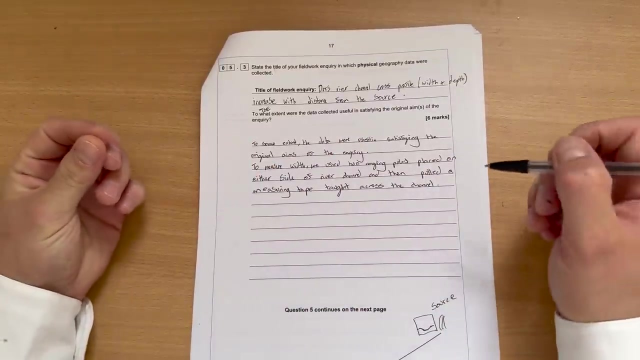 a measuring tape taught, which means tight across the channel. okay, now we've said what we did. how did that? it meet the aims. this is where you get the marks and this is where kids and I think some teachers don't- don't follow through. here we've got to say this. 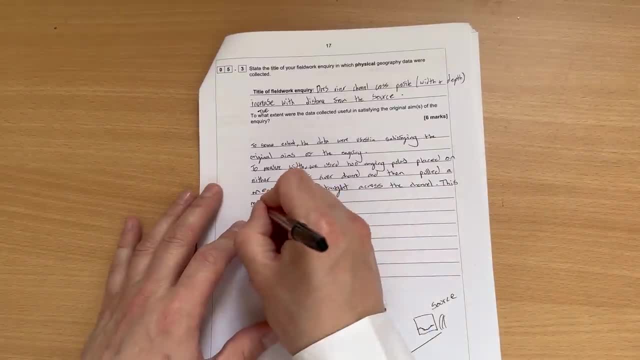 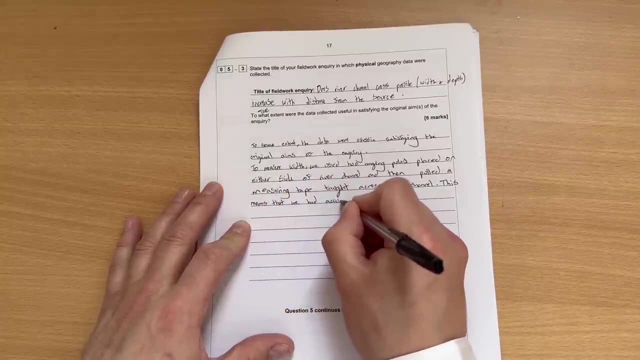 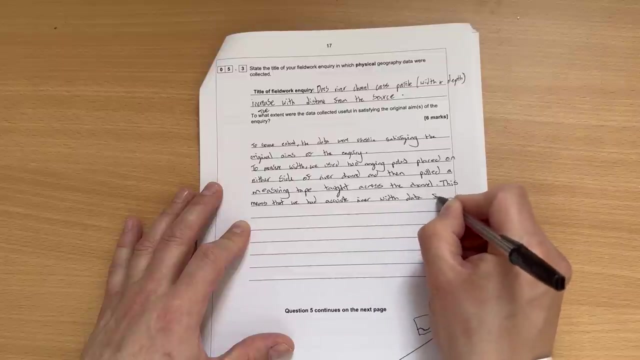 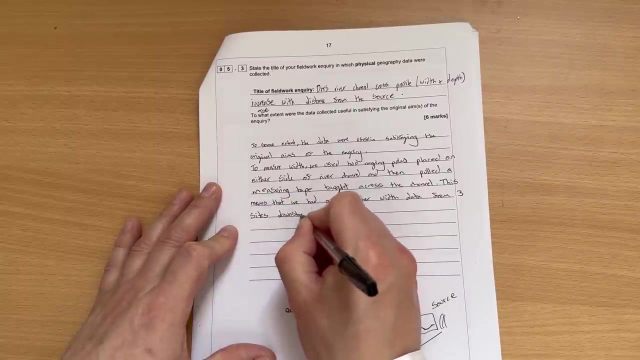 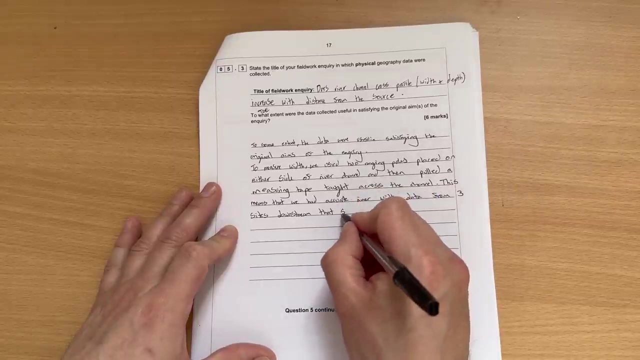 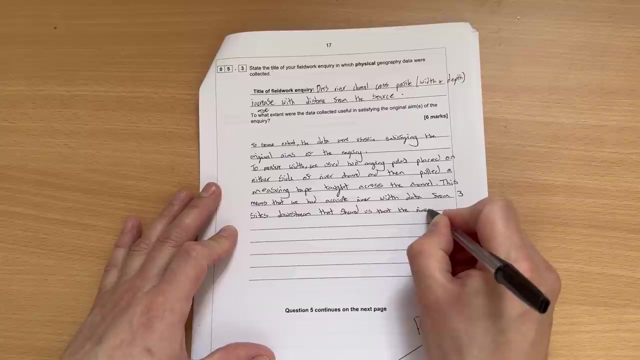 means that we had accurate river width data from three sites downstream. that means that we had accurate river width data from three sites downstream. that means that we had accurate river width data from three sites downstream that showed us that the river channel did. showed us that the river channel did. 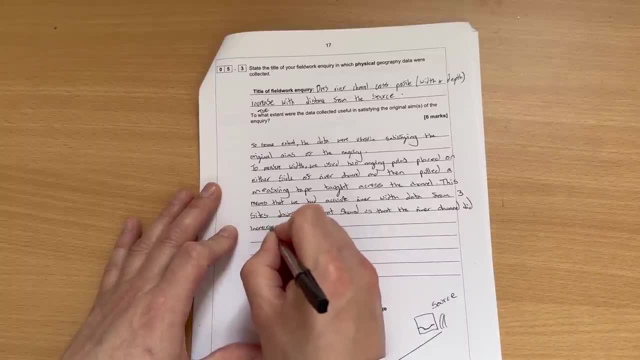 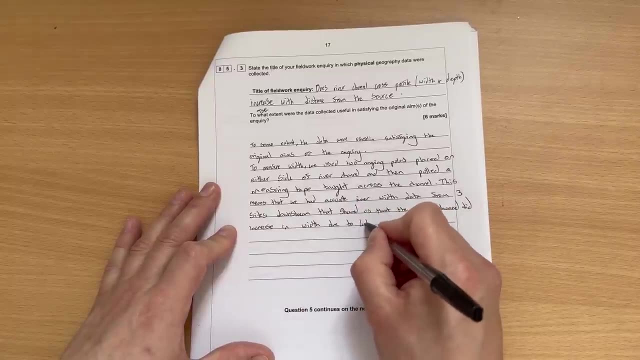 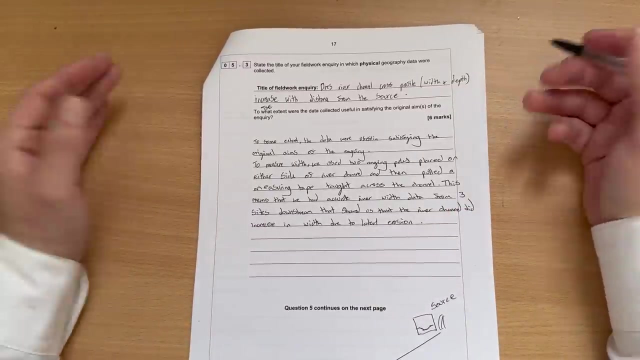 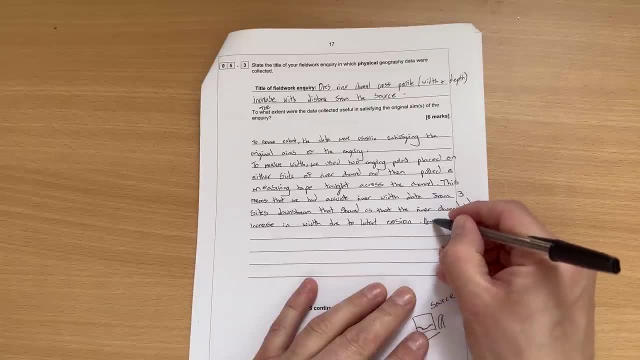 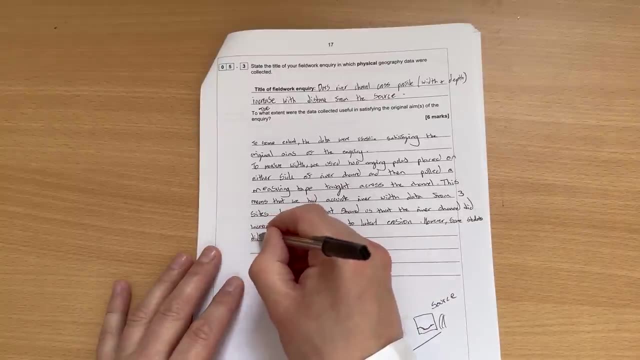 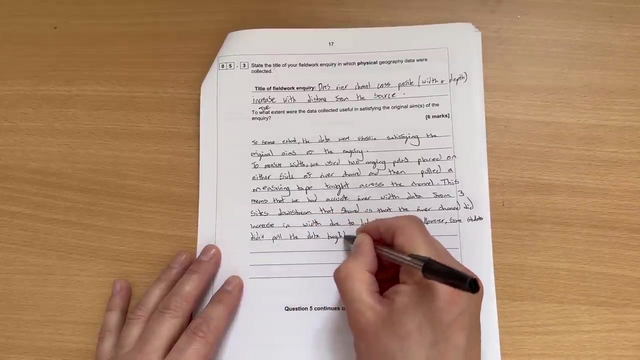 to what extent was it useful? you could talk to what extent was it useful. you could talk about the problems here just briefly, about the problems here, just briefly about the problems here, just briefly. however, some students didn't pull the. however, some students didn't pull the. however, some students didn't pull the data taught. pull the data taught, the. 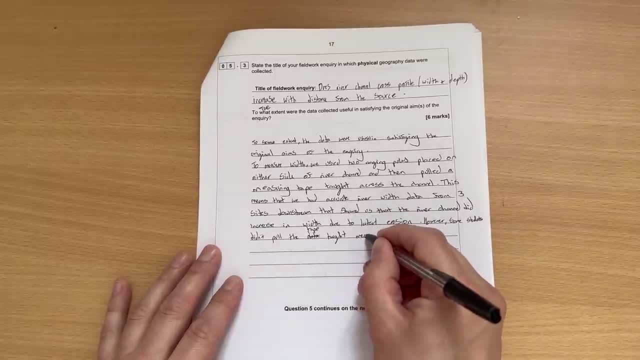 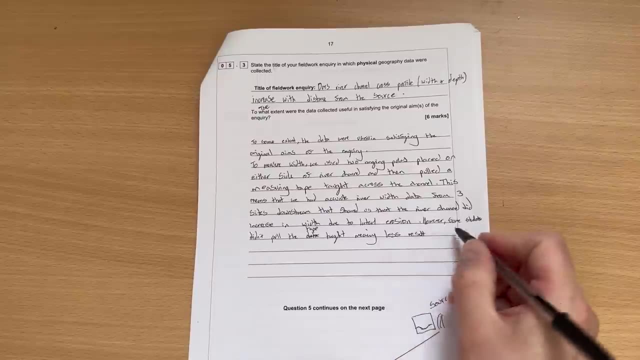 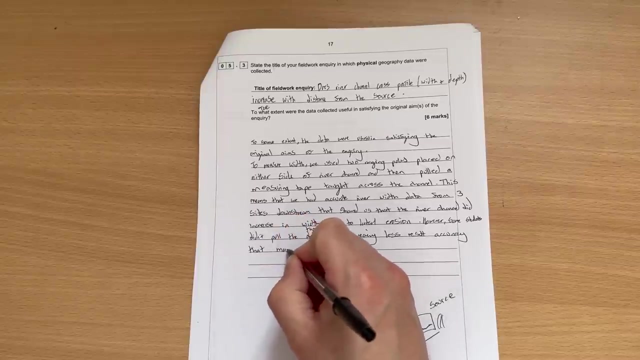 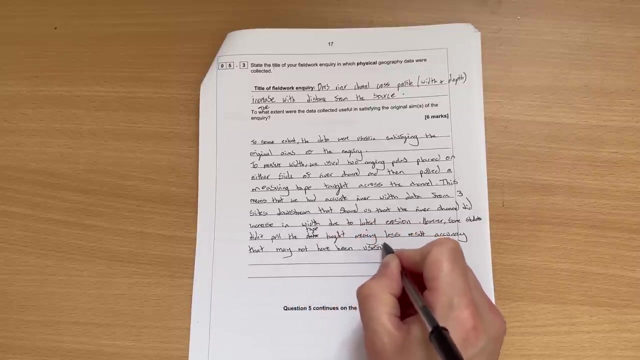 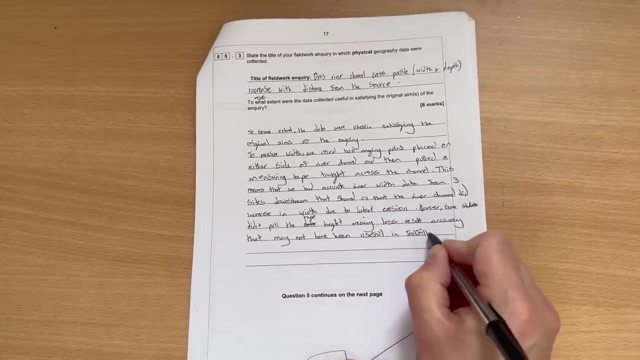 data taught. pull the data taught the data taught. pull the data taught the tape taught meaning less result. tape taught meaning less result. tape taught meaning less result possible. accuracy that may not being possible. accuracy that may not being possible. accuracy that may not being useful in fulfilling our aims of the 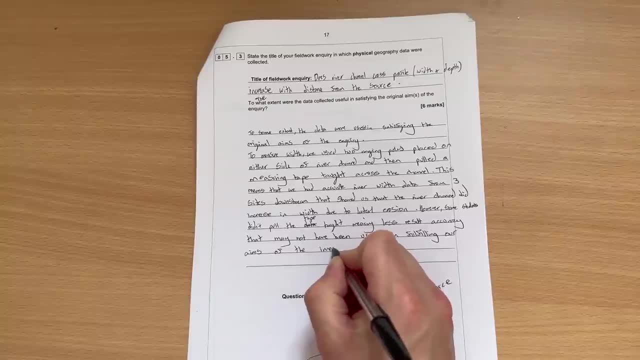 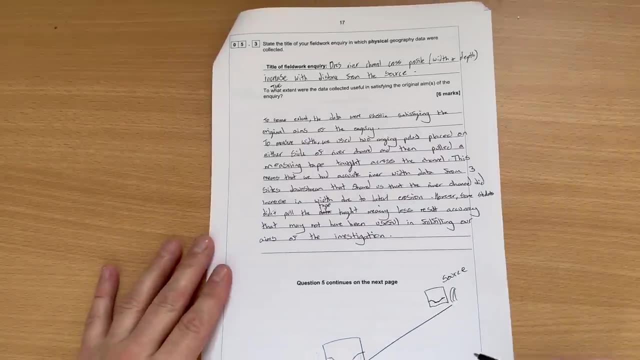 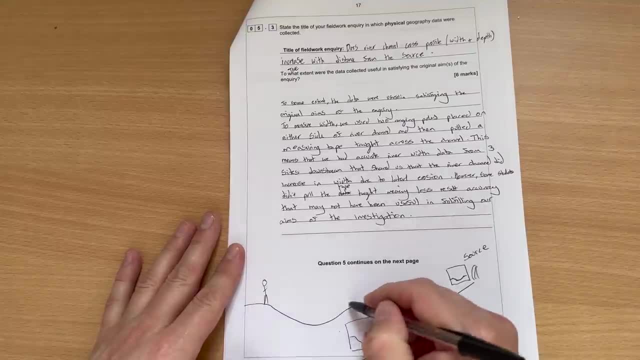 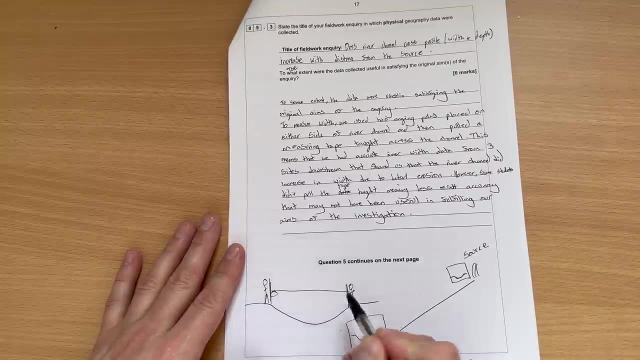 all right. the other thing we did, if you remember, is once we've got the river channel with area of our ranging poles, we pulled a tape channel with area of our ranging poles. we pulled a tape channel with area of our ranging poles. we pulled a tape measure across. in way we 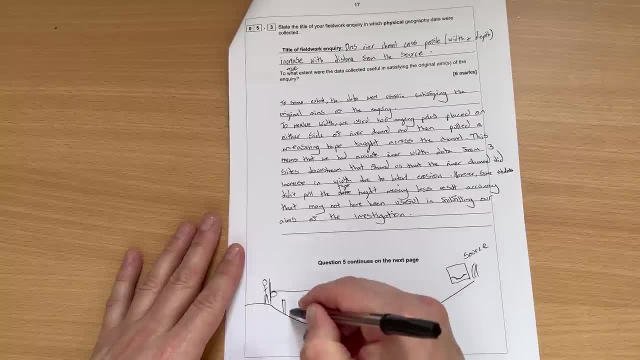 measure across in way, we measure across in way. we divided that distance by 10, and then we used a meter divided that distance by 10, and then we used a meter divided that distance by 10, and then we used a meter ruler at every tenth of the. 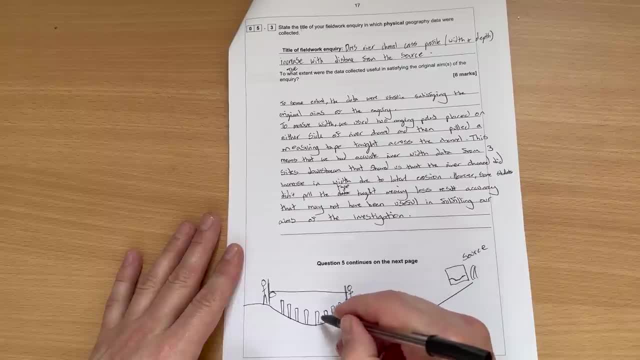 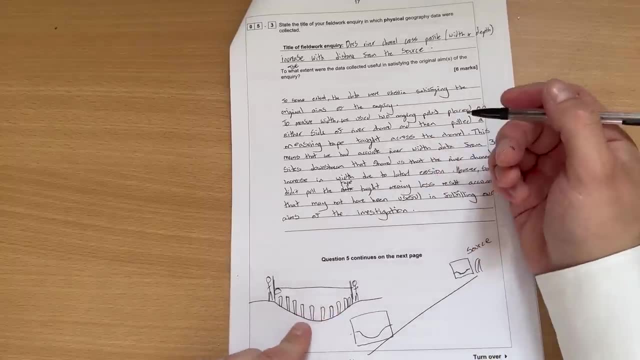 ruler, at every tenth of the ruler, at every tenth of the river, to measure, every 10th to show us depth. so then, what? every 10th to show us depth? so then, what? every 10th to show us depth. so then, what you would do is you would say: I'm running. 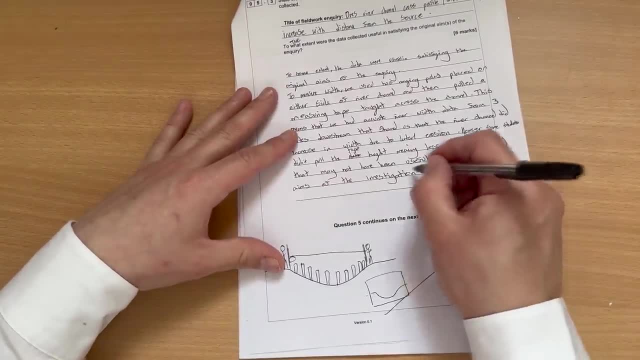 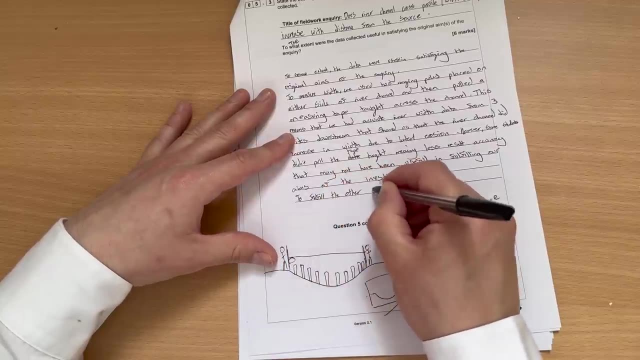 you would do is you would say I'm running. you would do is you would say I'm running out of space, but to fulfill the out of space, but to fulfill the out of space, but to fulfill the other aim, which was depth comma, and other aim which was depth comma, and 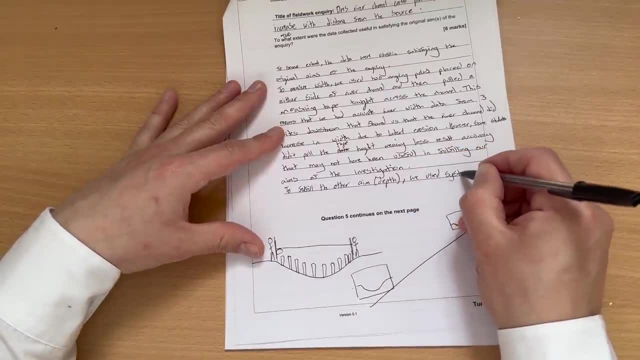 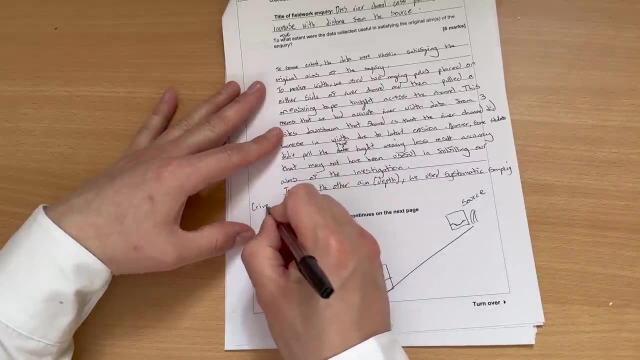 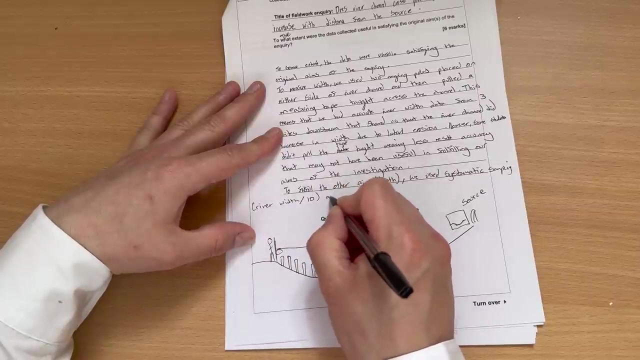 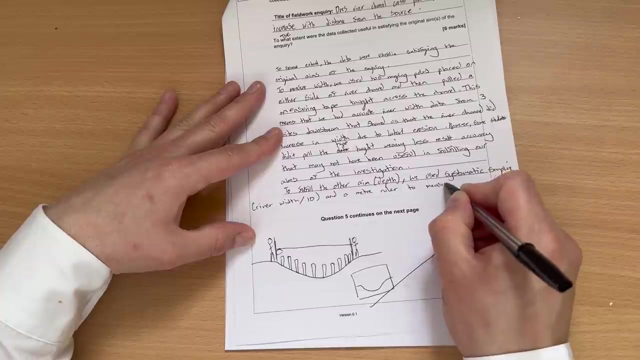 other aim, which was depth comma, and we used systematic sampling and start. we used systematic sampling and start. we used systematic sampling and start right now, right now, right now. river width divided by 10 and a meter. river width divided by 10 and a meter. river width divided by 10 and a meter. ruler to measure depth across channel. 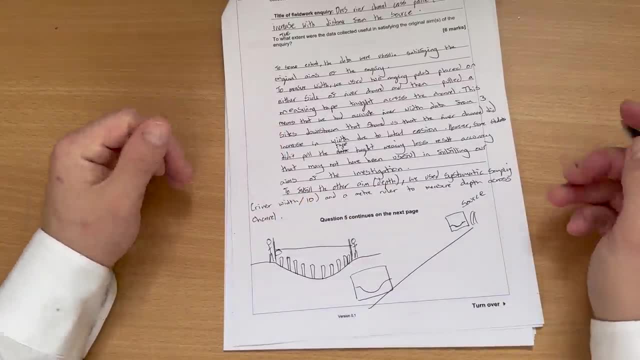 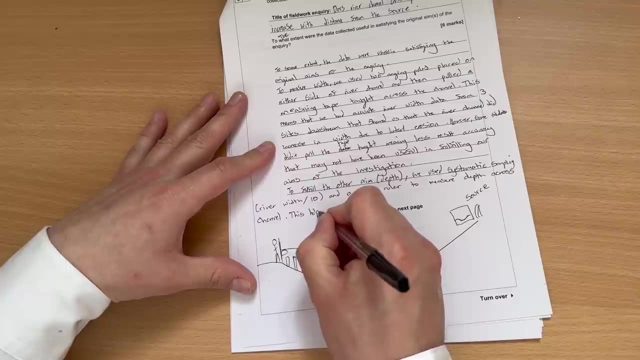 ruler to measure depth across channel. ruler to measure depth across channel. all right, did this help with the aims? all right, did this help with the aims? all right, did this help with the aims? yes, it did. this helped meet the original. yes, it did. this helped meet the original. 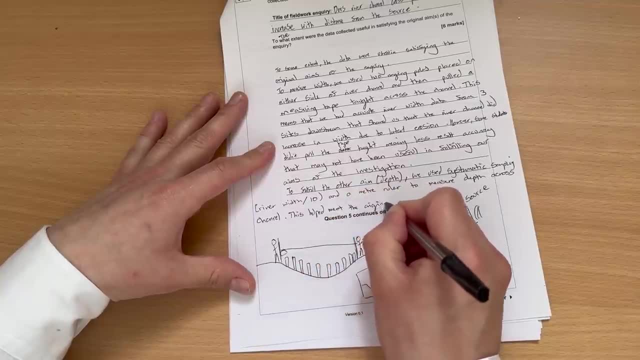 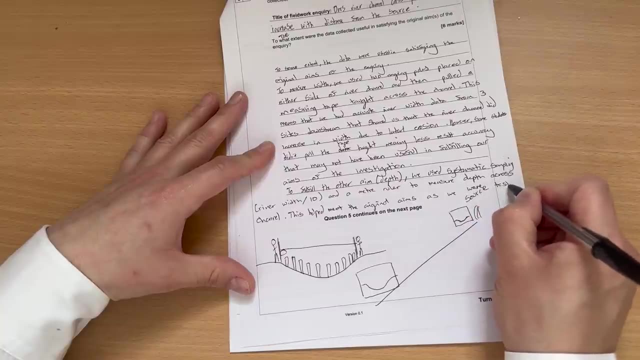 yes, it did. this helped meet the original aims as we were testing. they come down aims as we were testing. they come down aims as we were testing. they come down here a bit: whether could bring the here a bit. whether could bring the here a bit, whether could bring the Bradshaw modeling, whether the Bradshaw 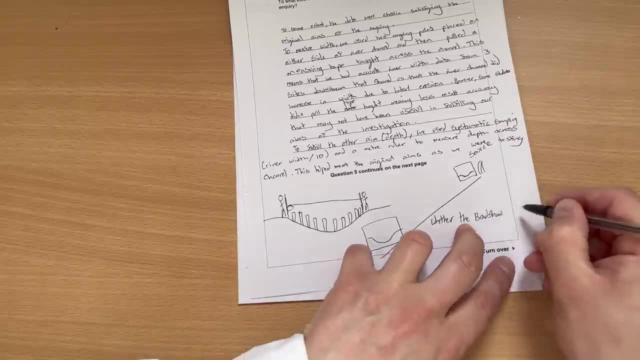 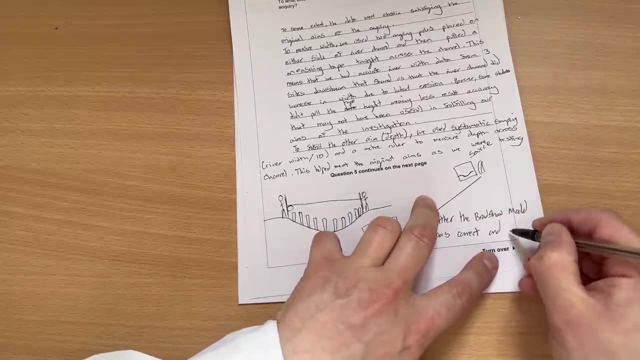 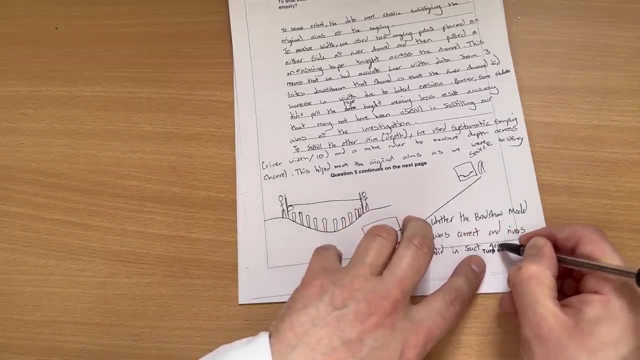 Bradshaw modeling, whether the Bradshaw Bradshaw modeling, whether the Bradshaw model model Bradshaw modeling, whether the Bradshaw model was correct and rivers did in fact was correct and rivers did in fact was correct and rivers did in fact get wider downstream. if you've got time, you. 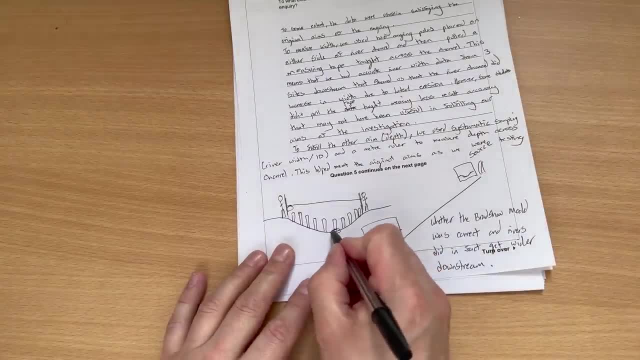 get wider downstream if you've got time. you get wider downstream. if you've got time, you can talk about the problems. you know can talk about the problems. you know can talk about the problems. you know some kids might put it on a rock we. some kids might put it on a rock, we. 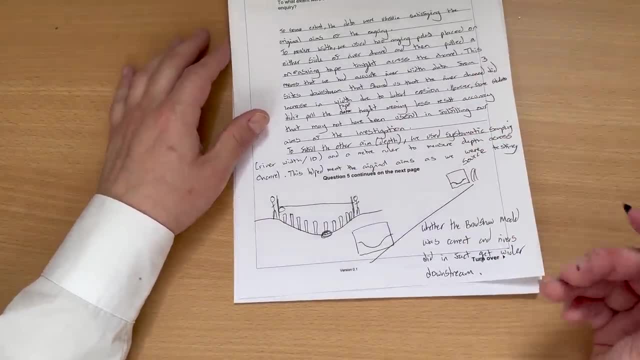 some kids might put it on a rock. we could have gotten better data by using a. could have gotten better data by using a. could have gotten better data by using a laser range finder, but good luck getting laser range finder. but good luck getting laser range finder, but good luck getting the school to pay for about two grams. 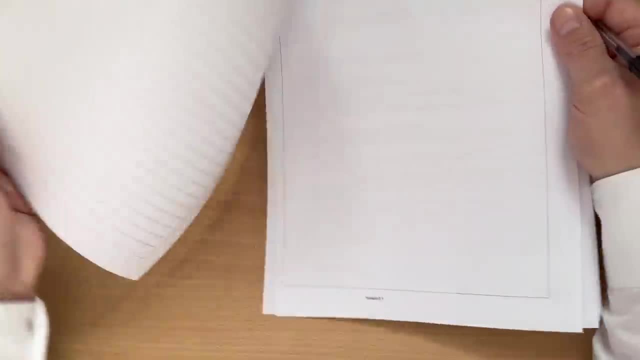 the school to pay for about two grams. the school to pay for about two grams worth of them. it's not appropriate, all worth of them. it's not appropriate, all worth of them. it's not appropriate all right final one of a 12 marker with right final one of a 12 marker with. 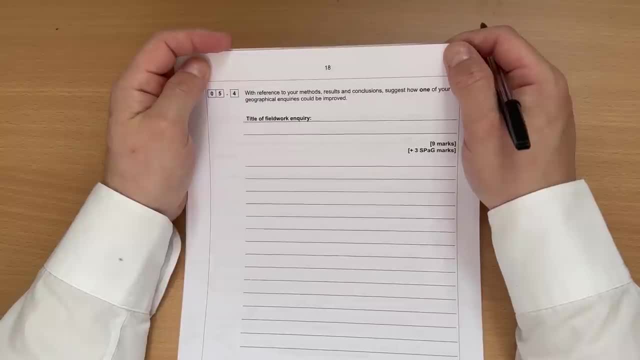 right final one of a 12 marker with reference to your method results and reference to your method results and reference to your method results and conclusions suggest that one of your conclusions suggest that one of your conclusions suggest that one of your geographical inquiries could be improved. geographical inquiries could be improved. 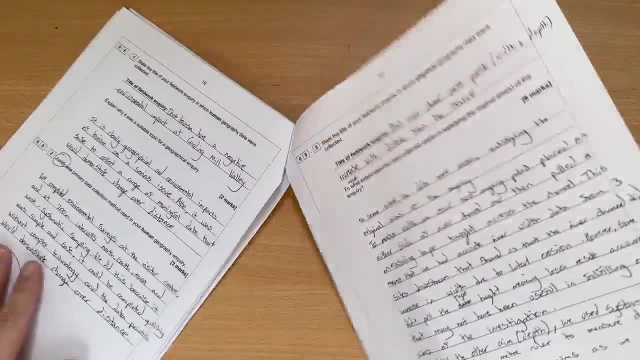 geographical inquiries could be improved. all right, this is a nice question. it all right. this is a nice question, it all right. this is a nice question. it doesn't confuse matters by saying the doesn't confuse matters by saying the doesn't confuse matters by saying the original aims of the thing. and now I've original aims of the thing, and now I've original aims of the thing, and now I've already talked about rivers, quite a lot already talked about rivers, quite a lot already talked about rivers, quite a lot. so I'm going to do this on the human. so I'm going to do this on the human. 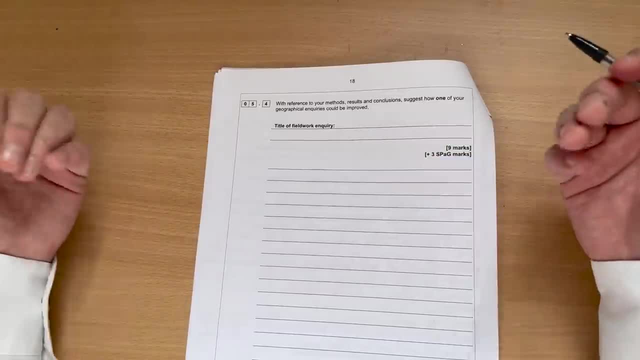 so I'm going to do this on the human geography, but you could do it on the geography, but you could do it on the geography, but you could do it on the rivers, basically what we've just said in rivers, basically what we've just said in rivers, basically what we've just said in the last answer to an extent. so title: 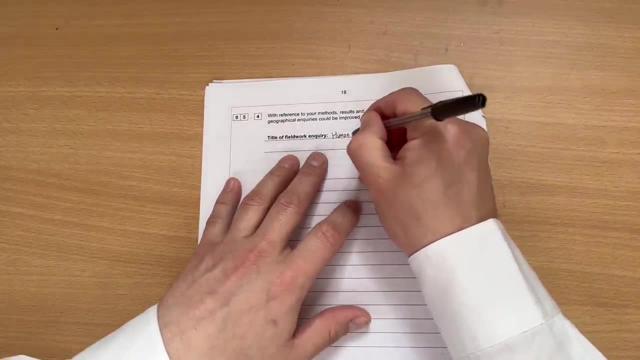 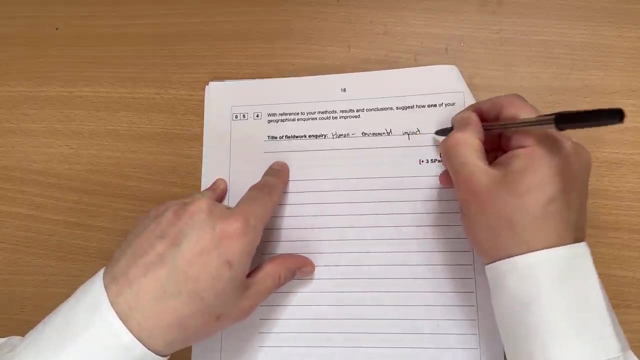 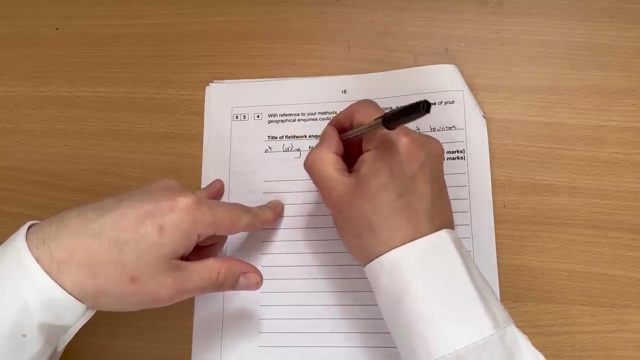 the last answer to an extent. so title: the last answer to an extent so title. so I'm going to put human environmental. so I'm going to put human environmental, so I'm going to put human environmental. impact tourism at Cardin male Valley- okay. impact tourism at Cardin male Valley- okay. 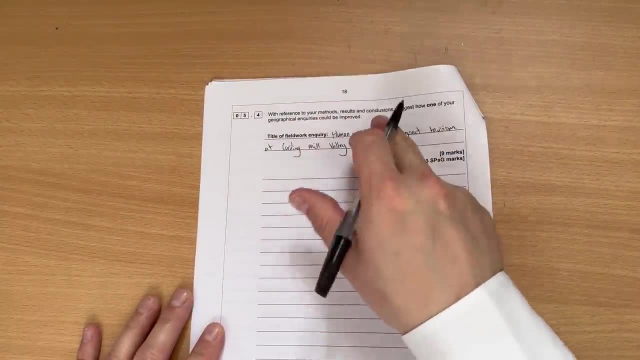 impact tourism at Cardin male Valley. okay now, whenever you see these three linked now, whenever you see these three linked now, whenever you see these three linked: methods results conclusions. I've done methods results conclusions. I've done methods results conclusions. I've done this with you loads of times. you could. 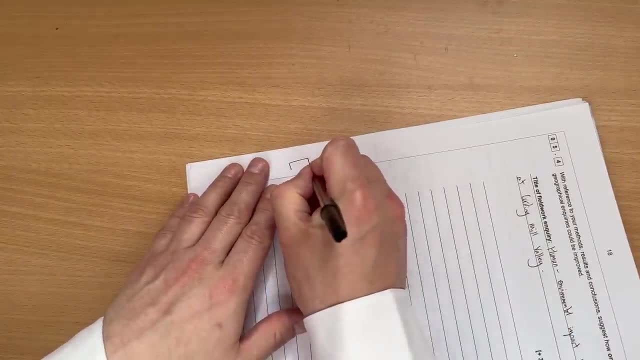 this with you loads of times. you could this with you loads of times. you could do it. you could do it at the side. do it, you could do it at the side. do it, you could do it at the side. remember it goes in a flowchart- methods. 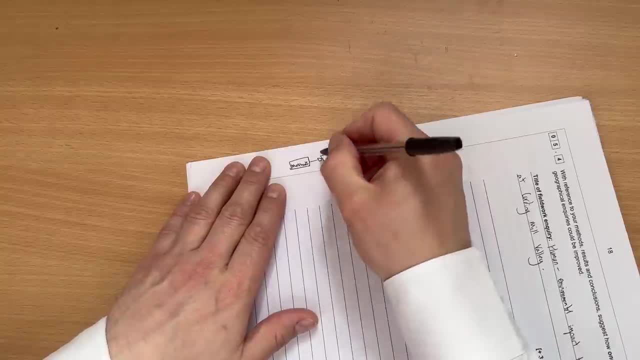 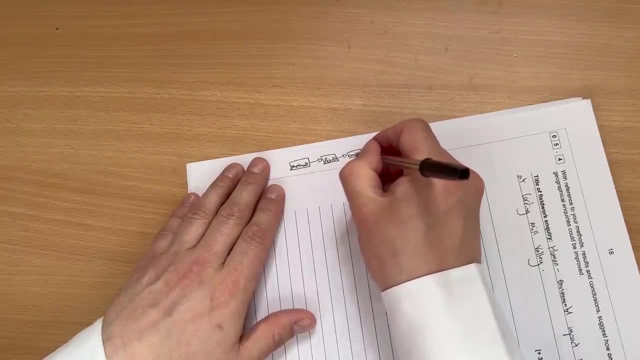 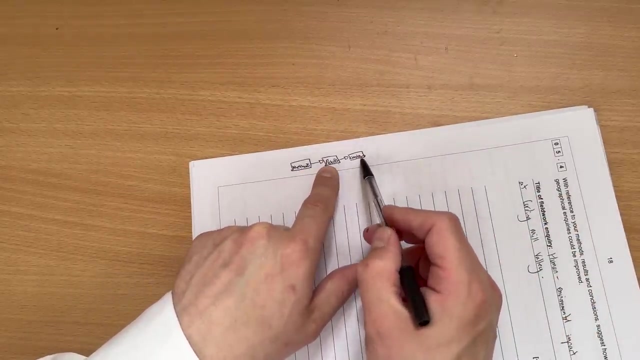 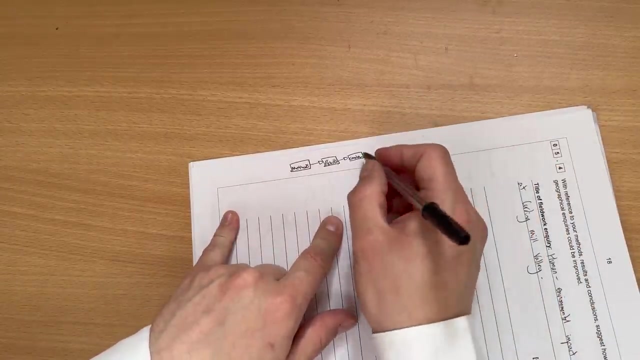 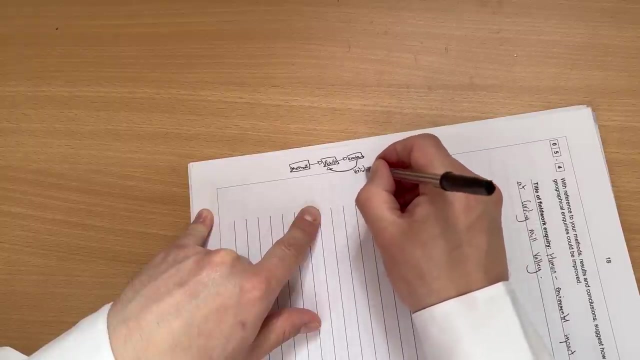 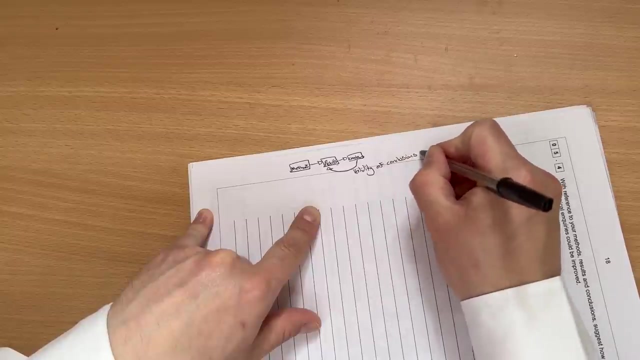 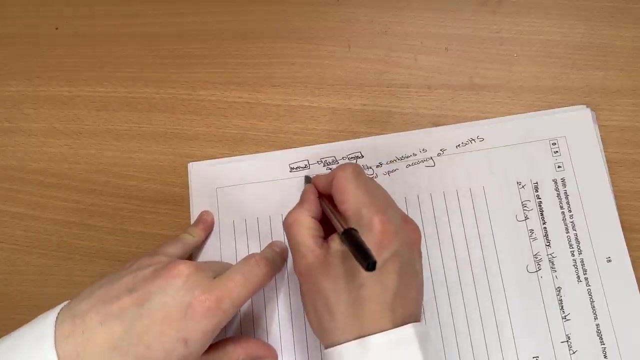 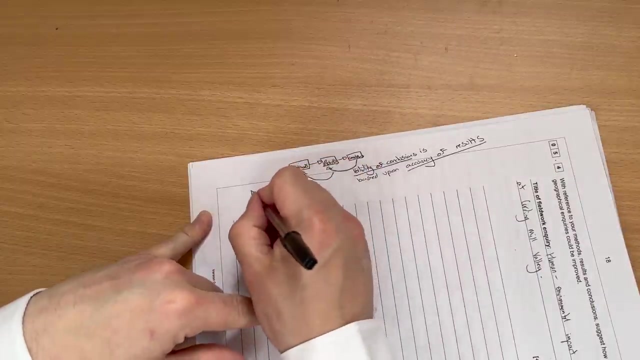 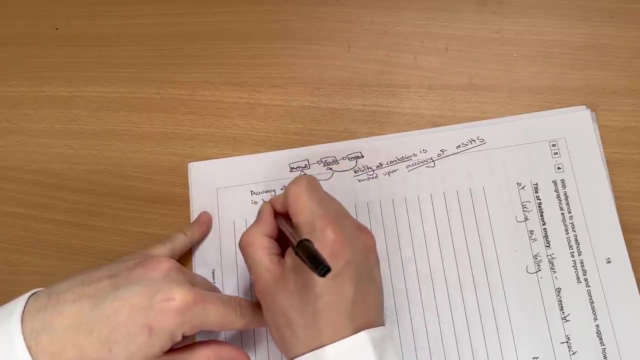 remember it goes in a flowchart methods. remember it goes in a flowchart methods to, to, to of conclusions is based upon: accuracy of conclusions is based upon. accuracy of conclusions is based upon accuracy of results. so keywords, accuracy of results. so keywords, accuracy of results. so keywords, accuracy of results is based upon valid now. 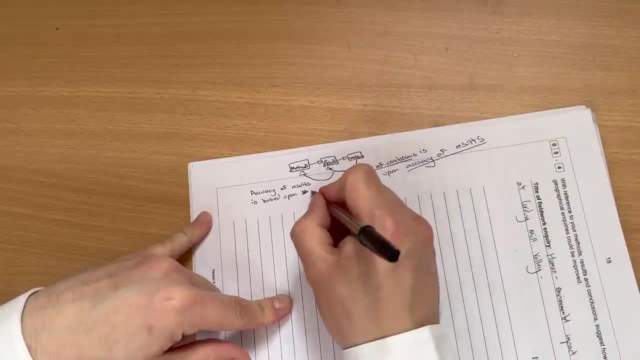 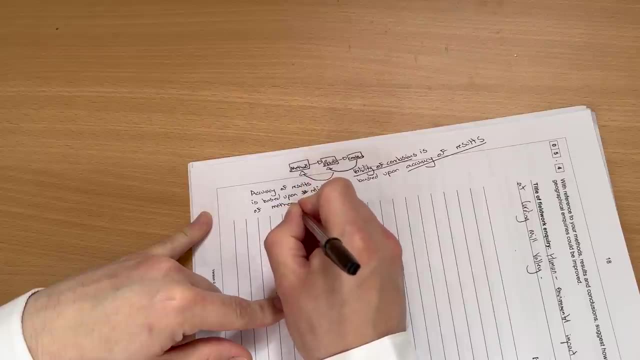 of results is based upon valid now of results is based upon valid now. accuracy was based upon the reliability. accuracy was based upon the reliability. accuracy was based upon the reliability of methods. so if your methods are of methods, so if your methods are of methods, so if your methods are unreliable, your accuracy of results is. 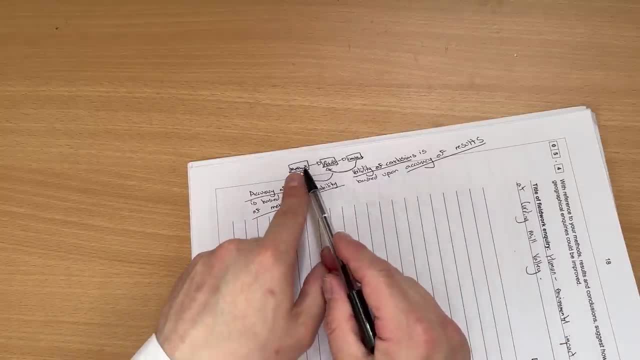 unreliable. your accuracy of results is unreliable. your accuracy of results is going to be lower, and that's what we do: going to be lower, and that's what we do: going to be lower, and that's what we do. so, if we want to improve our results, we 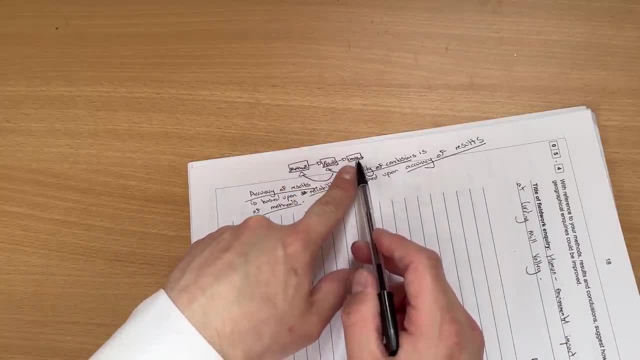 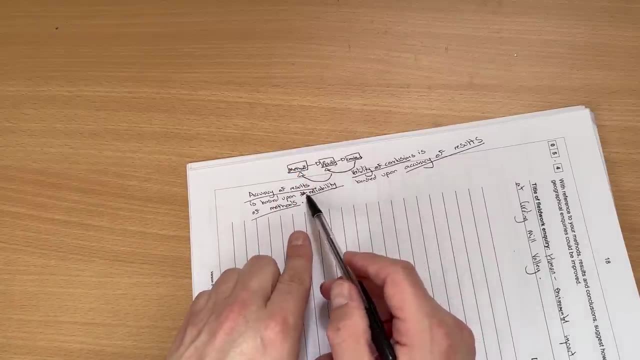 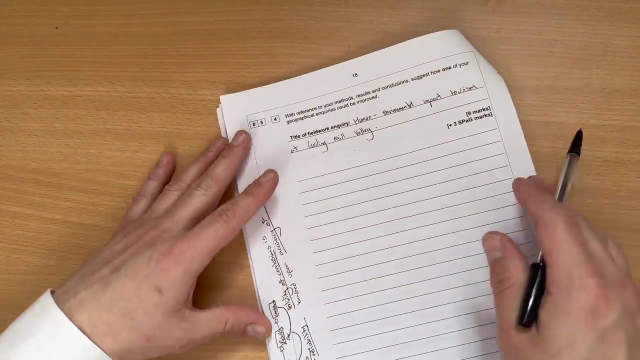 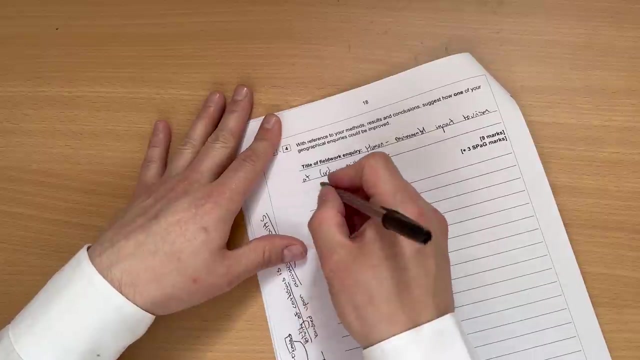 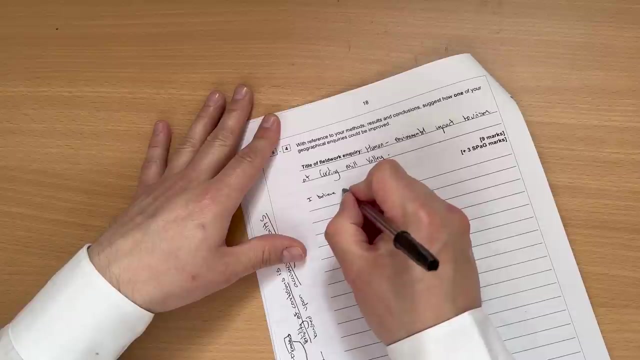 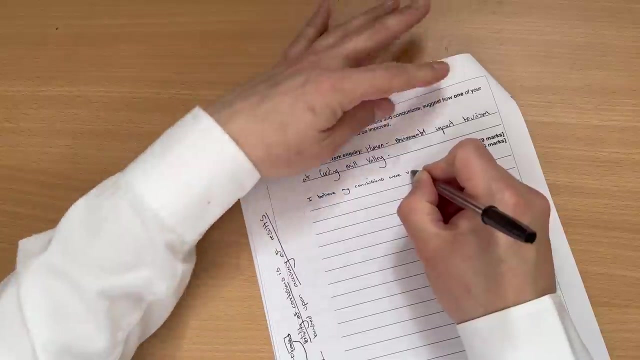 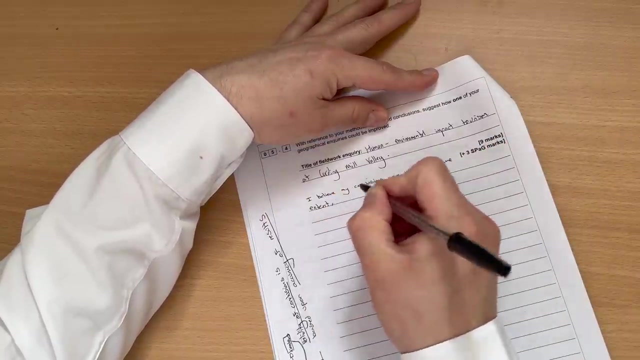 so if we want to improve our results, we make the methods more accurate. if we want to improve our conclusions, we have to make the results more accurate. we need the methods more reliable. all right. so reliability, accuracy, trustworthiness, validity. so times it wrong. the smash said 10 minutes. I believe my conclusions were valid to some extent, comma. however, 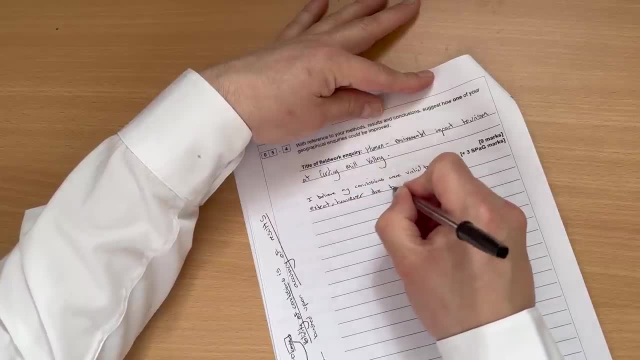 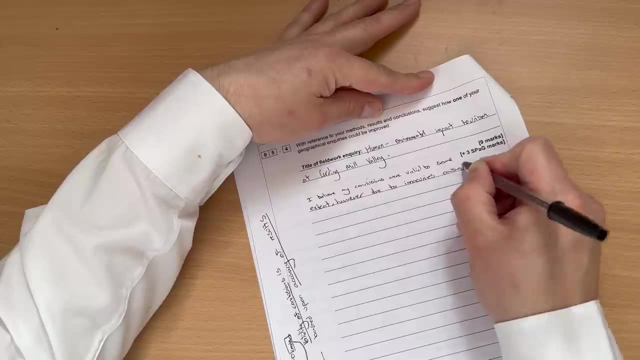 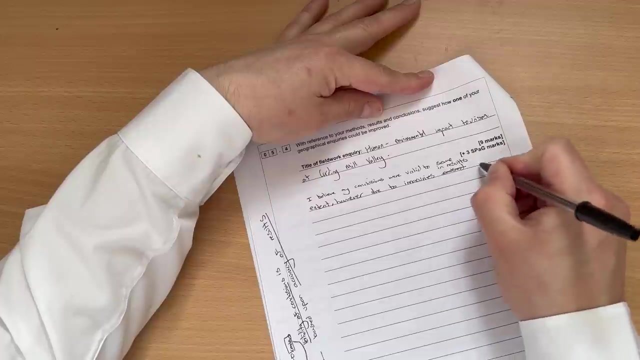 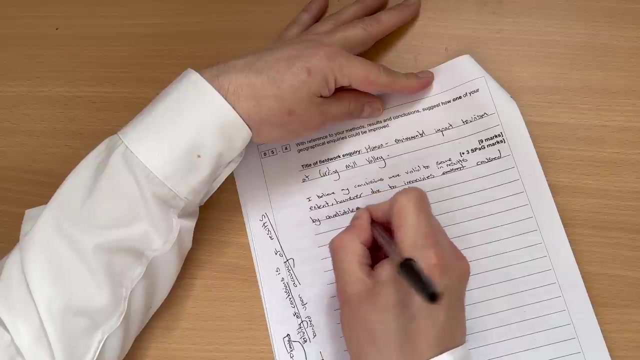 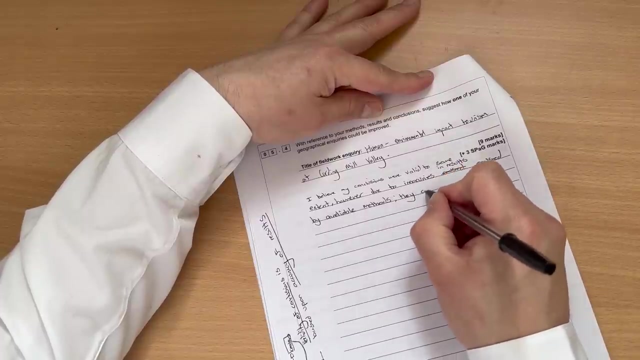 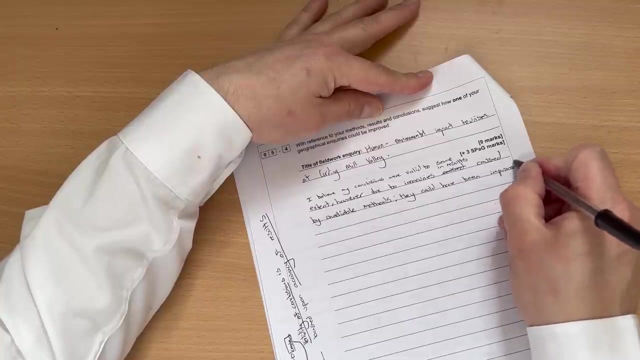 do you in accuracies caused, in accuracies in results caused by unreliable methods, semi-colon? they could have been improved. so what you've done there is: you've showed the examiner you understand this kind of cycle, this flow chart. right, we're going to set the scene a little bit. 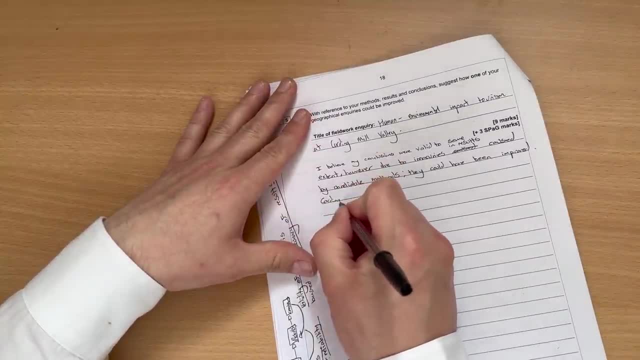 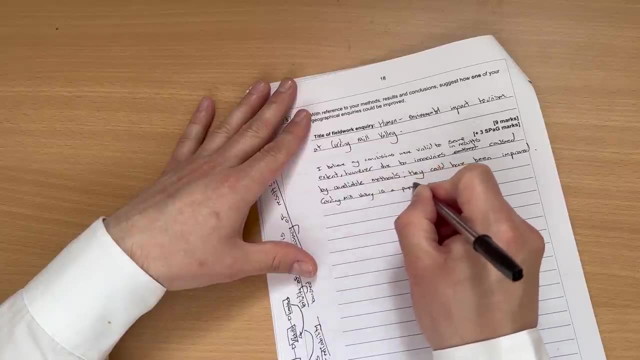 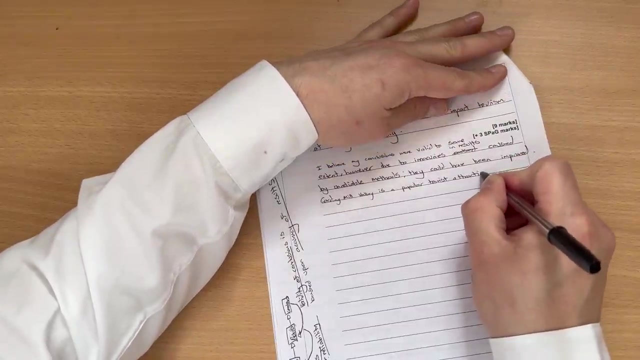 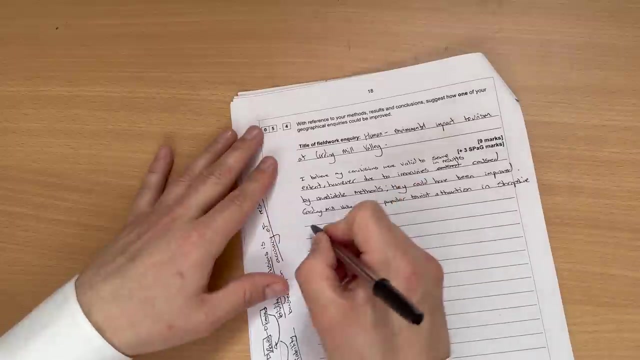 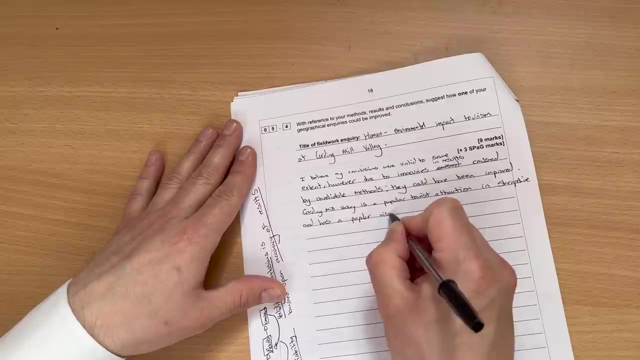 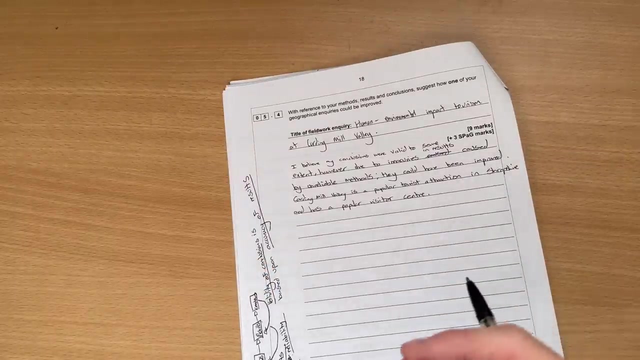 so Carding Mel Valley is a popular tourist attraction in Shropshire or Church Stretton in Shropshire and has a popular visitor centre. you can remember the Butler model talks about how tourism impacts an area, so you could bring that in the Butler model. 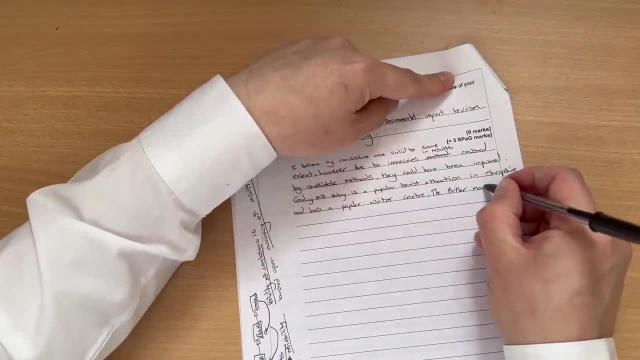 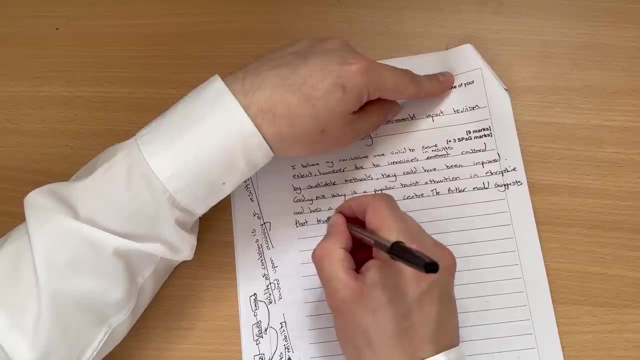 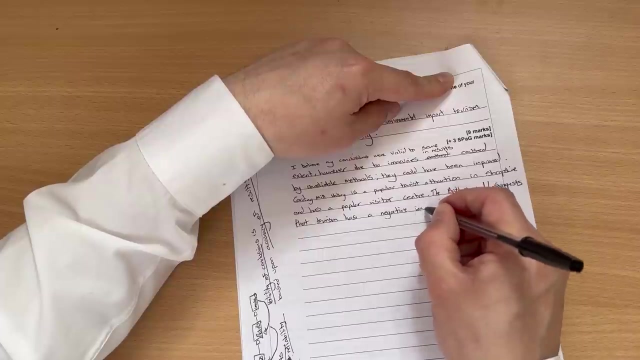 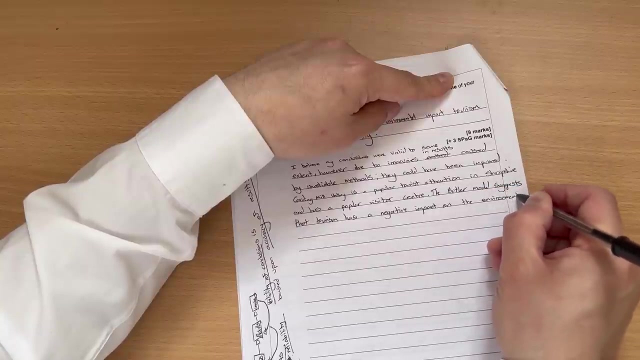 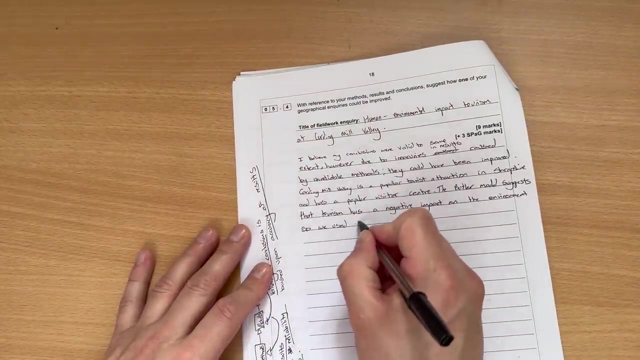 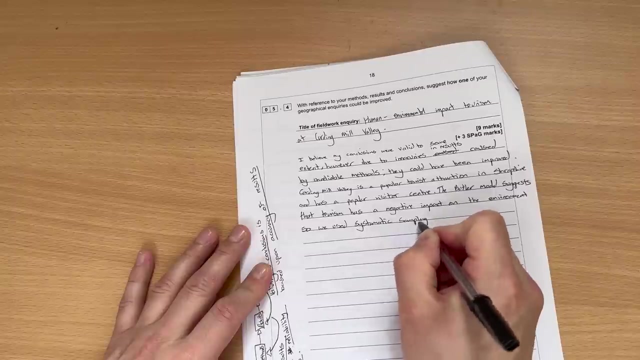 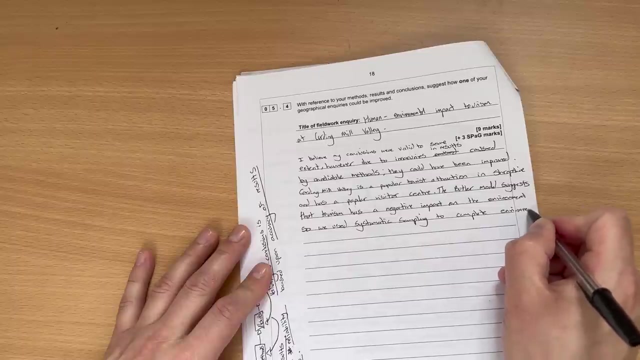 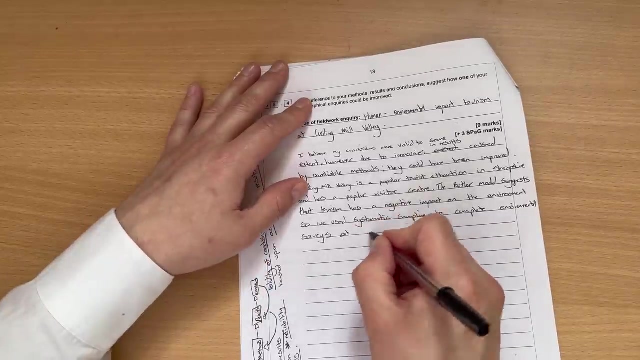 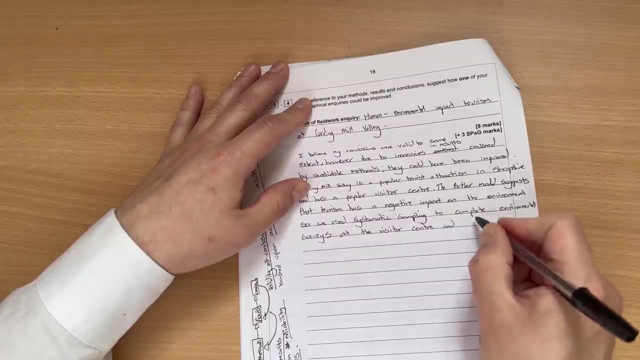 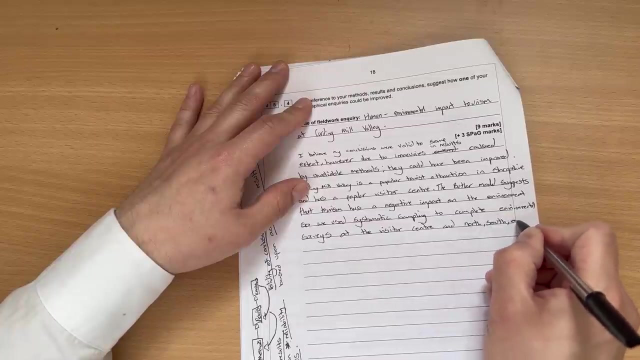 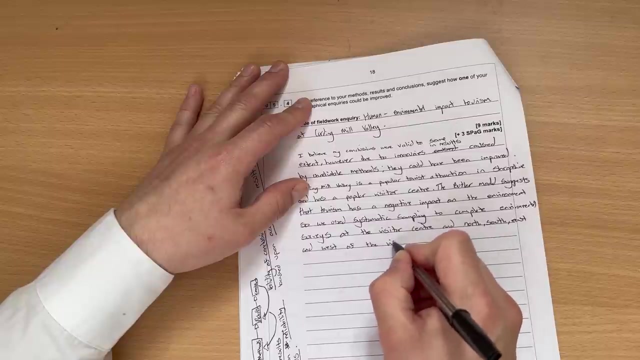 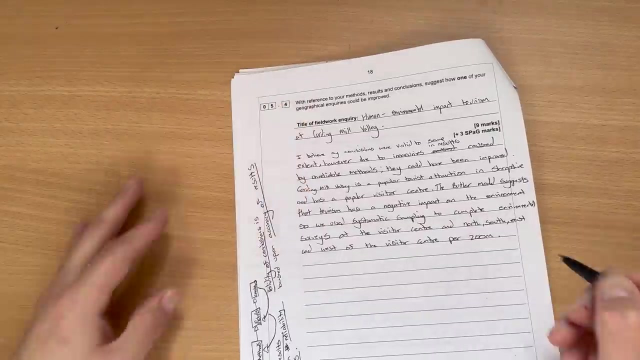 suggests that tourism has a negative, or potentially negative impact on the environment. so we used systematic sampling to complete environmental surveys at the visitor centre and north, south, east and west of the visitor centre per 200 metres. now that's a bit overkill, because we're setting the scene. 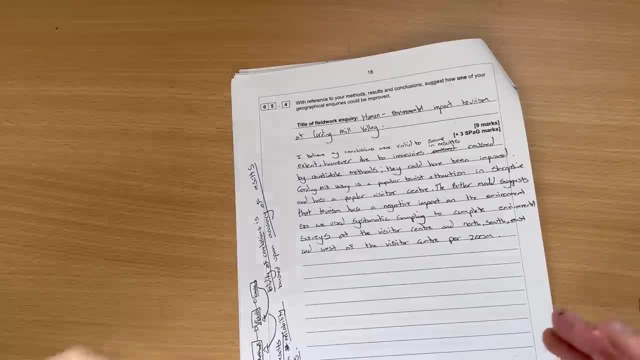 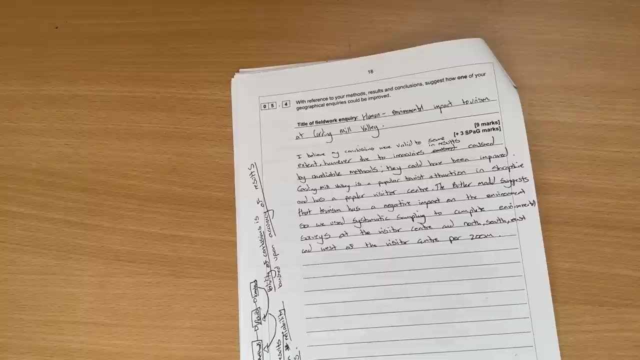 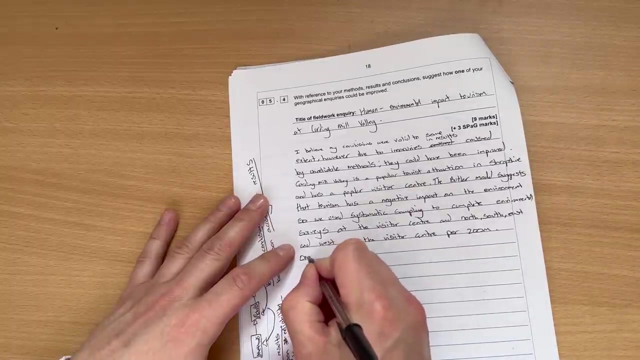 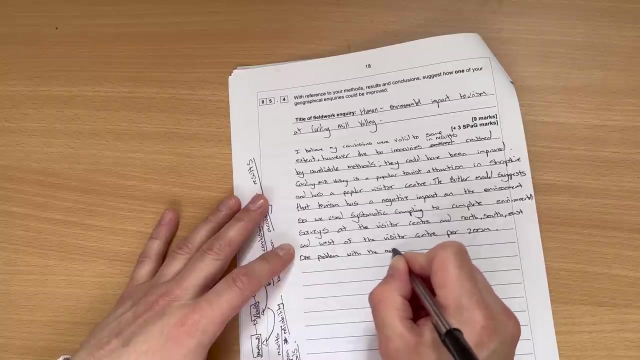 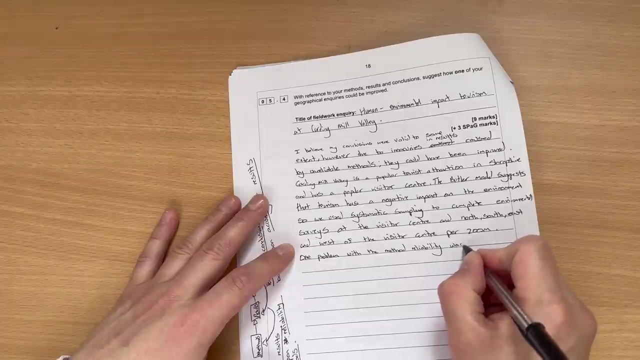 but we're setting it to a grade 9, I think so the examiner should. yeah, I get what's going on here now. what were the problems right? first of all, let's talk about the actual data: data collection. one problem with the method- reliability- was when we tried. 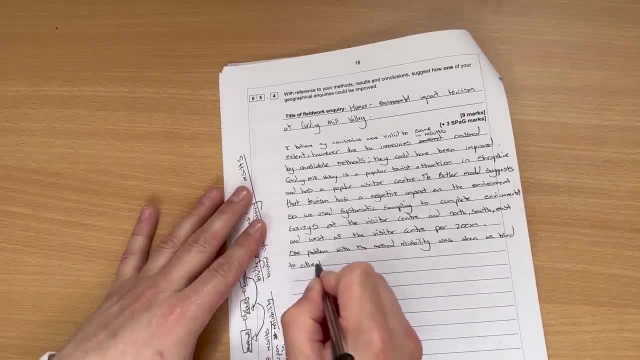 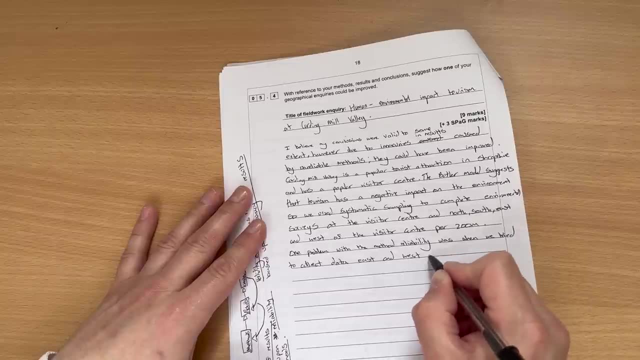 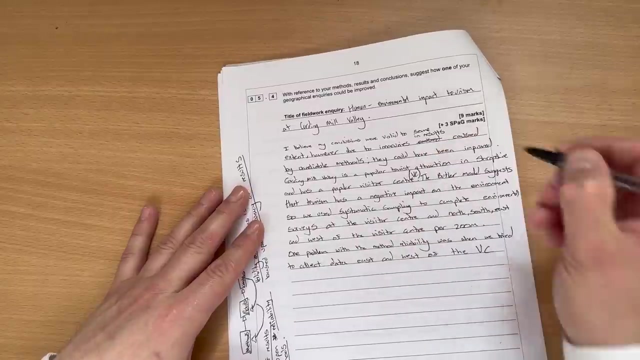 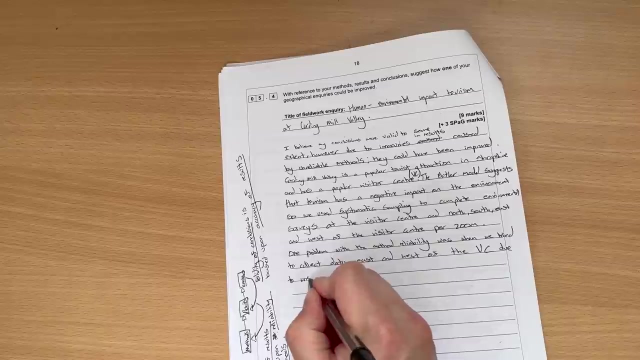 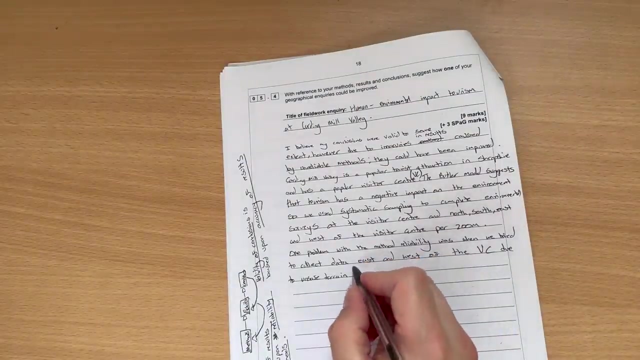 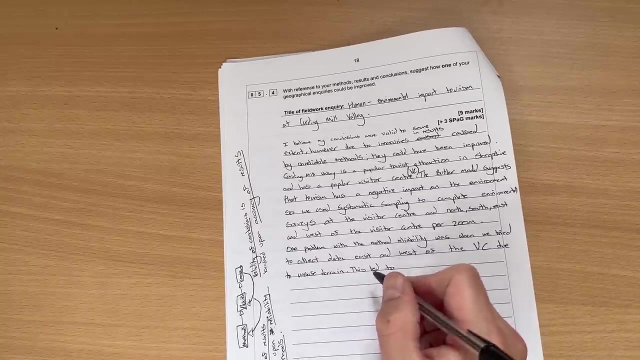 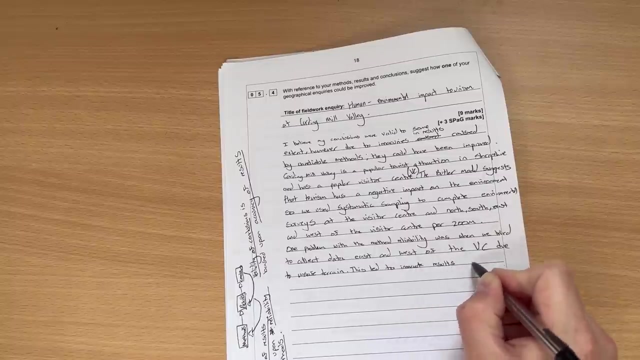 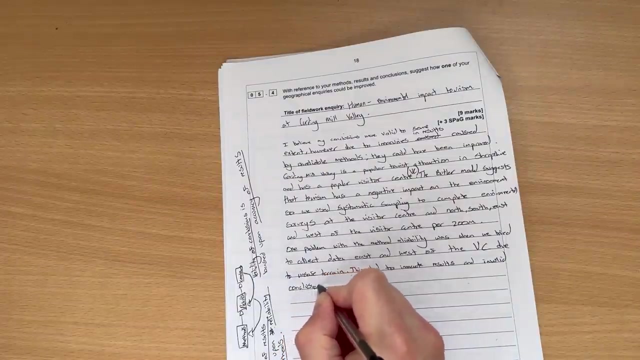 to collect data. to collect data, to collect data from a those. these led over the two Inaccurate Results and In valid conclusions. This is it. wants you to improve it? Okay, suggest that we could improve it. This is where you get in the marks. to be honest, to improve. 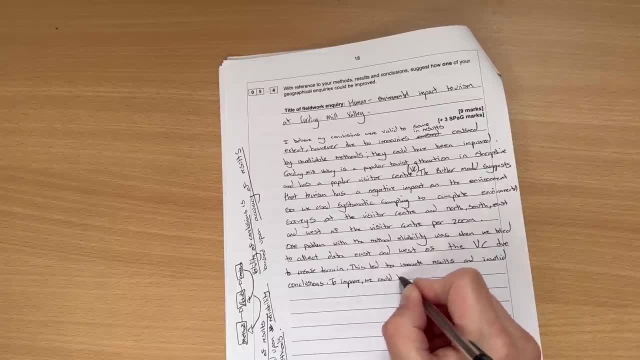 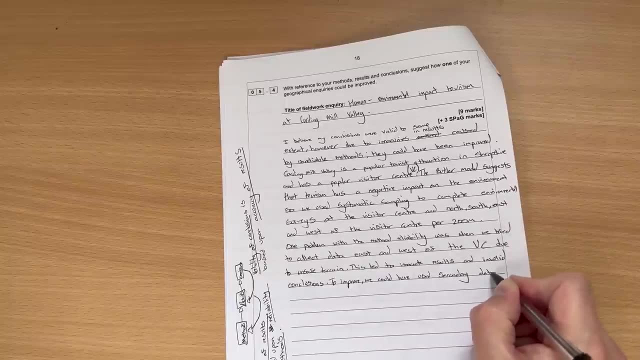 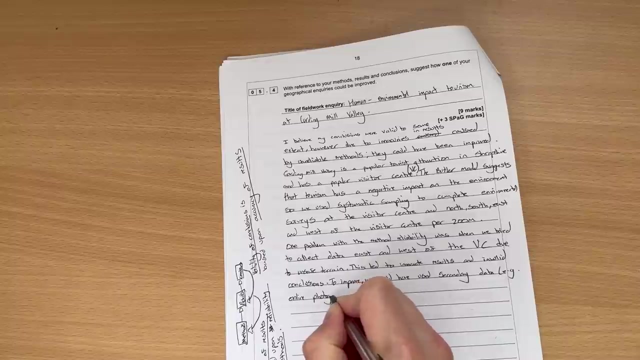 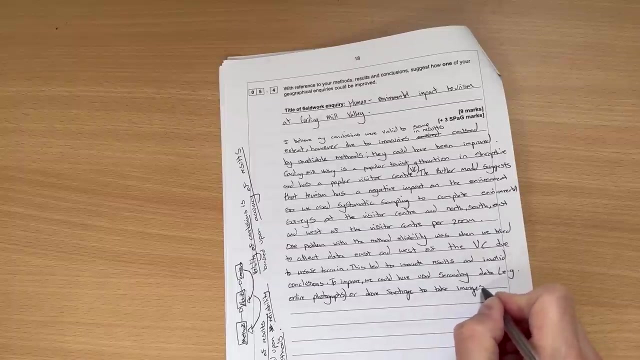 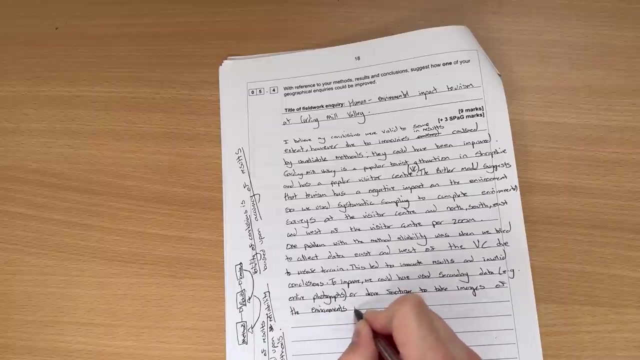 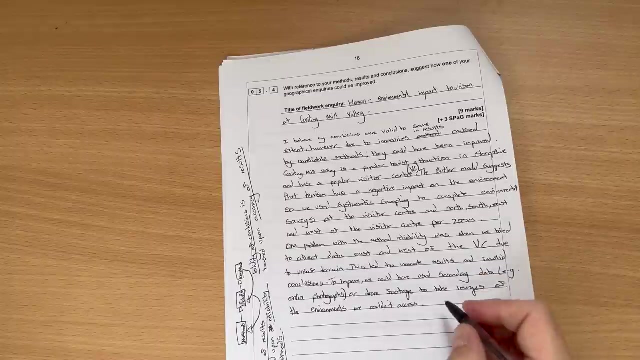 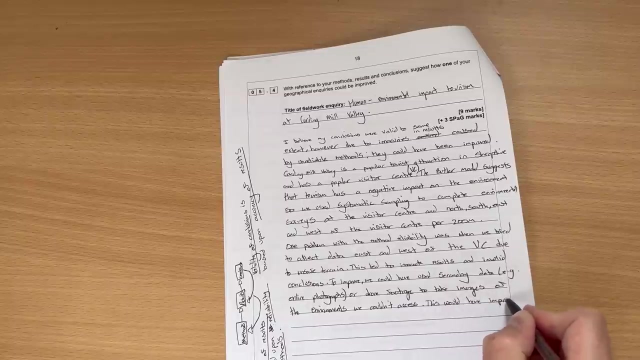 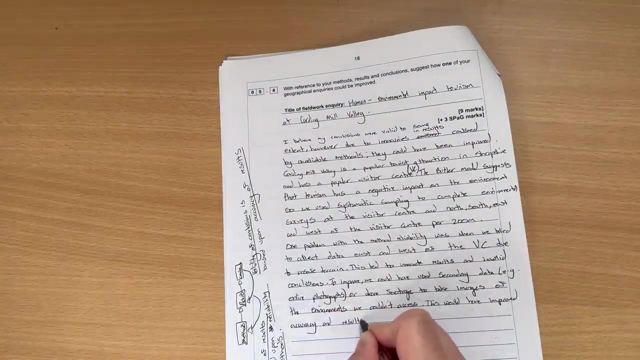 Comma. we could have Used Secondary data, EG online photographs, Or you know I love drones or drone footage- To take Images of, Of the environments We couldn't access. All right, let's bank the marks. this would have improved Accuracy of results And validity of. 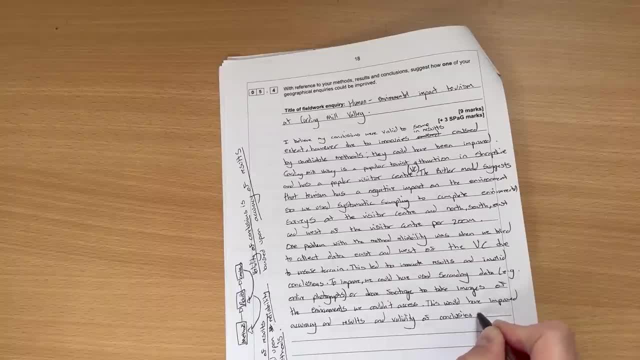 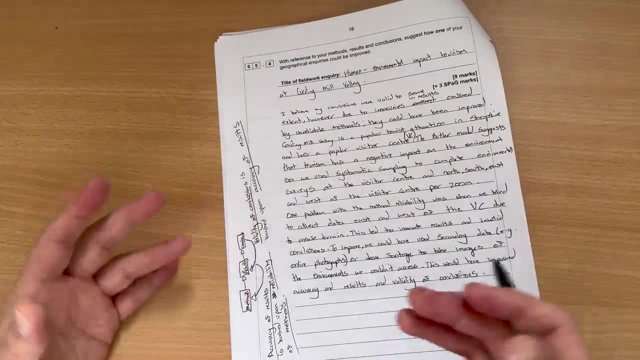 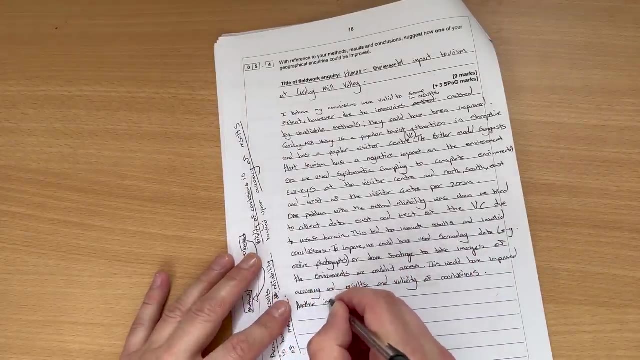 conclusions. So don't want the question. I saw we've got a long way around. it will remember. we want to properly set the scene. What else could we do? Well, subjectiveness. Oh, It was not to town, wasn't he? another issue Was the surveys we created. 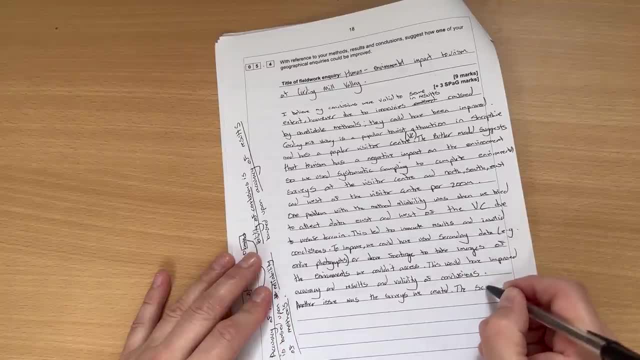 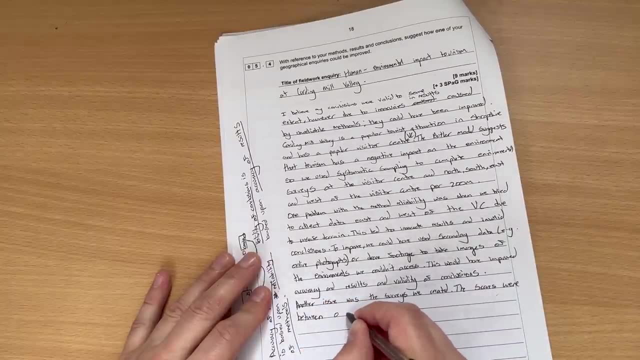 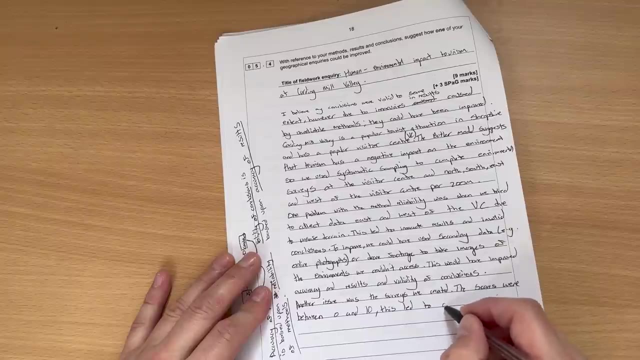 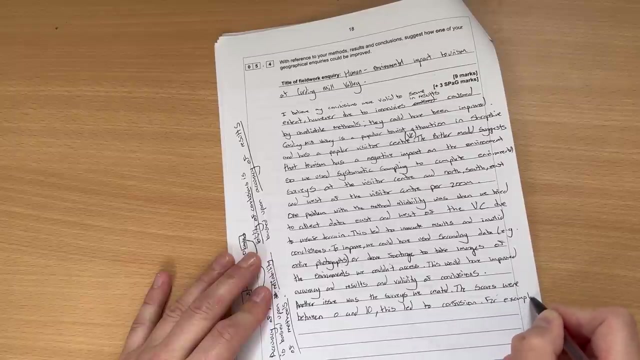 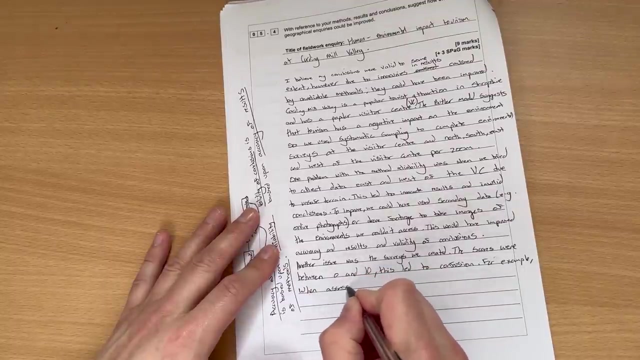 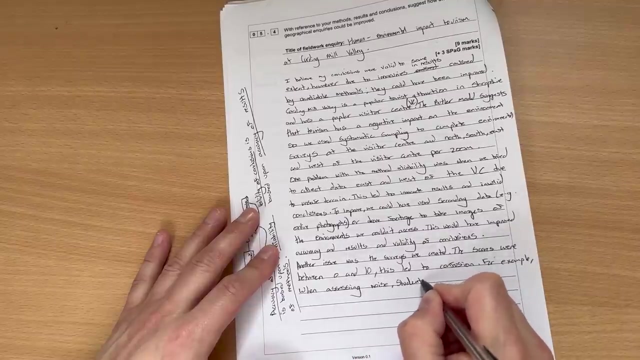 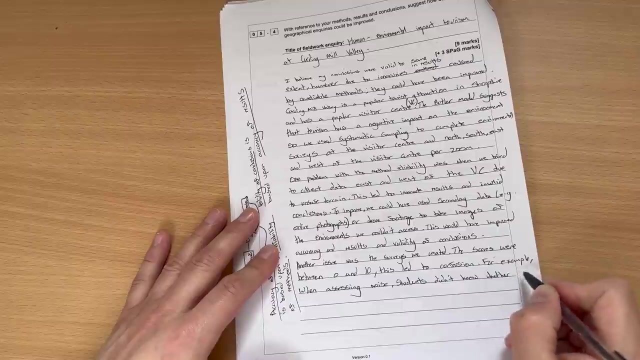 And The scores Were between 0 and 10. This led to confusion. This led to confusion- For example, Comma when Assessing. So that's what we're looking for: Assessing when assessing. That's what we did- is we assessed the environment. When assessing noise, students didn't know whether 10 was good or bad. 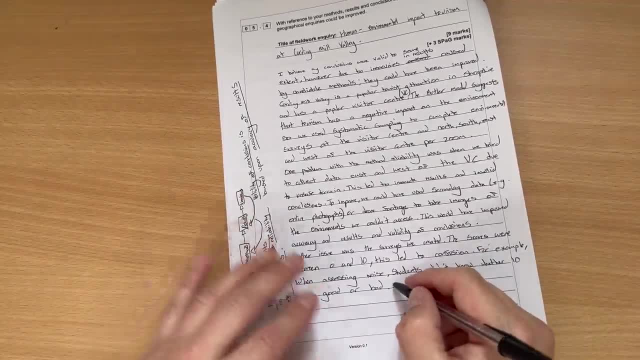 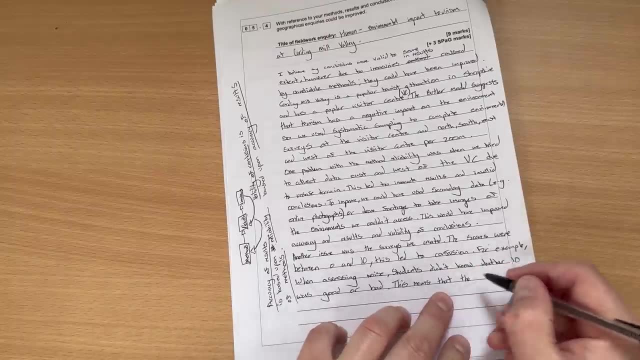 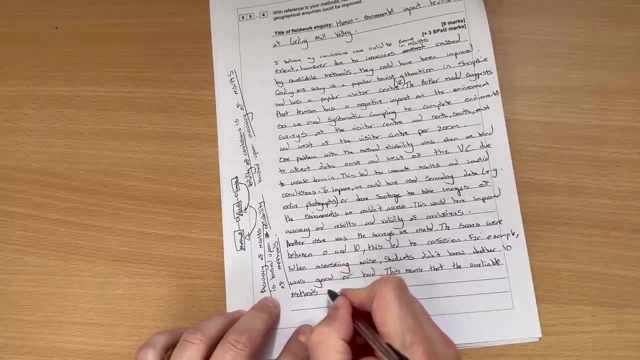 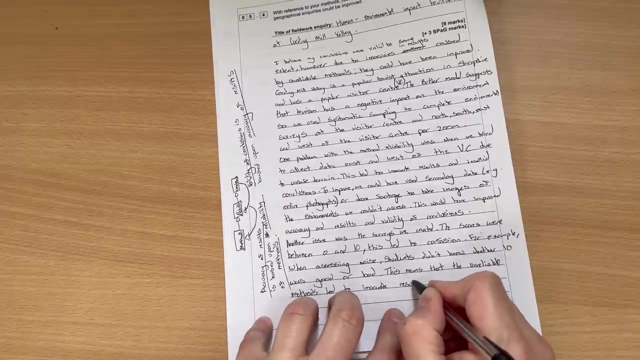 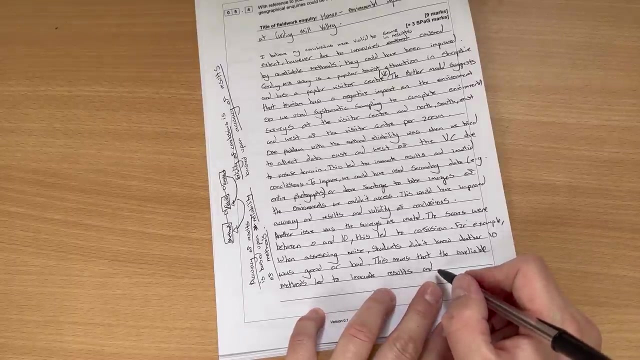 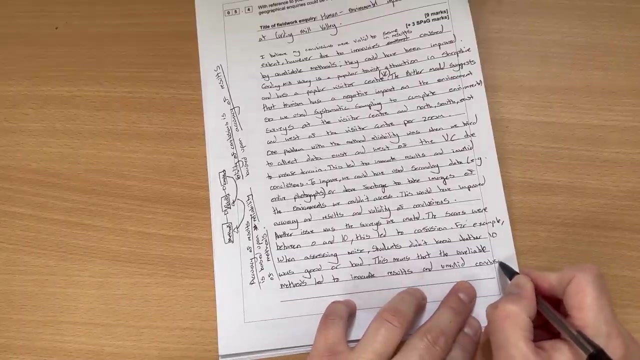 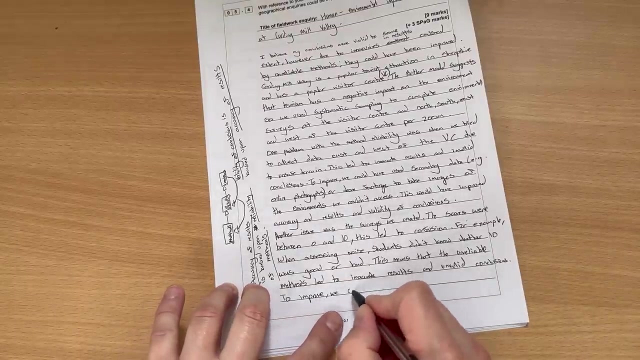 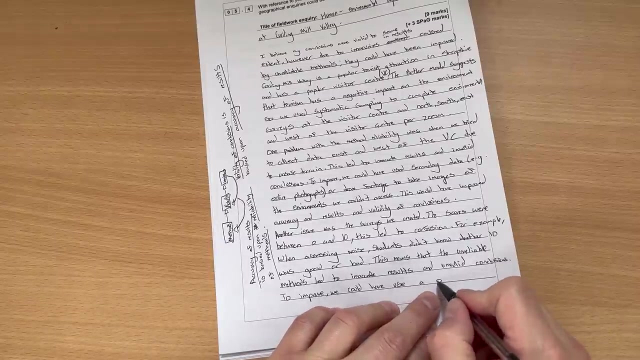 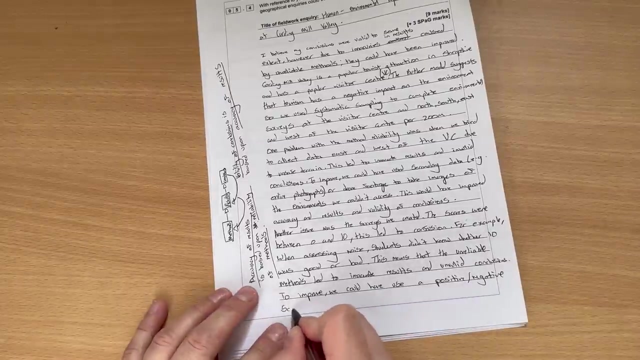 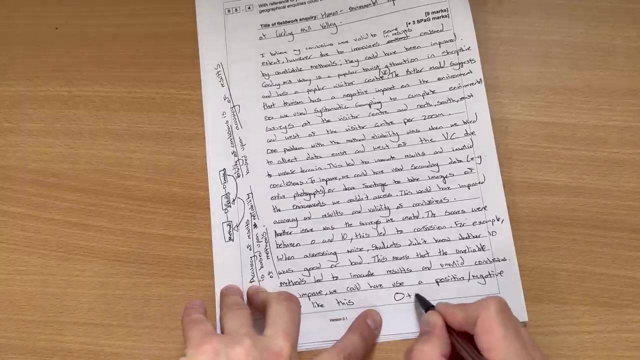 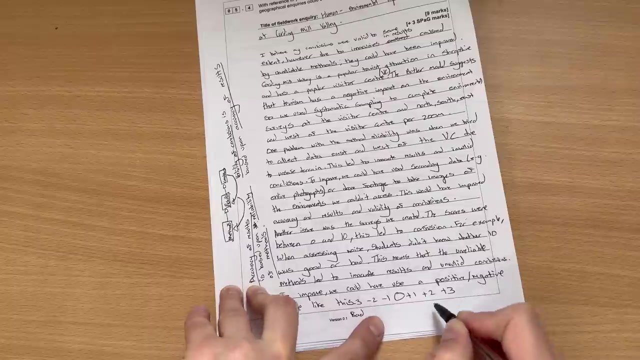 And this means that the unreliable methods led to inaccurate results And Unvalid conclusions. now this is where I'm getting the marks To improve comma. we could have used a positive negative scale, sometimes called the bipolar chart, like this and Drury: zero plus one plus two plus three minus one minus two minus three- bad. 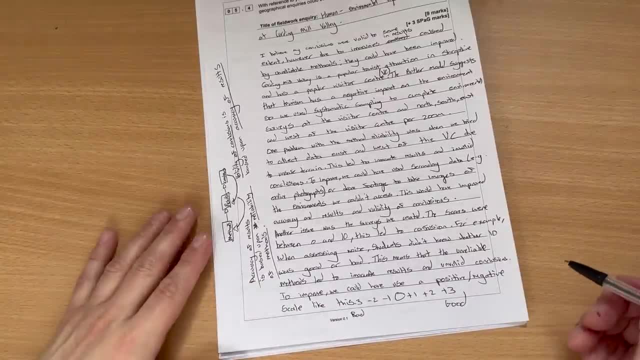 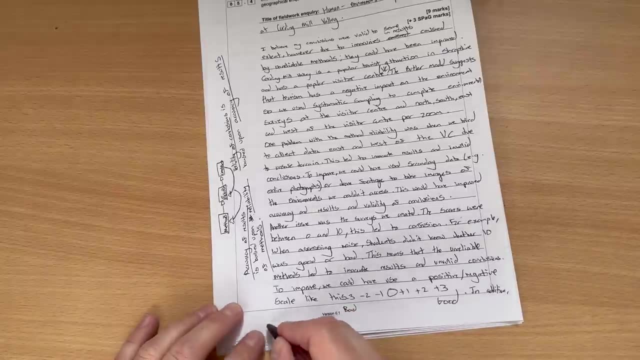 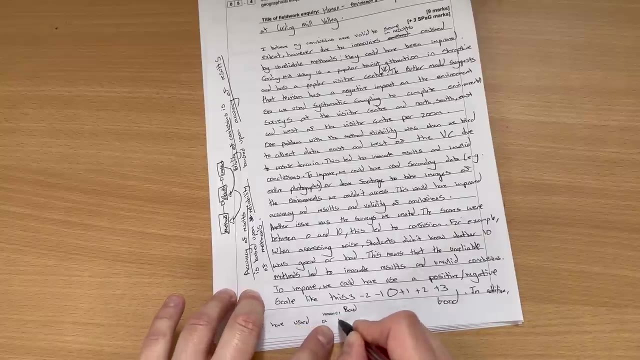 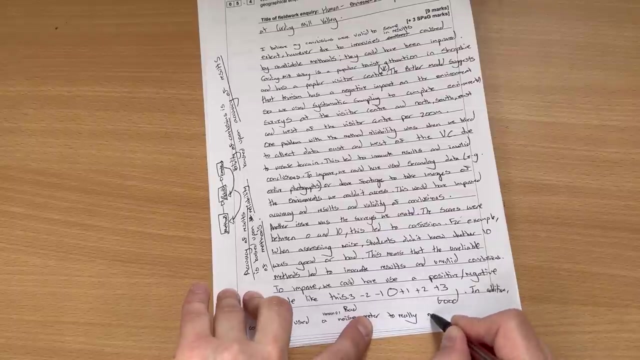 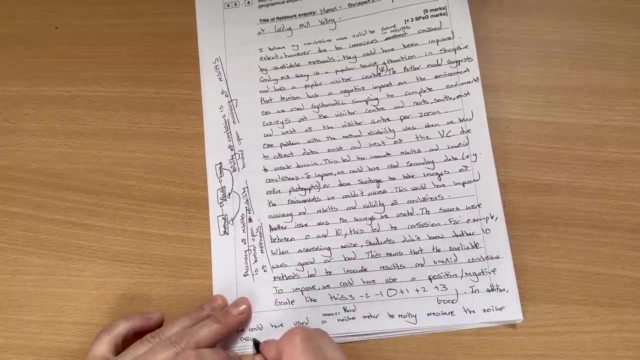 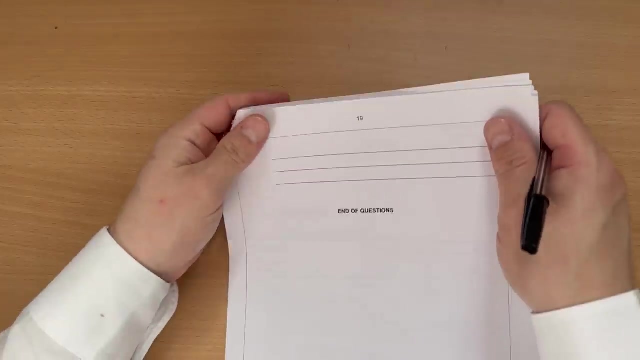 Good, Now again away from what that's showing. In addition, We could have Used A noise meter- some of that measures noise- to really measure the noise accurately. All right, a little bit more space finally, comma. 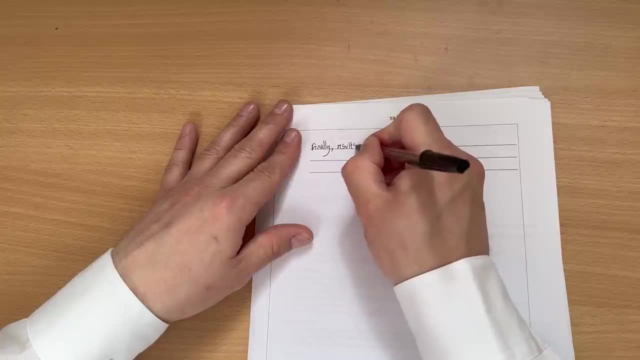 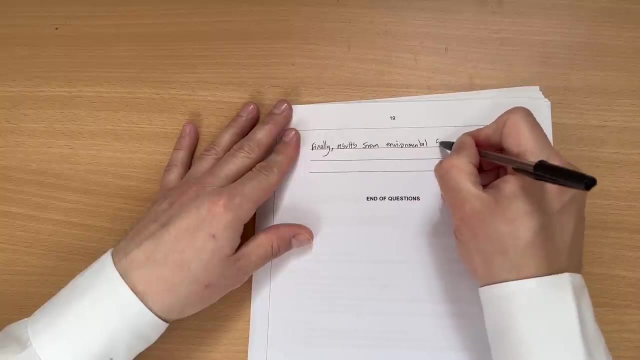 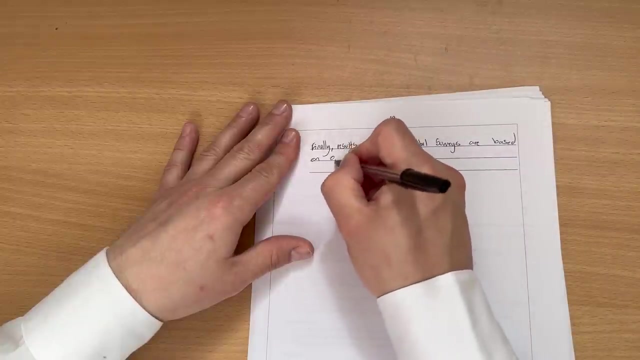 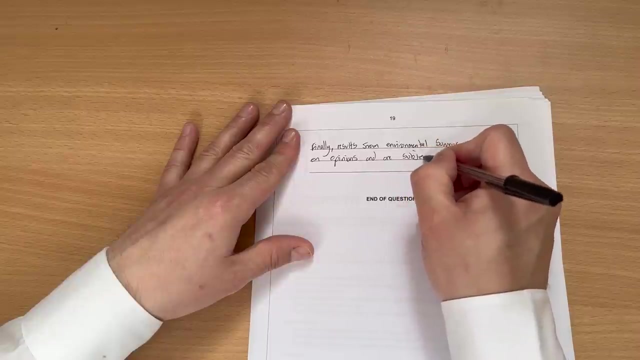 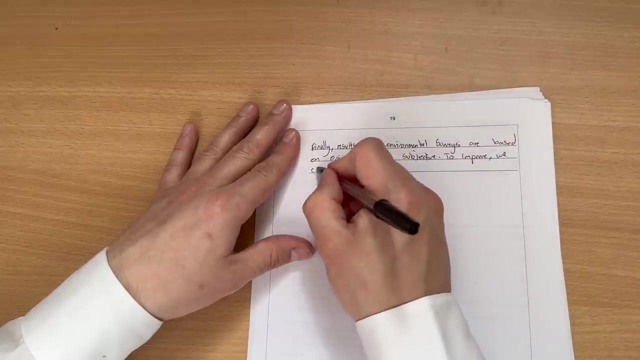 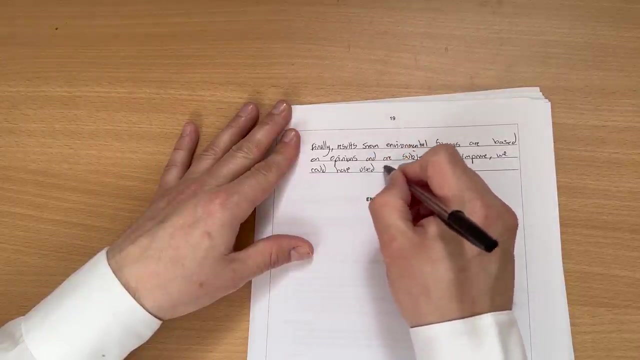 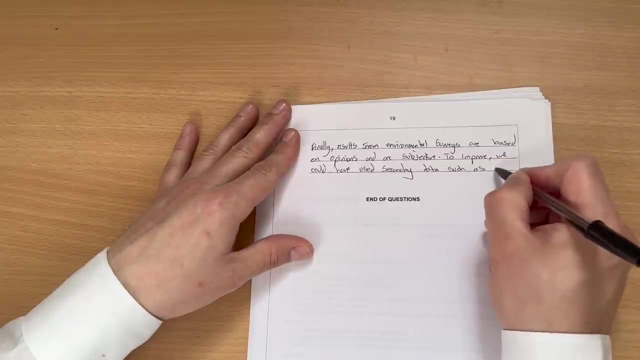 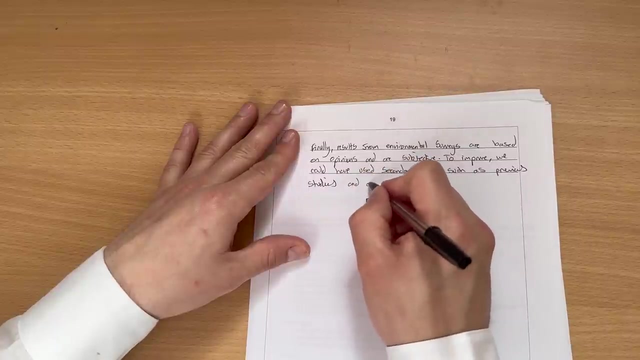 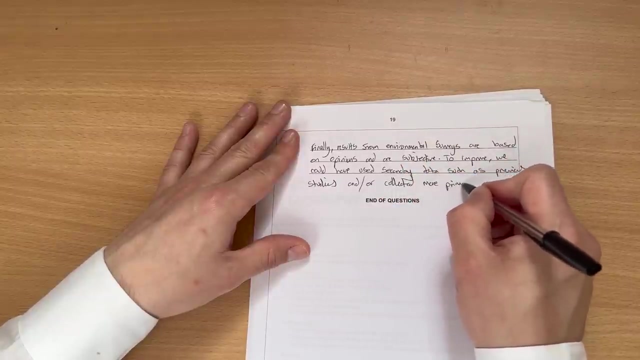 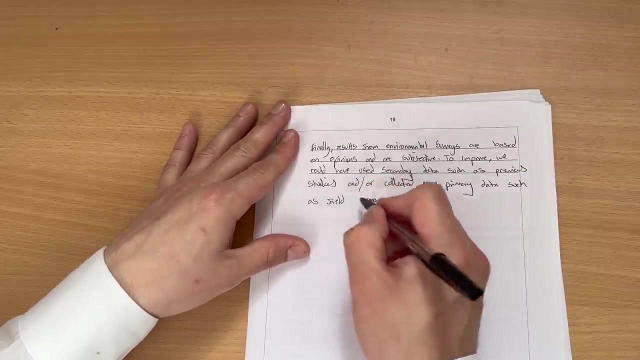 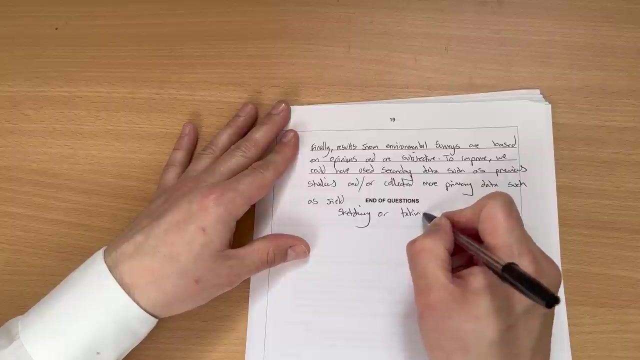 Results From Environmental surveys Are based On opinions And are subjective. To improve, We could have A negative scale Of used secondary data, such as previous studies, and or collected more primary data, such as field sketching or taking photographs. now remember that if I'm going to say this once, 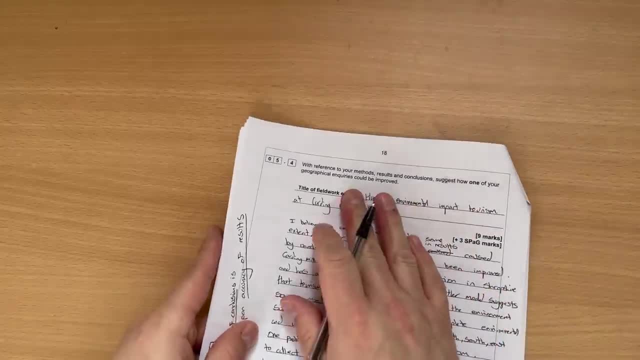 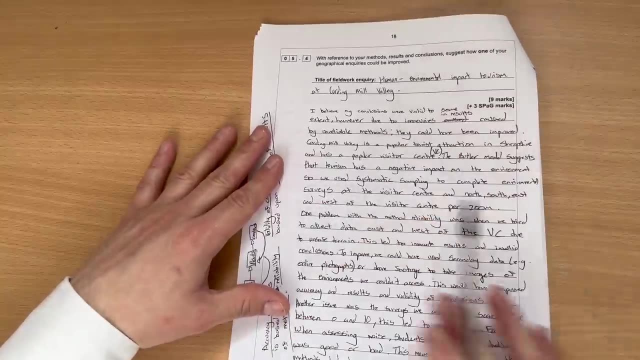 I say ten times the key thing about this question: you do what it tells you to do. you could have got these two men to mark writing less than this by just doing this. remember, I'm setting the scene, I'm trying to help you revise at the same time, but what it wants to say is: how could you? 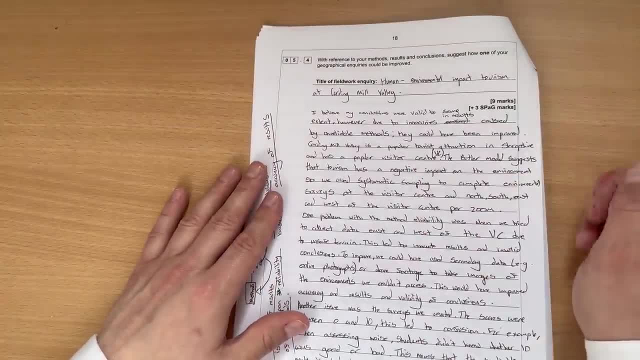 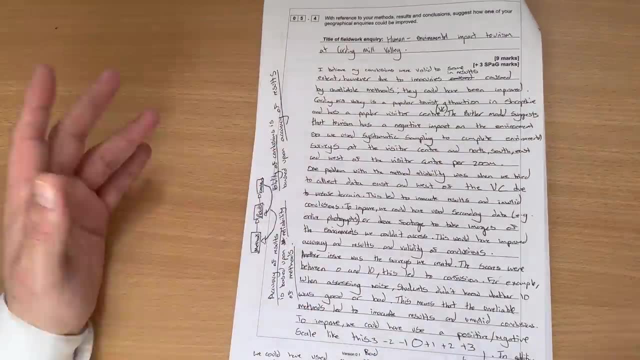 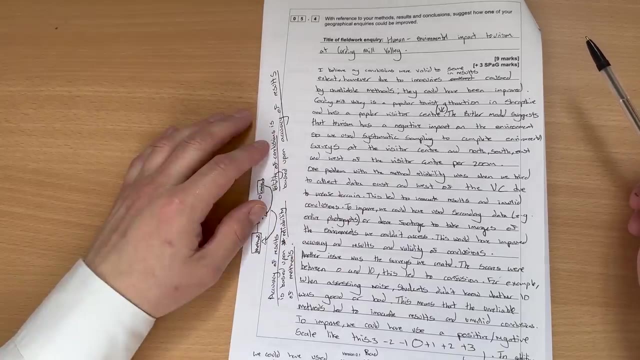 improve these. you could say the surveys were not very good. we didn't understand the scales. to improve this, we could have used a bipolar scale that looks like that. all right, you could have said the results were subjective. this means that was based on opinion. to improve the results, we 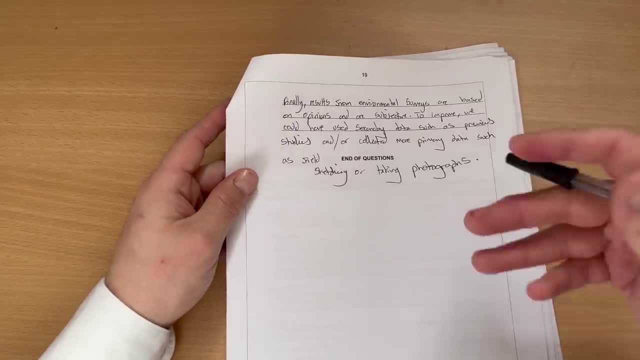 could have taken photographs and we could have assessed them back in the classroom. all right, so there you go, respect.